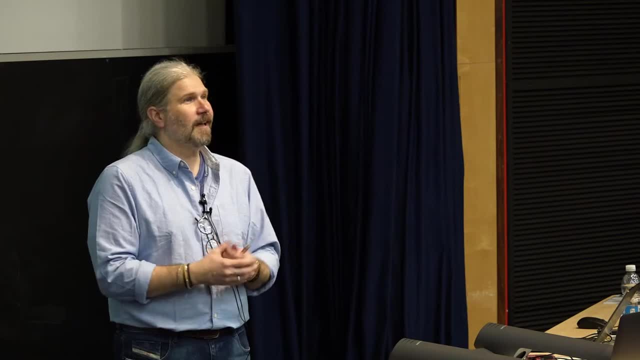 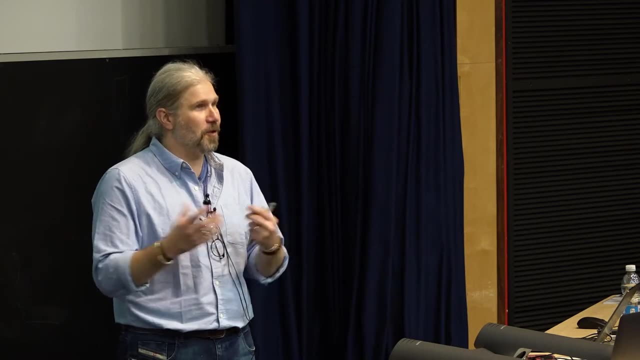 sandpit to understand how we can develop new technologies. And even today, Barbara's beautiful talk is actually a lot of underlying quantum optics tools in the process. All the operations we do on qubits, two-qubit gates, all of that is developed from what we've done with quantum 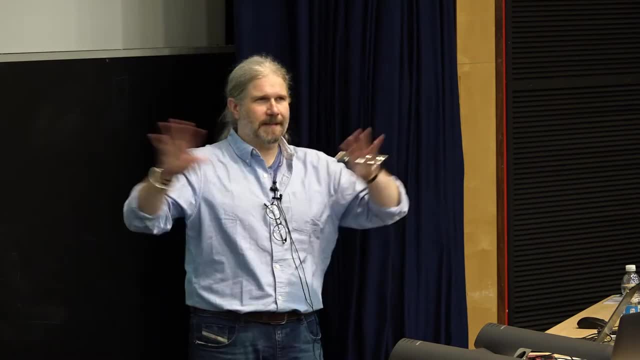 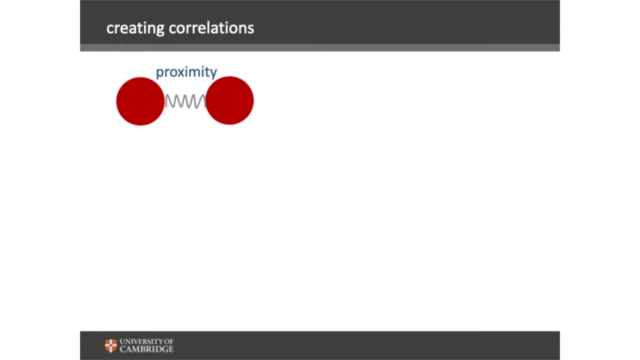 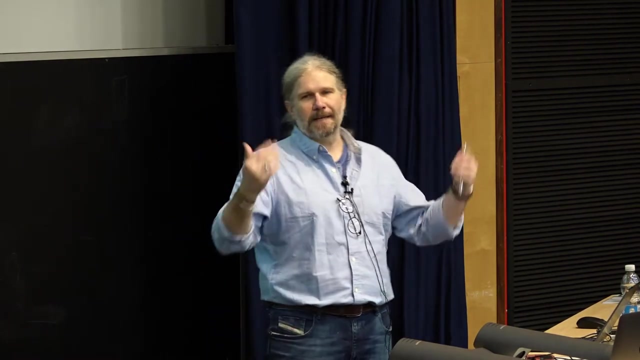 optics, But I'll extend this to as much as I can on what the impact is. So let me start with actually a very simple question, and hopefully this will highlight why this has all been so exciting to go in the realm of various applications, including. 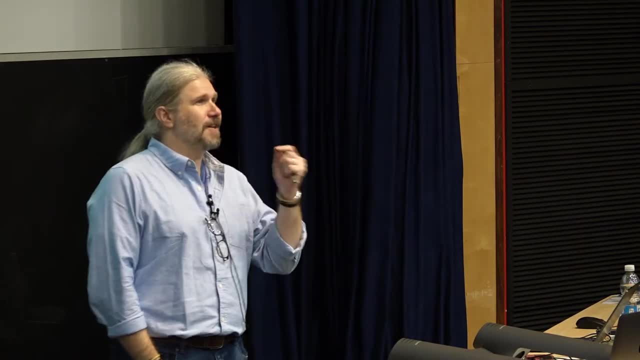 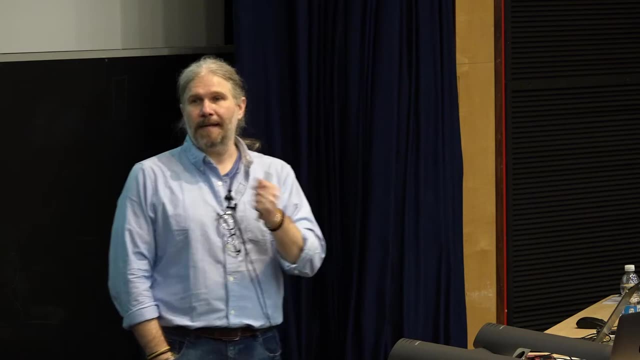 quantum networks. So let's start with the concept of creating correlations. If I need to, If I need to identify matter, I would say it is formed by putting many, many, many things together, like atoms. But just because they happen to be around each other is not enough. 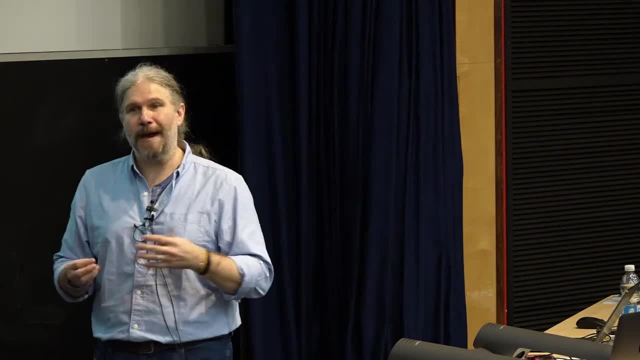 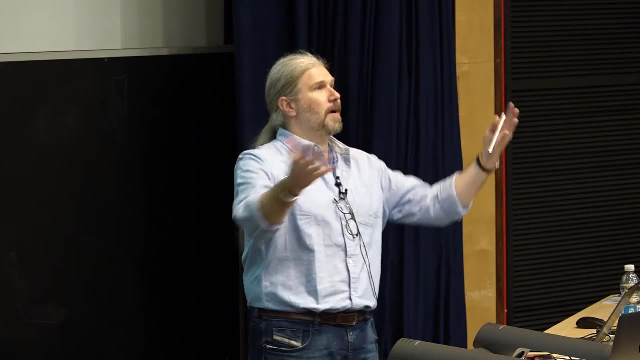 to form a solid or a liquid or a gas right. The phase of matter arises only because you have interaction. Interaction leads to correlated states and that correlated state combined leads to a collective phase. and now we have a matter, a large-scale matter. So it all. 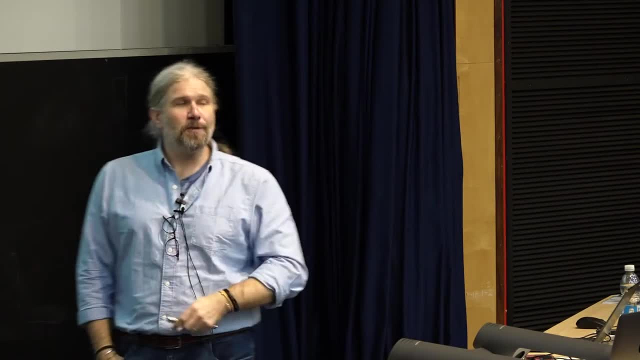 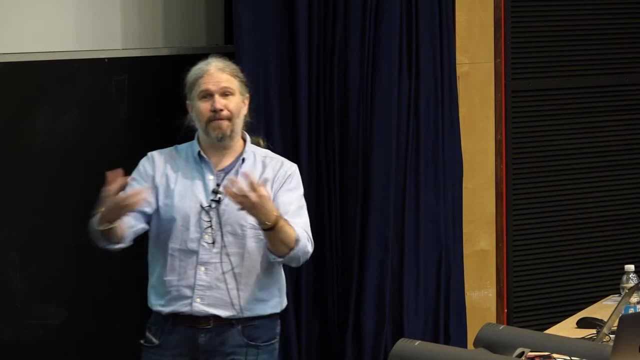 starts with this. Let me see if this works. It all starts with this: You take two objects, you bring them together and you let them interact. If they're interacting attractively, they might form a bound state together. right, That's the formation of a molecule. But the 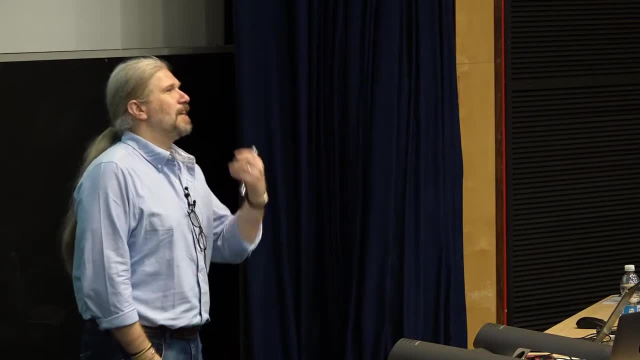 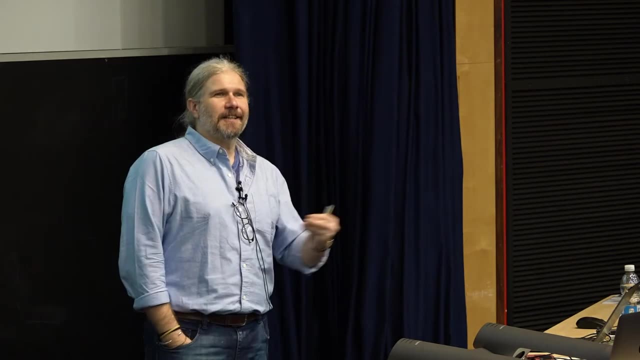 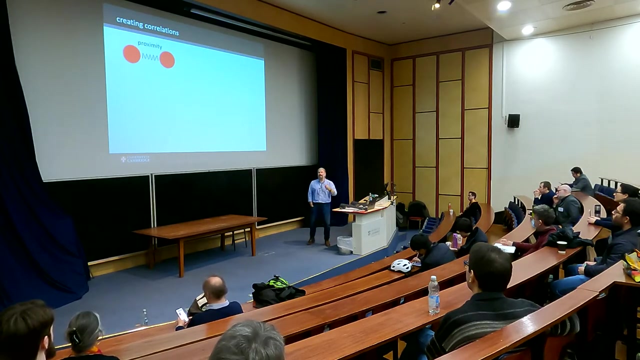 whole point, then, is the word proximity. I think it's an underappreciated technical term in science. Proximity means there is a length scale, characteristic length scale, required so that you can induce interactions, to have the right strength of interactions, so that 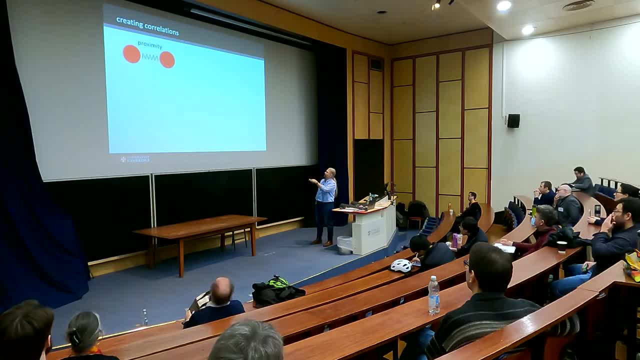 that system now cannot be treated as This red blob. I'm a physicist, so red blobs are perfectly fine for me as physical objects- This red blob and that red blob, but rather a two red blob object like a molecule right. 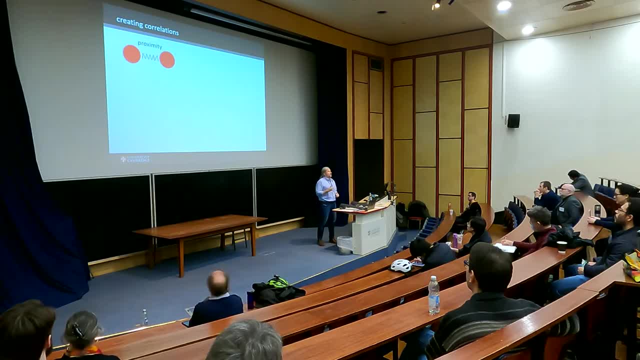 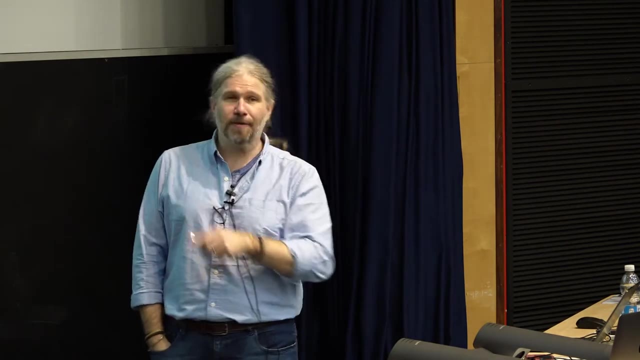 So, for whatever your interaction of choice is- electricity, magnetism, anything else- there is a characteristic length scale that defines what this word means to you: Proximity. Every matter that you know relies on this and has a corresponding weight: The word proximity. There is one and only one example I can find, and please help me. 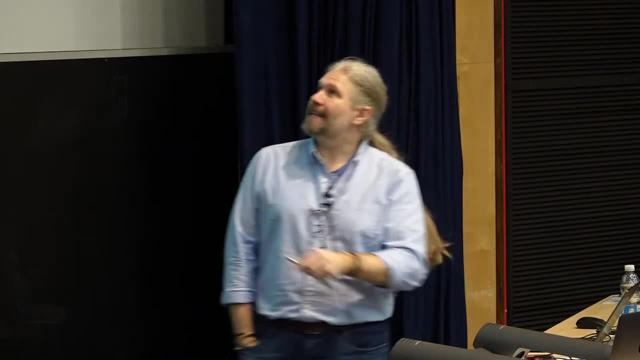 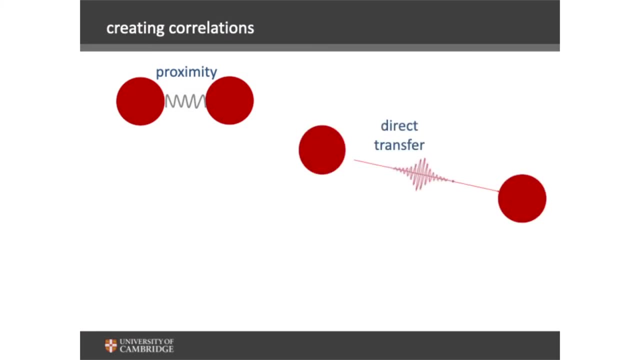 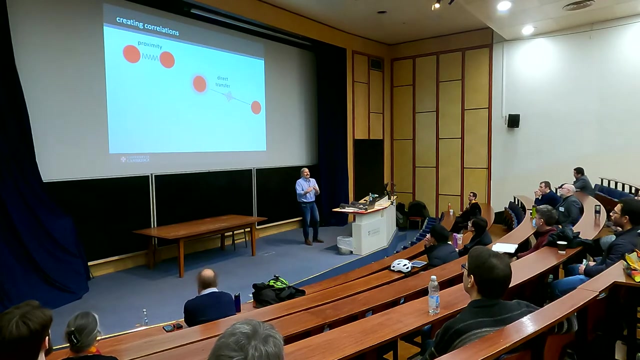 if you have other examples, but there is one and only example I can find where I can beat the concept of proximity and still create a correlated state, a single entity, And that is if this red ball has a red hue or a pink hue around it, what does that mean? It means 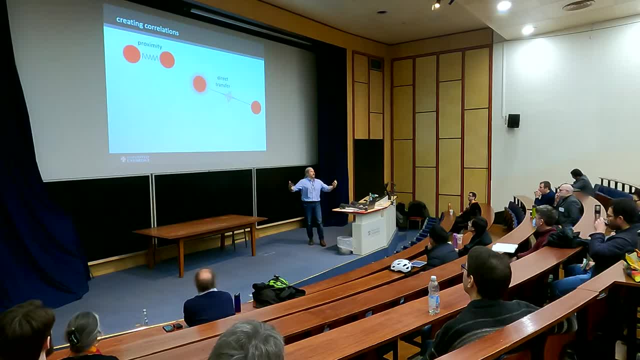 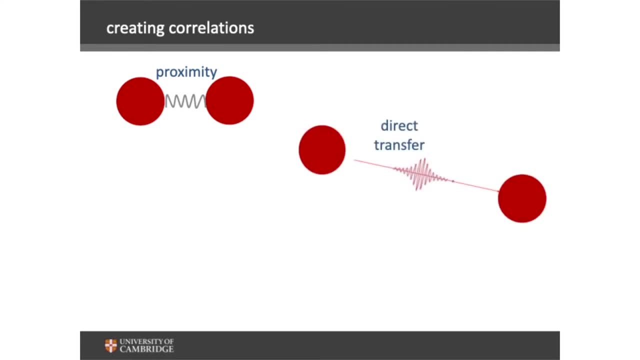 this red blob can couple to light some electromagnetic radiation, And if that radiation can be exchanged with another red blob, I no longer care about proximity, physical distance between the two red blobs. What I care about now is what is the efficiency of taking this energy, this 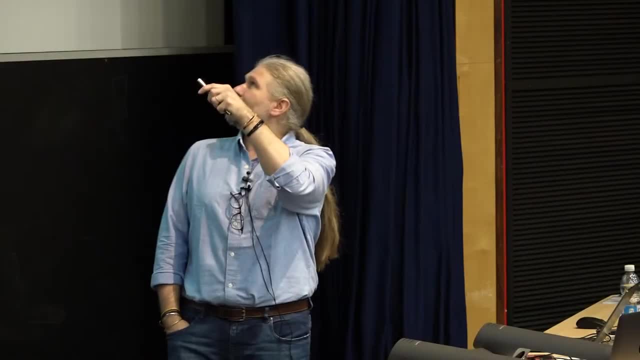 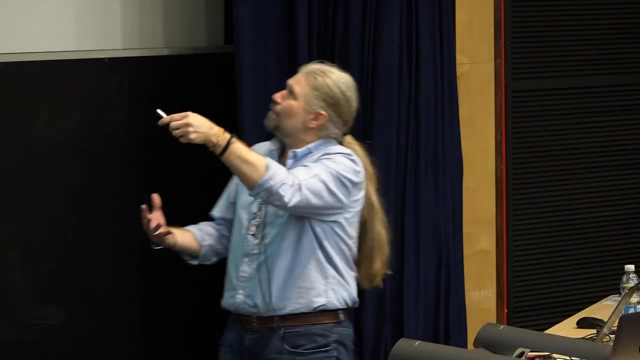 energy exchange between the two, from this one to that one, with sufficiently strong, let's say, interaction. So you wouldn't think of the actual physical distance between these two objects, but you would think of- let me draw a virtual curved mirror here and a curved 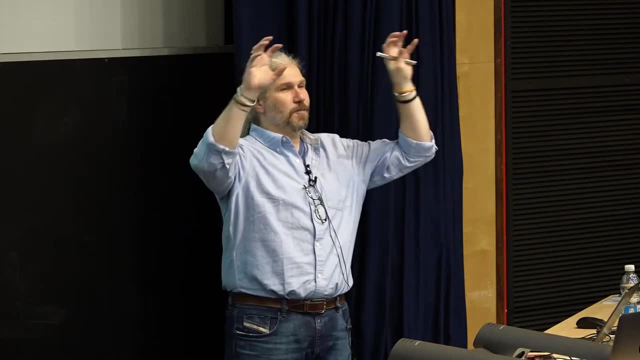 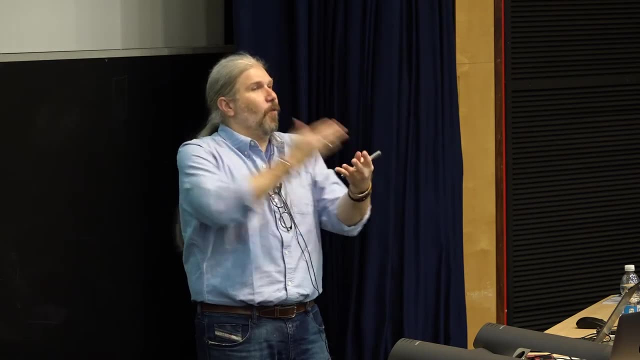 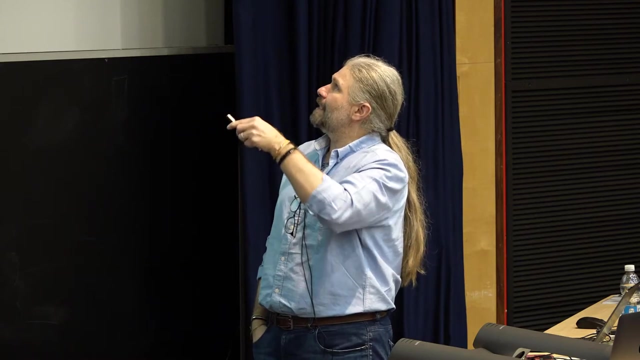 mirror. here You can think of a big cavity, optical cavity, and you put two red blobs where the red blobs are at the antinodes of the cavity mode. So then you're interacting through this one common, well-defined optical field trapped inside this cavity. So then I don't care how far 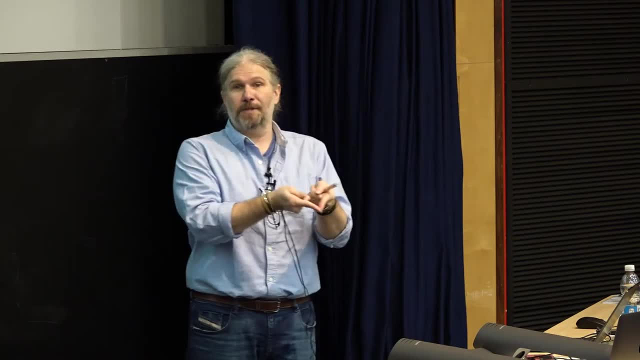 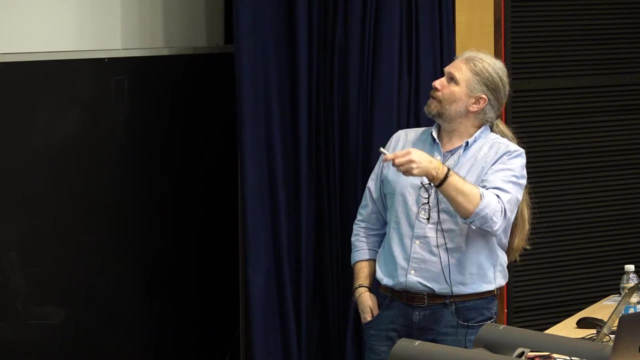 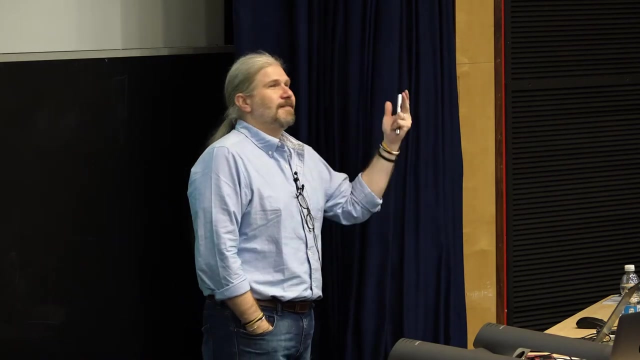 these are as long as they're both individually talking to a common object, which is now the radiation mode. If I have that, I can create strong interactions between these two objects through exchange of radiation energy. So that's the only example I can find. Help me if you happen to know another one Now. 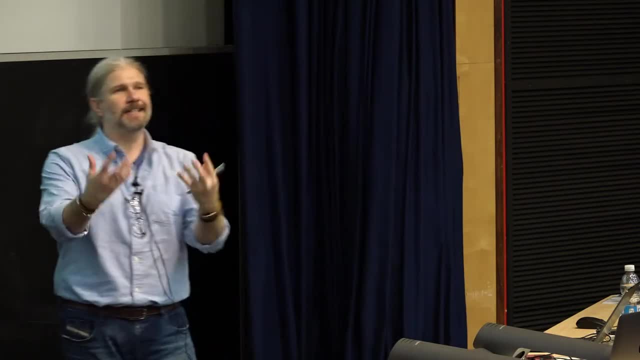 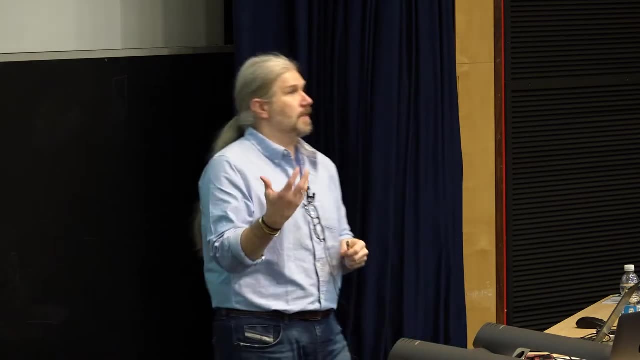 that's a material property. That's how I will justify matter-light interaction, the heart of quantum optics. That is just one example of why it's worth studying, why it's interesting to go in that direction, to create correlated systems that do not obey our notion of proximity. 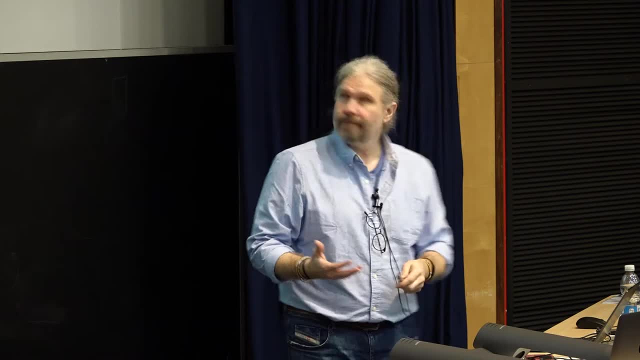 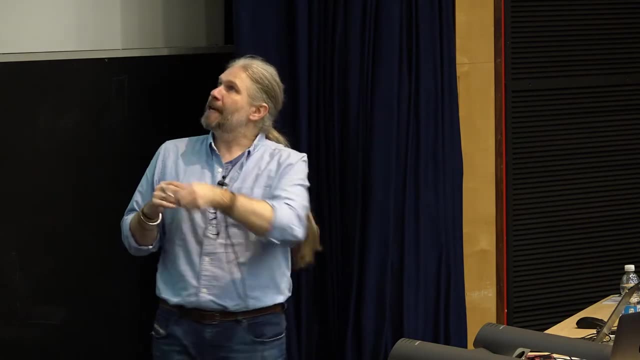 requirement or how things are laid out in physical space. You can imagine not two, but two million of these things If I have these one-to-one couplings of two million instead of creating two million of these ones based on lining them up one by one to create a lattice. 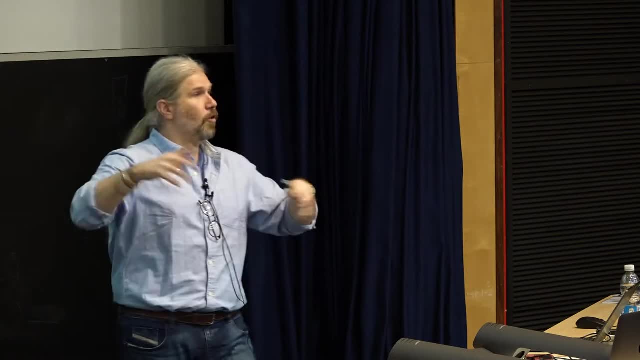 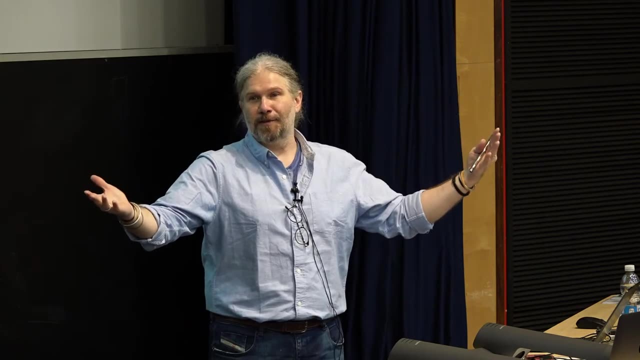 I'm now talking about arbitrarily located atoms, all linked strongly, creating the effect of the phase of a solid, for example, without looking anything like the ordered solid that I know. As long as I keep track of each one, I'm building up a topology that is independent. 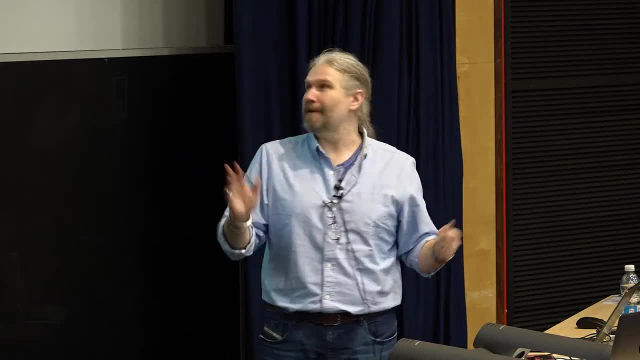 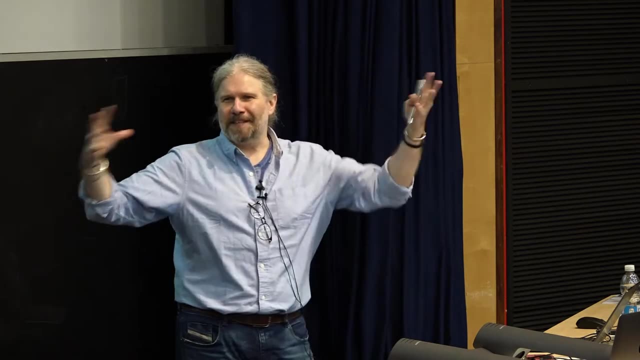 of real space, essentially. So. that's attractive for its own merit, But that's busy, right. I have to have- if it's two million of these, I have to have one million cavities, optical cavities to identify modes, and all that. There is something. 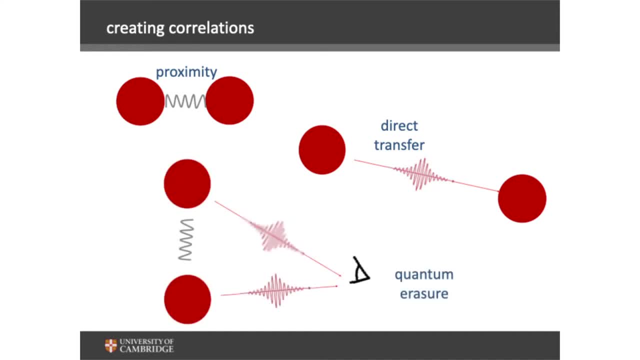 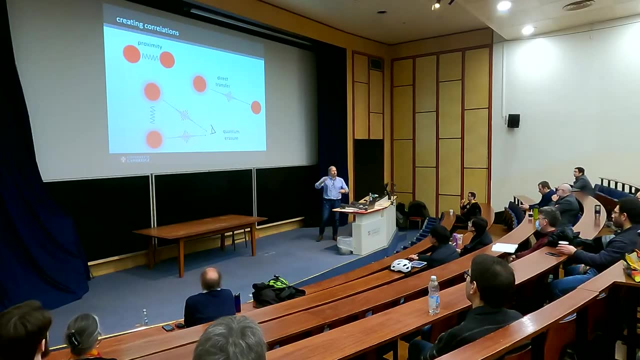 else quantum physics can give us, and it's the concept of never even interacting in the first place. right, The concept of quantum erasure, where you make a measurement to not find out about the answer, but in the process you make sure that no one else finds out about. 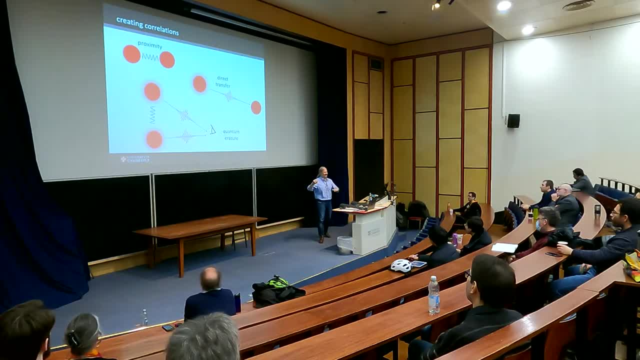 the answer either Okay, that's as colloquial as it can be, As long as I can make it. You want to erase the information in such a way that you create the ambiguity in colloquial terms, or a superposition state in more technical terms. Now, how does? 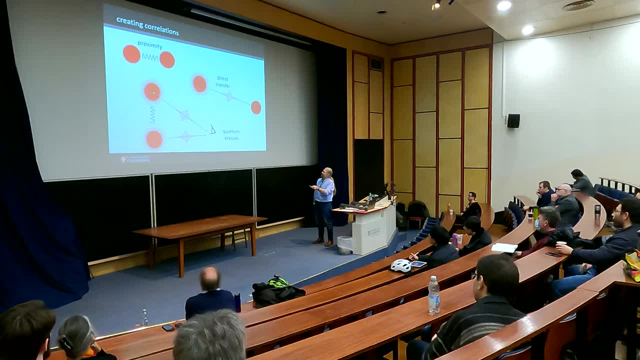 that work, You have your two red balls with the pink hue again. The pink hue allows them to couple two well-defined modes, optical modes. But then there's a third party, a third party that looks at the photons or even, in some cases, the probability of photons coming. 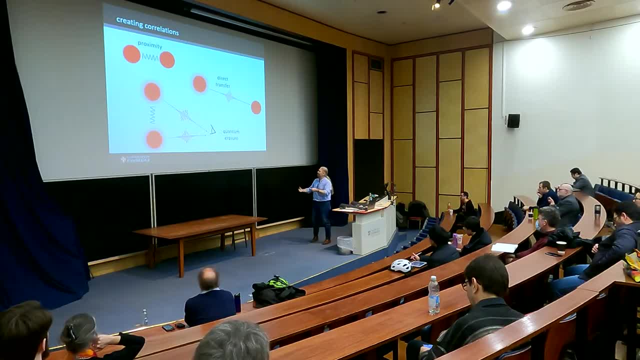 It's not even real light, but the probability of the light might come this way, And as long as this eye over here cannot tell the difference between these clearly distinguishable arrows, but let's say that it does a special trick over here and completely. 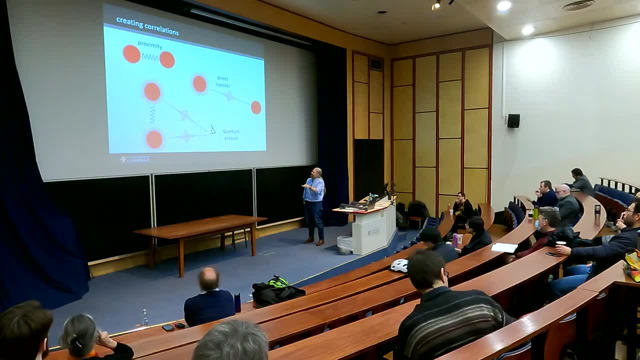 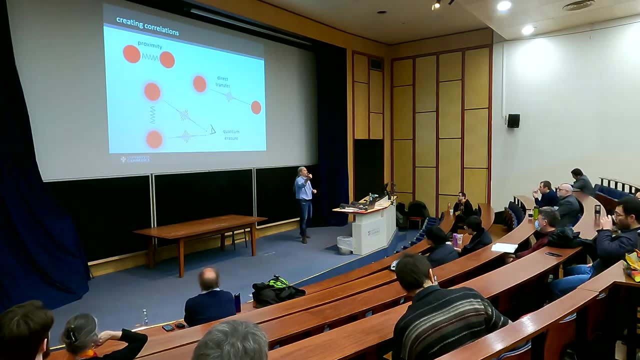 confuses that information, then you can end up creating, if you're lucky, if you do it the right way, you can end up creating correlations between these two red blobs without the need for each of them being particularly positioned anywhere And, of course, again, no link to. 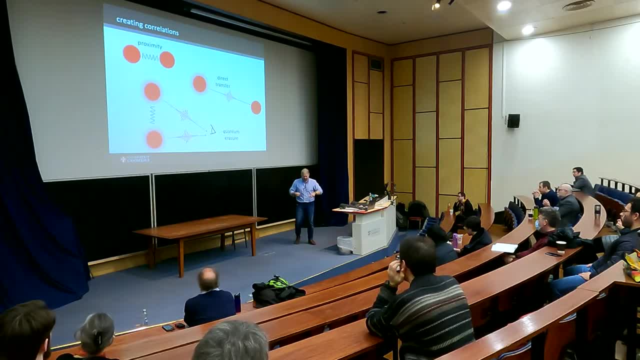 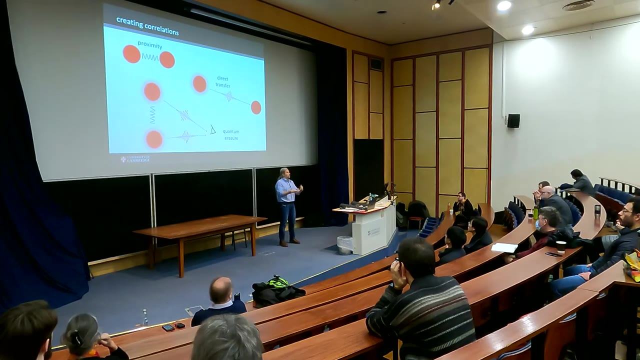 their proximity. So imagine this eye over here like a puppet master with all the strings attached- strings being light strings- to create pairwise correlations on a large ensemble of, let's say, two million of these guys. And again the same concept that we talked about over here of two million atoms with an emergent. 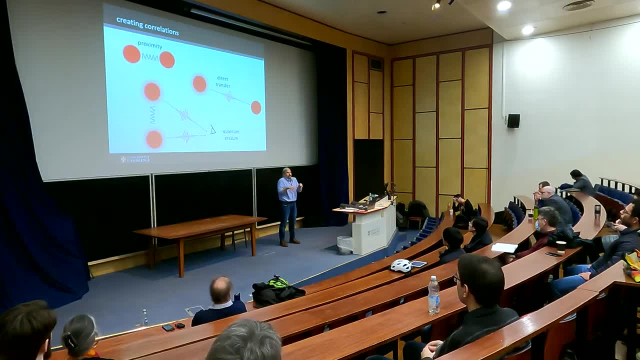 correlation, at the end of it with a certain solid phase. I can do this by literally being one control unit, controlling all of the atoms, dialing them up pairwise through pairwise interactions, entanglement or correlations, And then I create this new phase of matter. 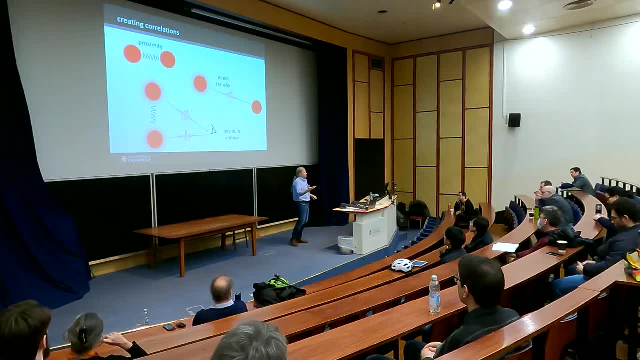 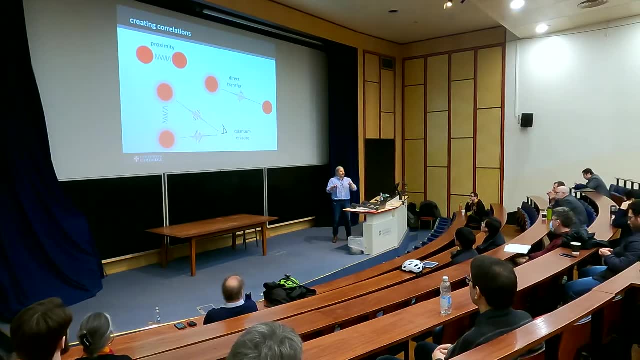 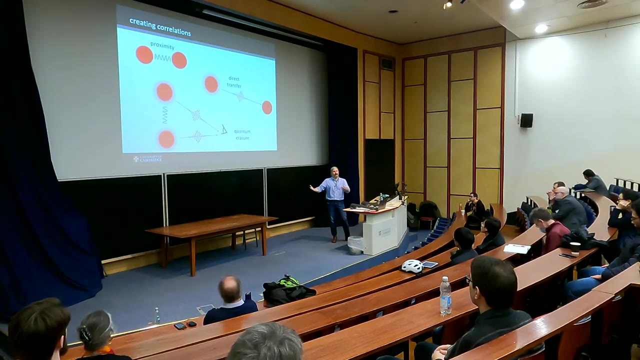 that isn't linked to where they are, but rather to the topology, the index map. That's attractive to be able to create matter at will or engineer synthesized matter at will by programming rather than bringing things together. When we synthesize matter now, we're 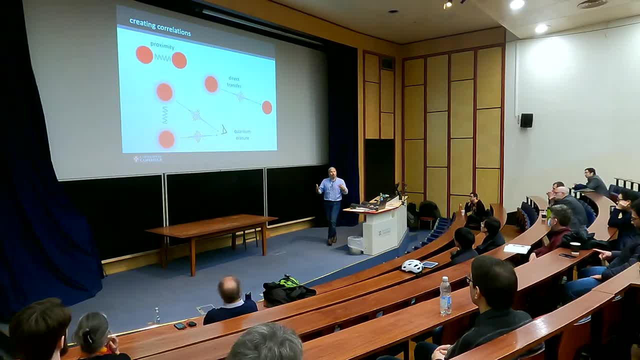 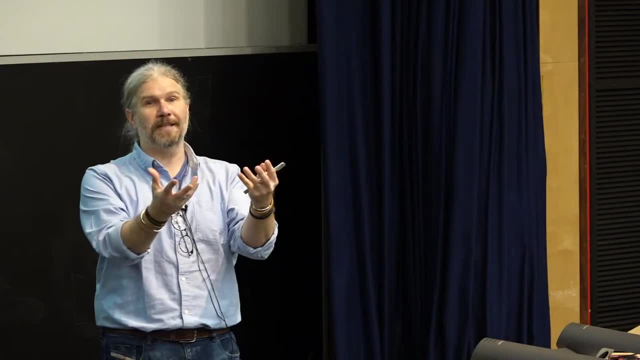 in a very advanced stage of making new materials in the lab. we're always doing this. This is all we do. We bring atoms that wouldn't normally naturally exist, we bring them together and then we have a new material. This, if we can achieve this over a very large, scalable format, we'll be making materials. 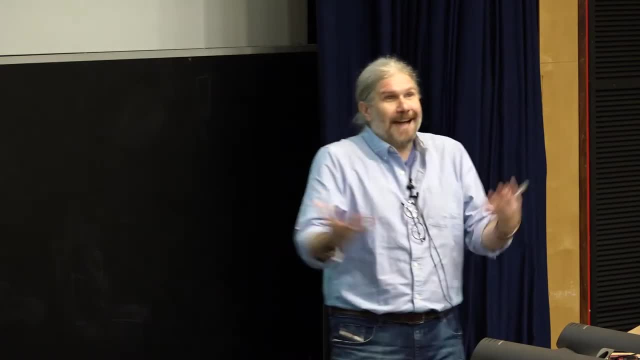 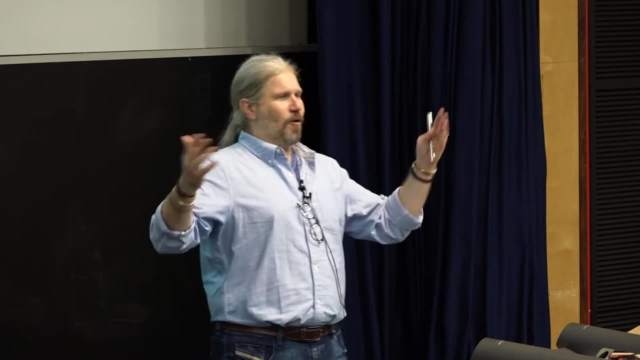 and studying their response, without ever actually putting things together in the lab. See how attractive that is. I could have stood up here and the first slide could have been: quantum networks are exciting. we like to do quantum networks, but I didn't. There is more to it. 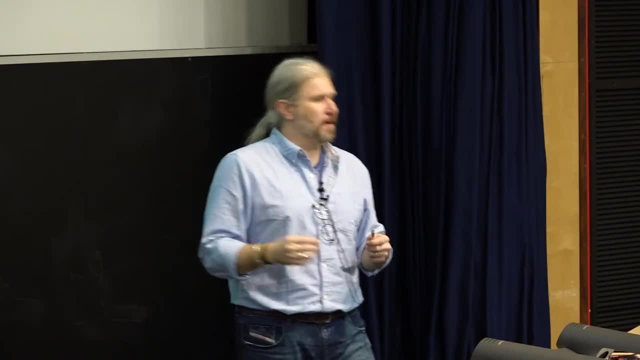 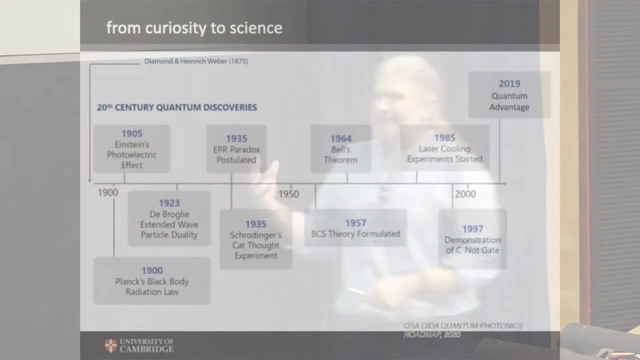 if we can get to the large scaling than just building quantum networks for an application. So it's good for science as well, to our understanding of matter. So let me go back to this Again, this history. we always treat it as you know: fundamental science, science. 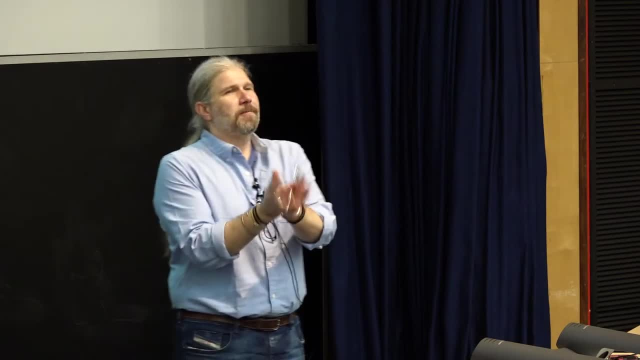 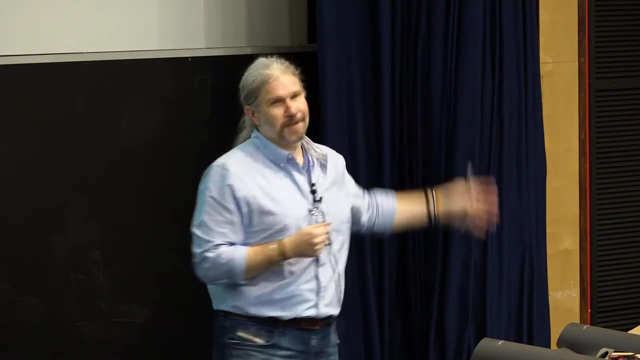 leads to technology. you develop science, probably out of curiosity- blue skies research- and then you find a way to use it for some application and you develop business based on that right, And this is a very nice. this is from the Society of America website. it's: 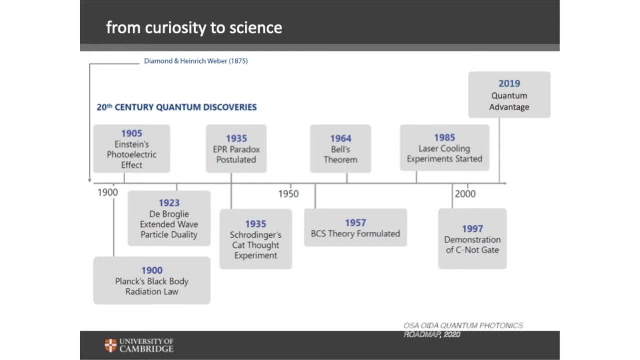 a nice flow of, I would say, randomly highlighted advances in quantum physics, mostly related to light of some sort, And it, of course it all starts as with our usual, let's say, mainstream education. all starts with Planck's Black Biter Radiation, and then the photoelectric effect, where he 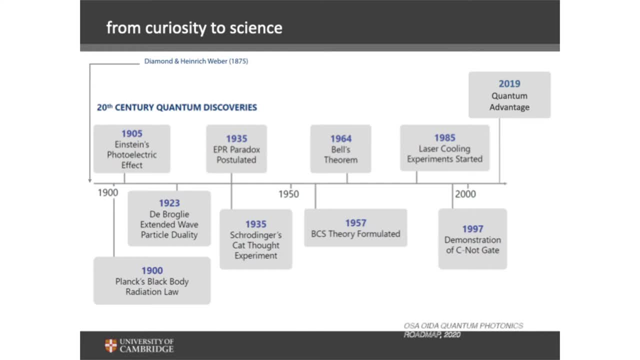 got the Nobel Prize for it and so on and so forth. But I'm adding here which I'm going to use later on. I'm adding here one more date: 1875, Heinrich Weber. Does anyone know what Mr Weber did? 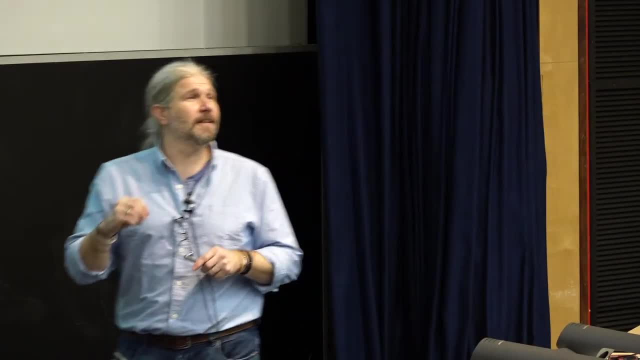 Mr Weber measured the heat capacity of a whole energy plant, and he did it in this example. Mr Weber measured the heat capacity of a whole energy plant and he did that in 1875, he did that in 1875. 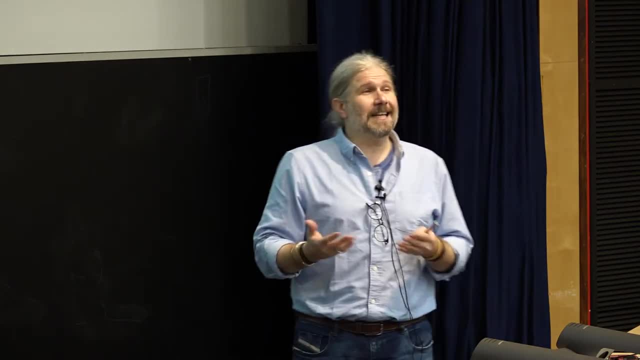 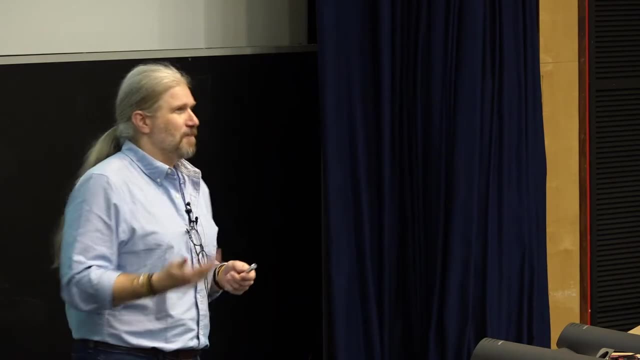 of things. and here's- actually it was one of the people- that show that heat capacity of things is quite boring, because it always comes out roughly the same value- three times a constant, three r or three kb balsam constant- in the end. so it's like it doesn't matter what temperature you look at. 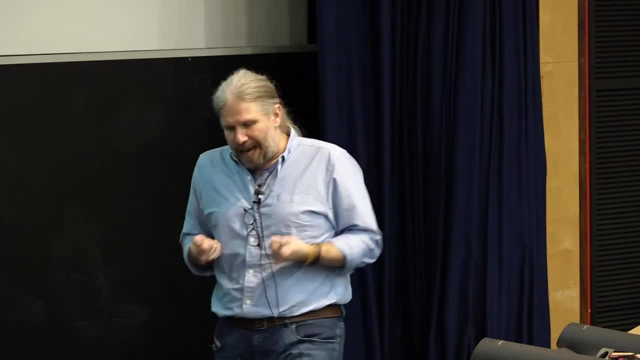 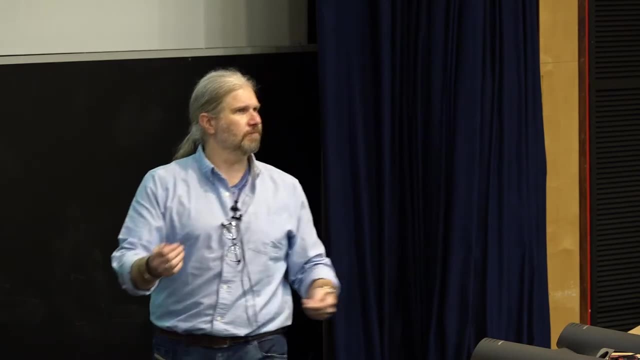 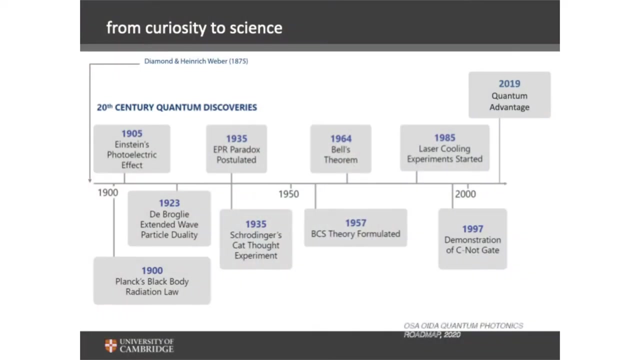 every material is roughly the same. what is heat capacity? how much energy do i put in so that the temperature of this matter, of this object, goes up by one degree? it's a simple question. what he showed in 1875, now this is prior to cryogenic experiments. this 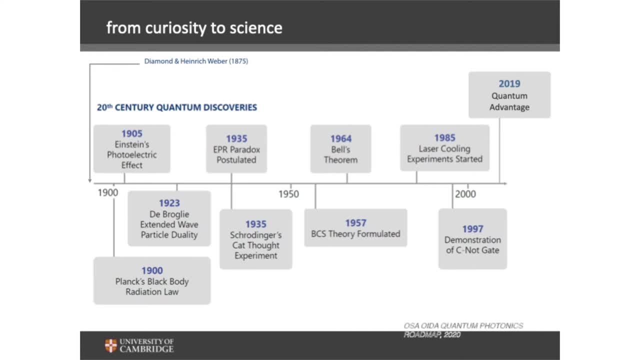 is prior to uh, liquid helium, liquid nitrogen, right. so 1875, he had to wait for winter to do the experiments so he can get some ice in large, large quantities to do the experiments. and summer time is, you know. now here we say summer time is research time for us, but actually summer time 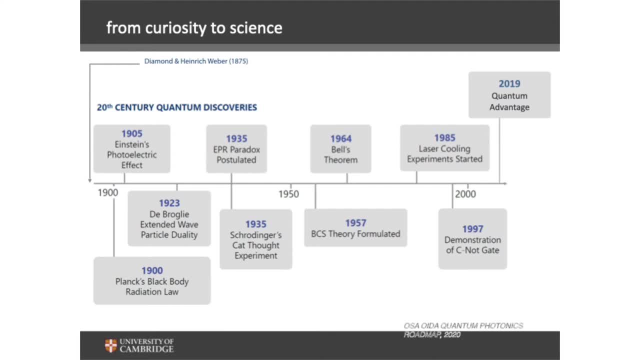 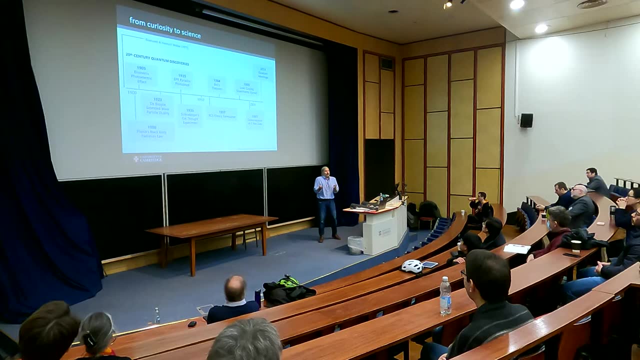 then it wasn't research time. so what he showed was diamond. specific heat was temperature dependent. so how much energy you need to put in to increase temperature by one degree depending on what temperature you start out with- and that's that's odd, because classical physics does not explain that at all. so that was something wrong. and what made einstein tip? 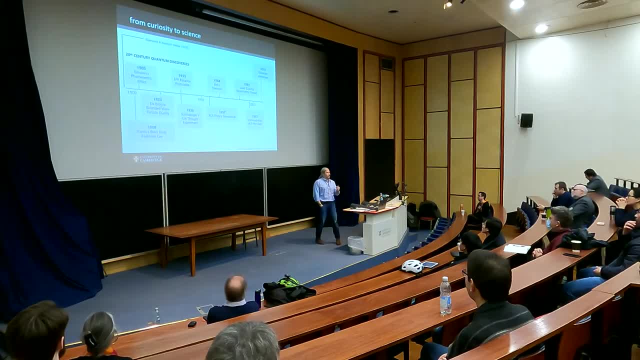 to the side of quantum for photoelectric effect 1905 and the concept of quantized radiation was when he realized that he can explain what happened to diamond specific heat by quantized vibrations phonons. so once he saw that fundamental particles the way we describe things if we quant. 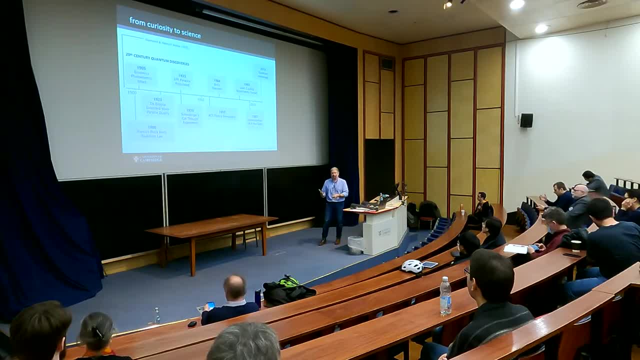 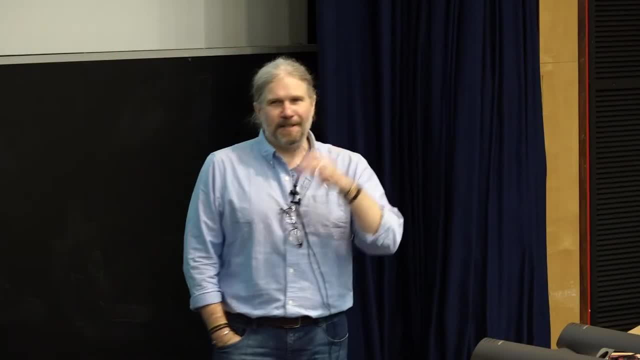 quantize them. we do see things that match with the physical reality. uh, that was it. he said. okay, so we're going to go through this, this particle nature of radiations and waves, and that triggered it. so that's the, the photoelectric effect. i wanted to say diamond in here because i'm going to use 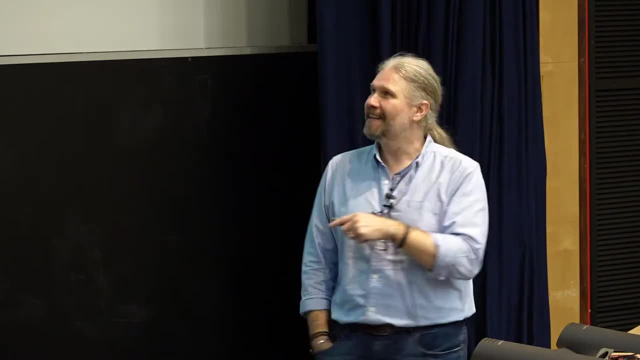 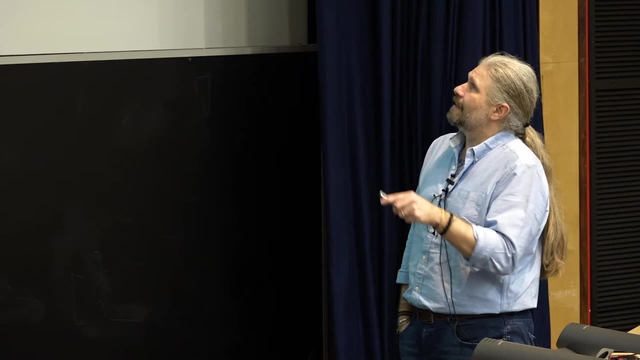 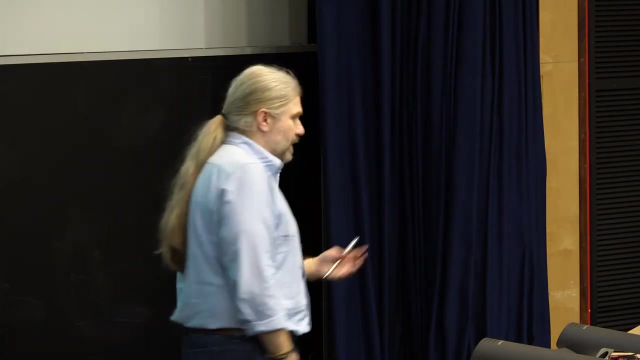 diamond later on in the talk, so it's going to come back. diamond has played a key part in many, in many, and here what you're seeing is in, in, in astonishing 100 years. we're talking about quantum advantage as as something that's realizable in the lab, in the first experiments and then 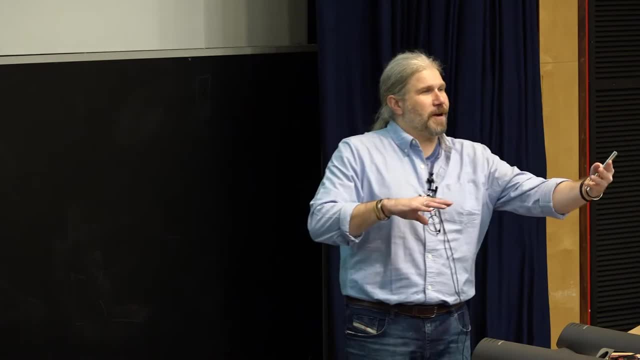 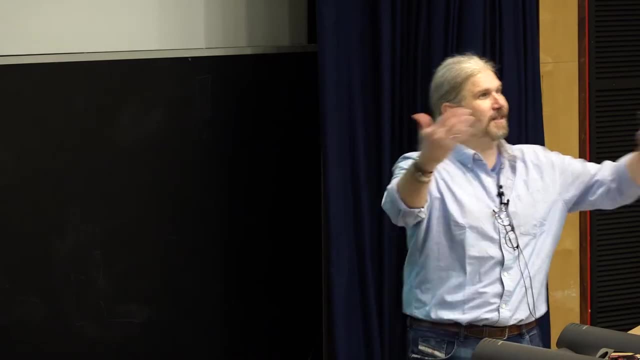 what will happen of course is: uh, you will show, demonstrate quantum advantage, then they will demonstrate a better algorithm, classically, that beats it, and then there will be another quantum advantage demonstration, and so on, so forth. so both classical and quantum world worlds propagate. but that's for the computing part, the 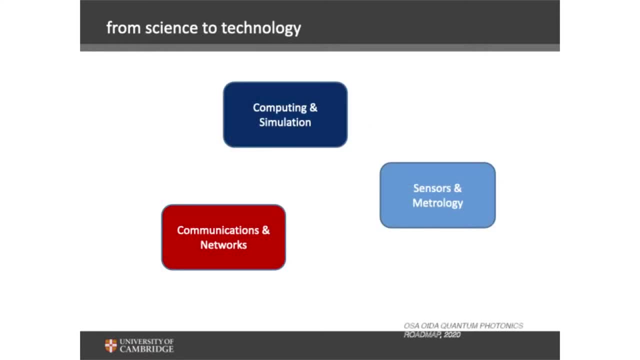 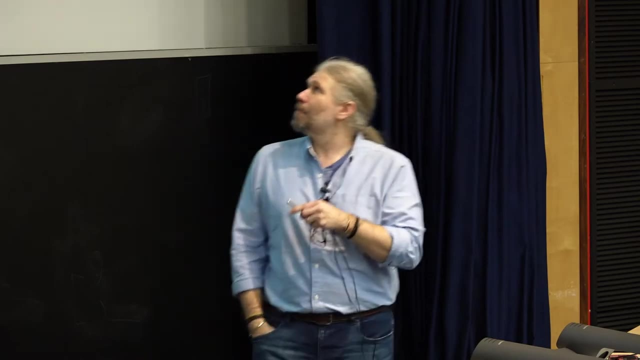 three main areas are expected from science to technology, from curiosity to science. we've seen, but science to technology. there are generally three areas in quantum technologies that, uh, that we would talk about. one is computing and simulation, another one is communications and networks and the third one is sensors and metrology. so i'll try to show is a bit of glimpse of where. 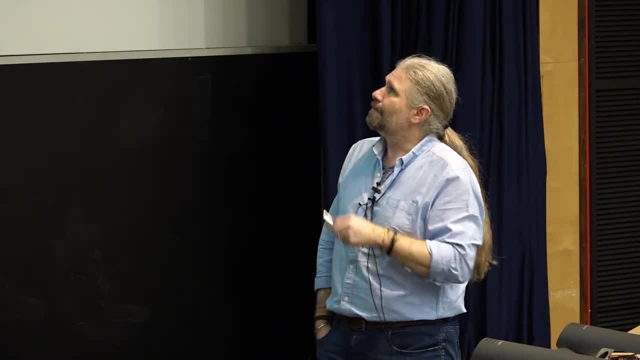 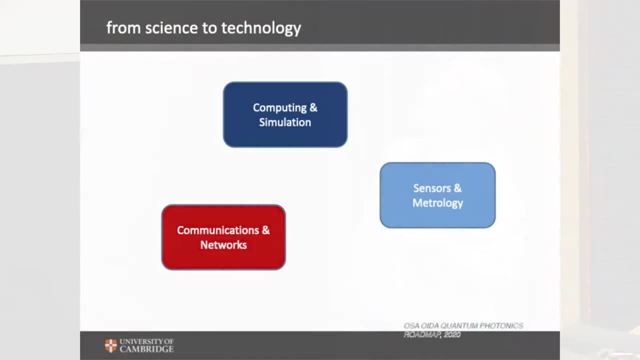 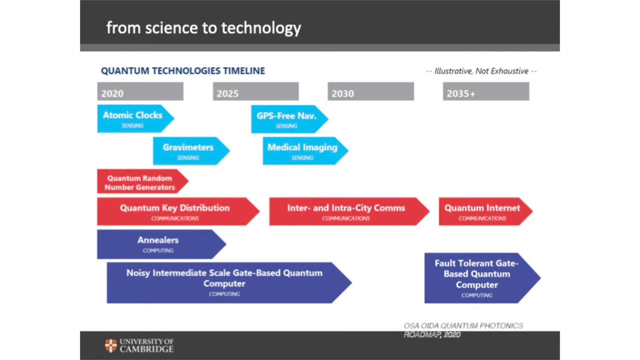 we are particularly with a material system like diamond for uh, for all three of these right predicted in 2020 that we would have inter-city communications till 2030 onwards and quantum internet in 2035, plus and annealers up to here. so on and so forth. 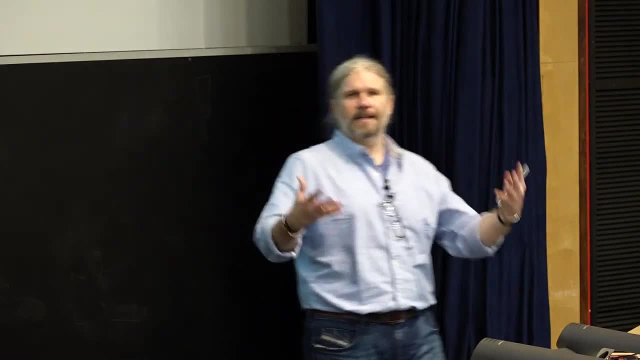 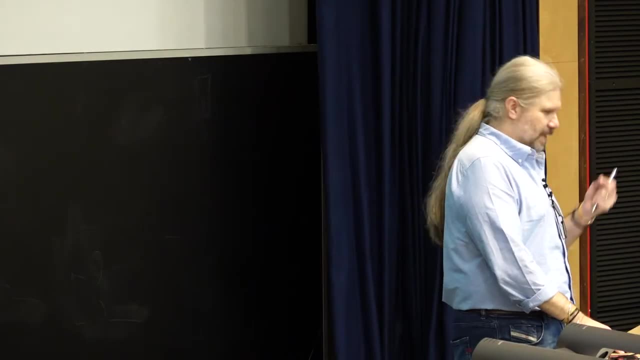 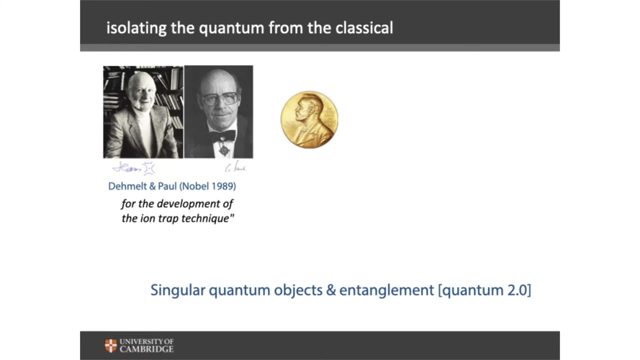 So we've moved on from curiosity to actually doing things with a reasonably well-defined roadmap, But it goes down again. the topic was quantum optics. so how does quantum optics come into this? It boils down to actually this work by these two gentlemen, Dan Melt and Paul developed. 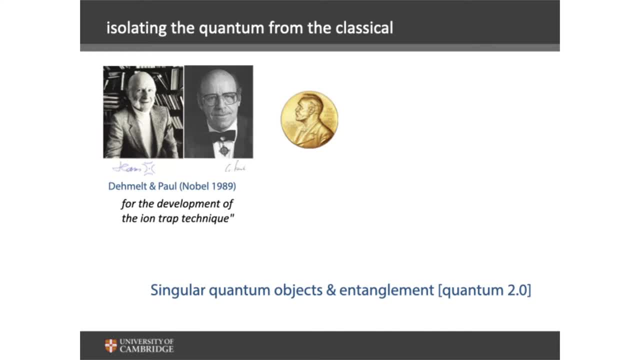 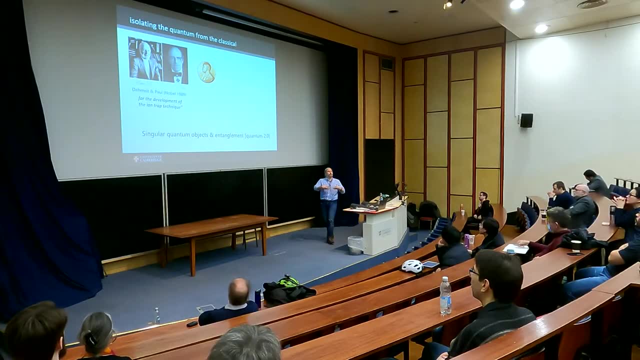 a way to actually finally trap a single quantum object. Until that time they got the Nobel Prize in 1989, the work was earlier, but until that time we had beams of atoms passing by when you heat an oven, and then atoms escape. 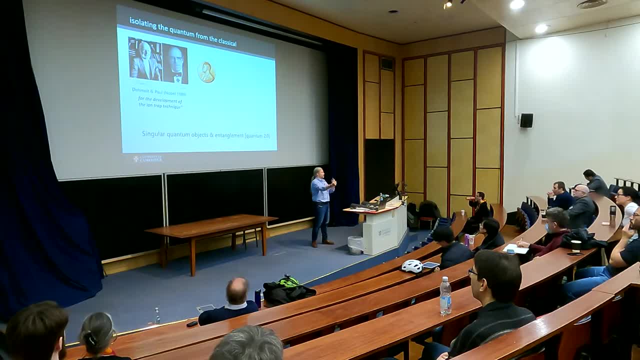 It was never a single isolated quantum object sitting somewhere where you can talk to and do work with it and study its properties. So it's the first work that actually trapped a single ion. you remove an electron, you have a charged particle, you create an electromagnetic trap potential and the ion just sits there. 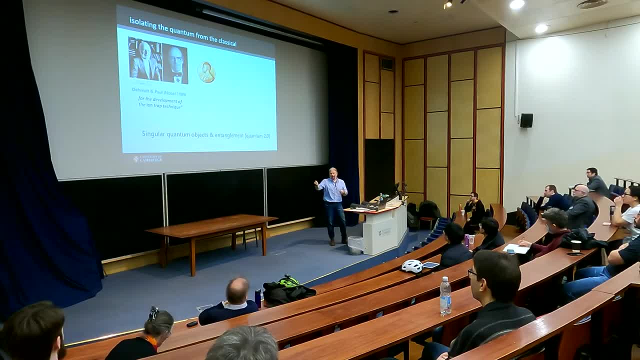 and can't move. And actually now these days it sits there for hours and hours. so it's the same ion all the time They trapped. and if you look by the way, it's a little anecdote: this was his original. 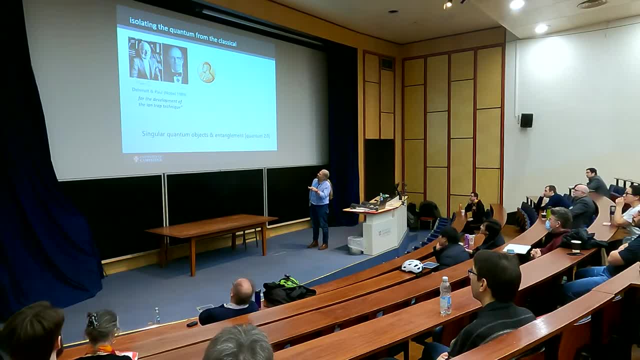 signature- Dan Melt's original signature- and after he trapped it, he added that to his signature. That is the ion in the middle And that's the trap. That's how he's actually trapping a single ion. So he changed his own signature because he realized the importance of this discovery. 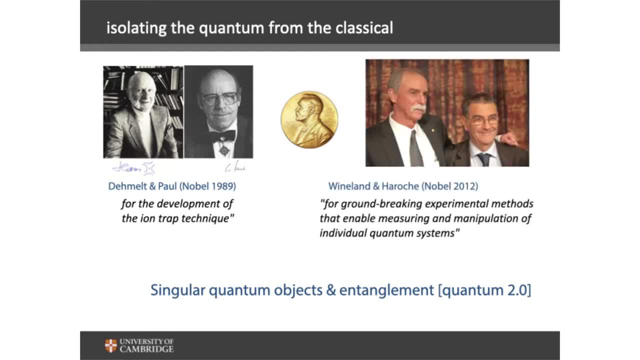 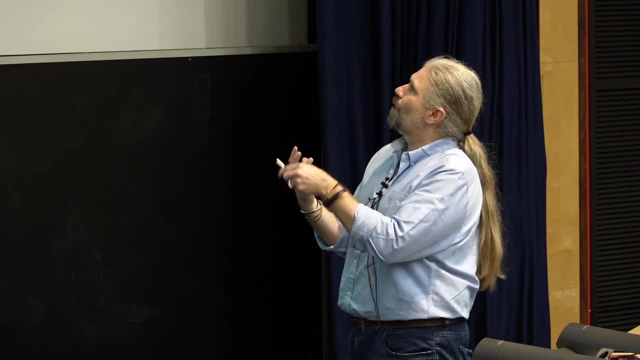 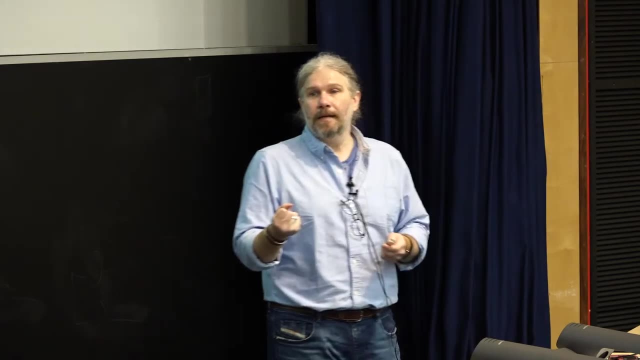 A second Nobel Prize topic was on not trapping that single ion but introducing the full quantum control tools that we have to be able to control these individual quantum systems. So isolating the quantum object from the classical actually has been only quite recently. It hasn't been since the 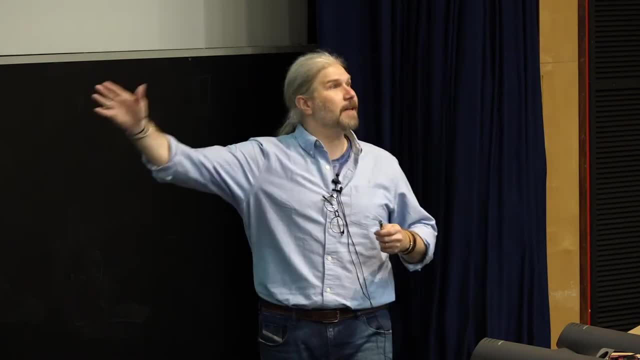 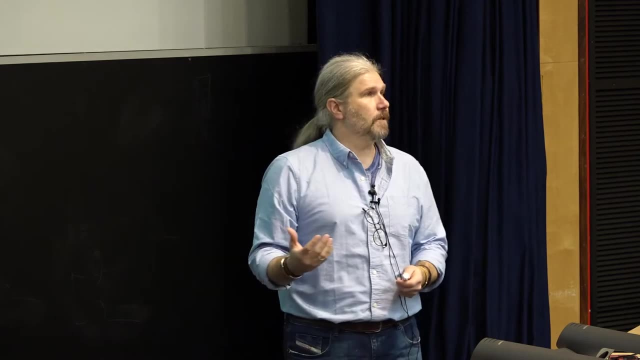 1900s The concepts. the curiosity part goes back to 1900 early. but actually being able to play with these things in the lab isolated, is actually not that far off. This is only in the last 30, 40 years. we have access to it. 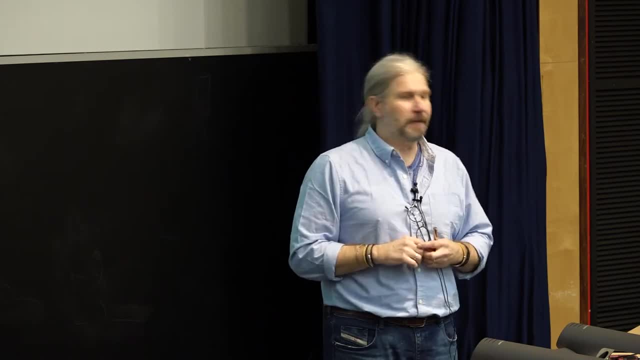 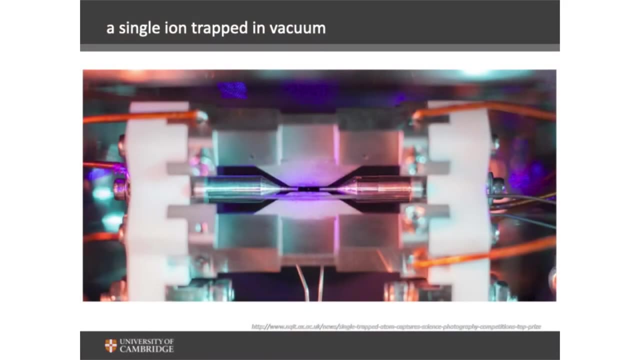 Well, laser is 1960, so we wouldn't have the lasers anyways, You wouldn't be able to do this. So this is Dan Melt's signature. You see the trapped ion right there, just from the Oxford group. trapped ion group. 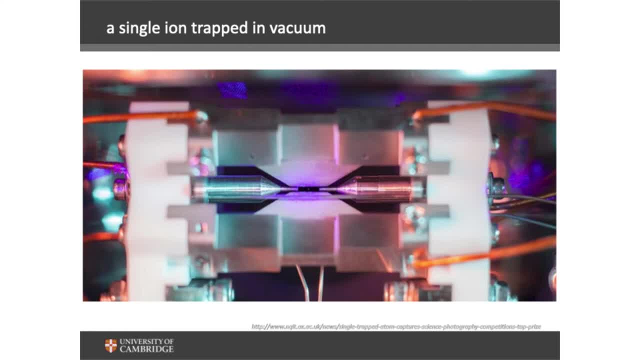 and this is the equipment that goes around to trap it. And in vacuum, in isolated vacuum, And then you do all your operations with it. The ground state is spinactive, so you can code information into the internal states of the ion as a qubit. 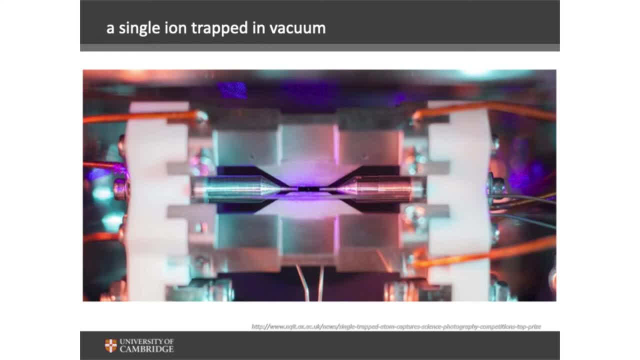 And it has optical transitions. so light comes out, and the light that comes out is related to the internal degrees of freedom. That's the So, in other words, that's the red blob And the pink hue is the photon that comes out of it. right? 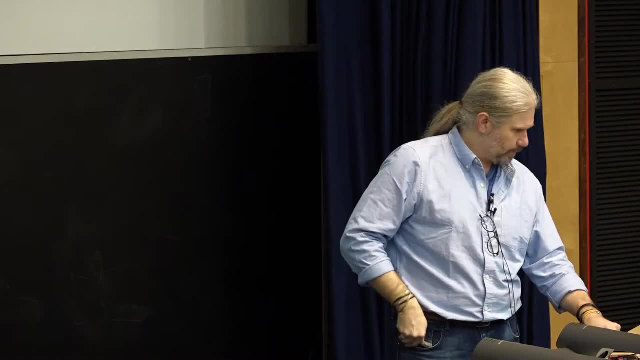 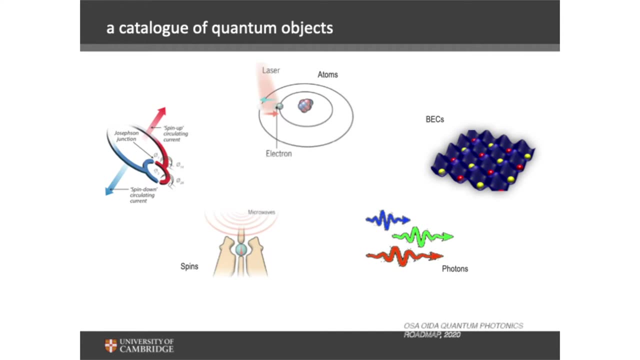 So that's what it actually looks like- those red blobs. There are many realizations of quantum objects now Isolated quantum objects, so trapped ions or atoms is the one that we start out with Photos themselves. as we know, you can't really trap them anywhere. 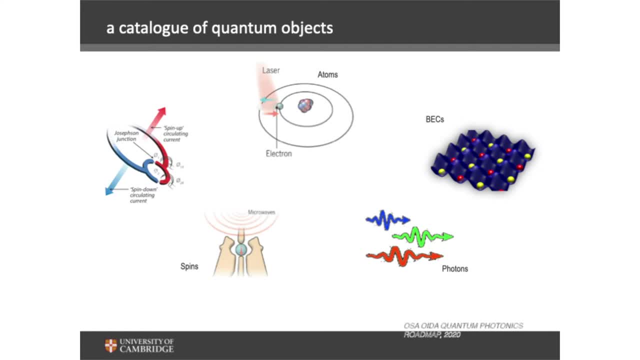 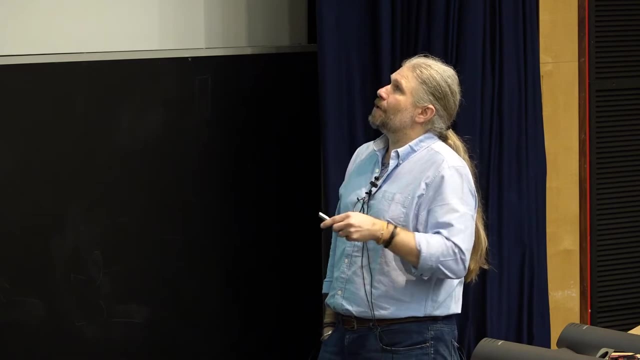 They tend to travel at the speed of light, But they're quantum objects, individual quantum objects and early quantum optics experiments relied heavily on photons using nonlinear optics. actually, Parametric down conversion was a process that generated entangled photons, Spins located in solids, superconducting systems based on Josephson junctions, cold atoms. 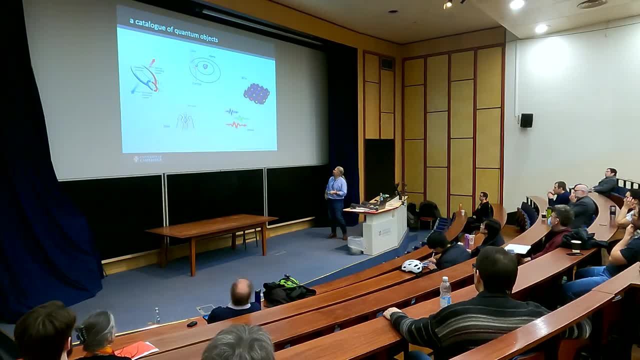 in optical lattices to create artificial lattice structures and whatnot. these are all different platforms we now have that I can say are isolated quantum objects we can access and measure And any other- even though I say isolated- any other leftover interactions they have. 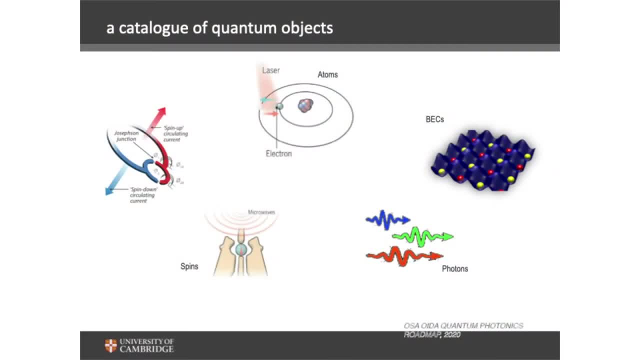 with the rest of the environment will treat them as dephasing or coupling to the environment, But the coupling is strong enough To us that they survive as strong promising candidates to realize applications with. This is that red blob in the pink hue again. 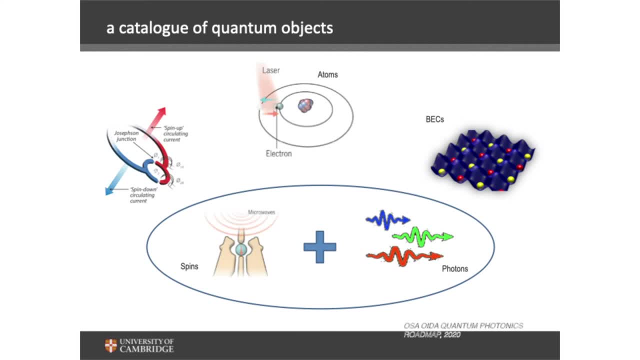 If you have a solar system, rather than a trapped ion, a single electron spin, for example, inside, buried inside a matter that is otherwise spin, vacuum, that does not have any containing, spin this little guy over here, trapped. if it is connected to photons, that gives you 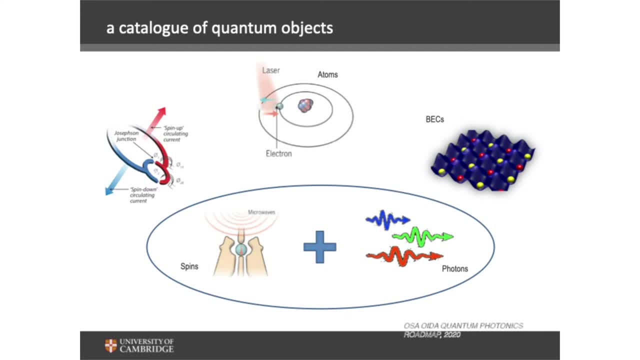 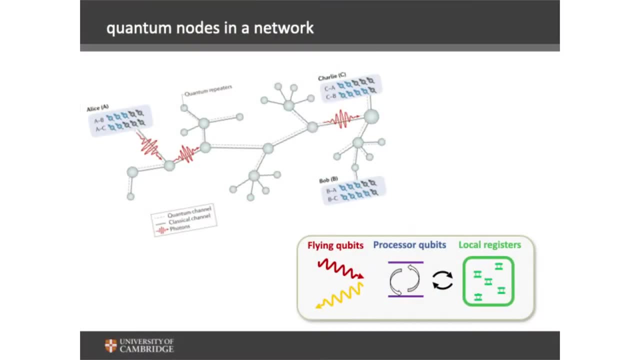 the spin photon interface, or it's this, the red ball with the pink hue. Why is that relevant? In the same concept as I was promoting quantum networks, you can then couple these blobs to each other by quantum radiation, by quantum light, and each of these blobs can be can. 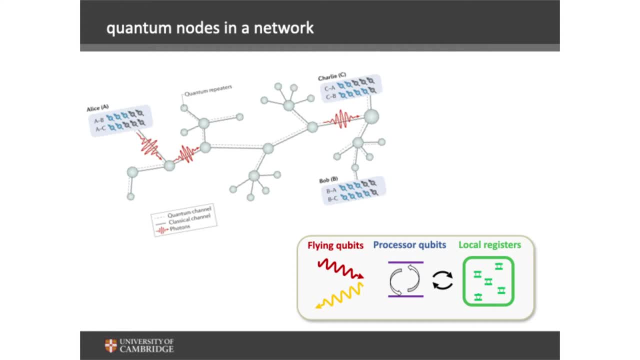 compromise: effectively a processor qubit, something that's your controlled qubit that you're interested in and coupling to the photons that transmit the information back and forth between different levels. So you actually need a local registry nearby and physical realization for these things. 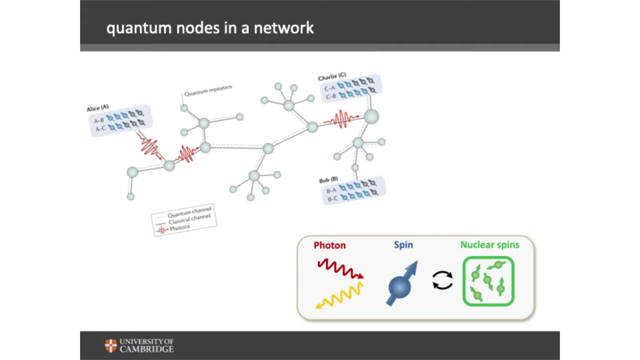 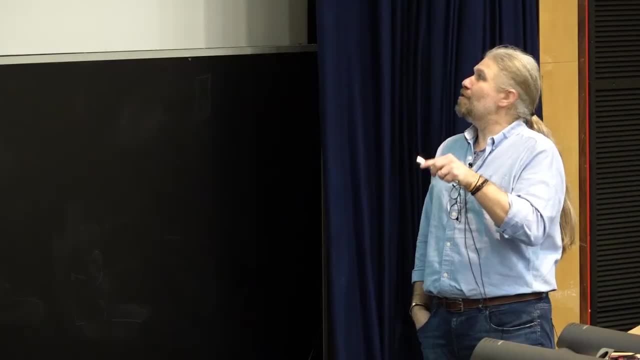 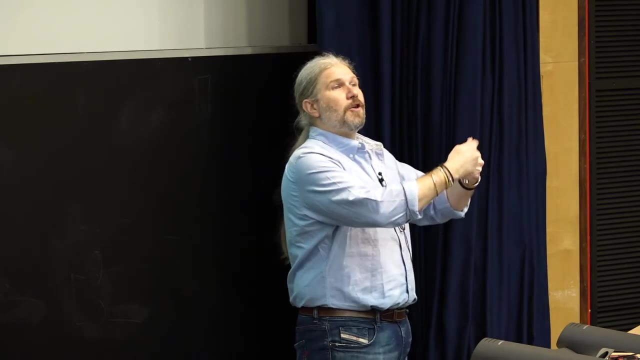 usually this is the fashion of the day- is usually photons interacting with a single electronic spin, well-defined electronic spin in a solid with a nearby nuclear spin ensemble that we can access- three, four, five, seven, whatever The electron talks to the nuclear spins. 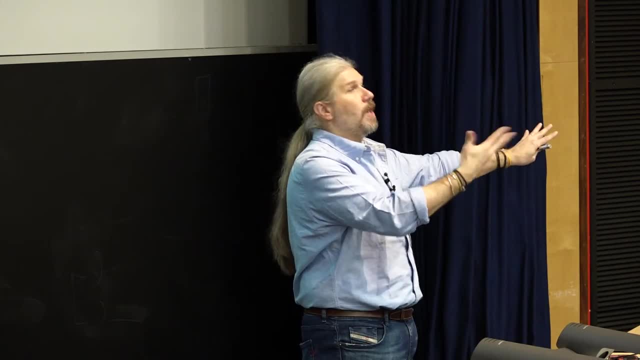 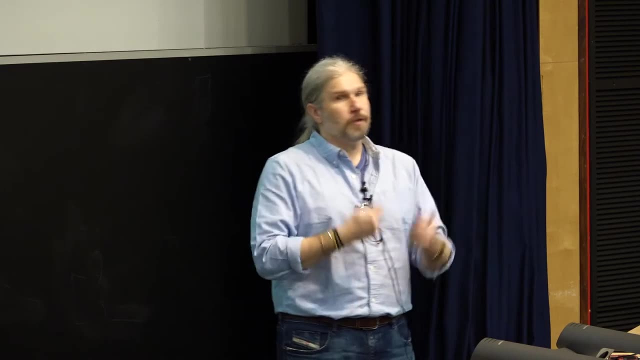 You can encode information into nuclear spins, store it. nuclear spins are well isolated so they're quiet. You can store information for a long time, whereas your electronic spin is fast, so it actually is good for processing and distributing information, essentially. 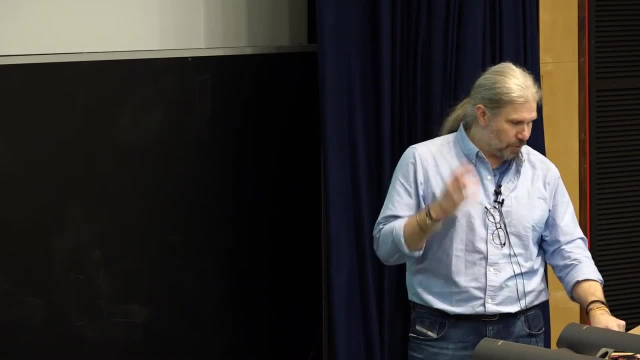 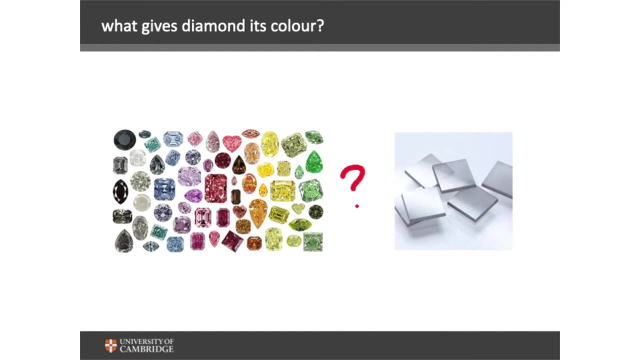 So what kind of a material system can host this trio? Turns out, diamond is a good one, and delta is one of the leading places for diamonds, so I'm very happy to follow Barbara for this. Normally, when I say diamond, this is what you think of, right? 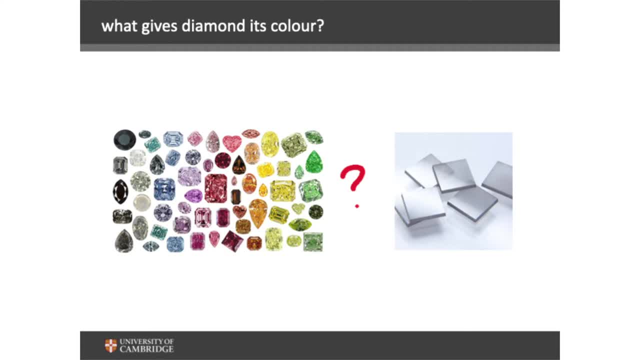 All the colors that you can imagine, But actually the diamond we work with, The diamond I really like is this one where there's absolutely no color, because color in diamond means anything but diamond. So if diamond is colorless, what makes these diamonds interesting is their impurities. How much you deviate from actual pure diamond is what makes it attractive. so we like our impurities. Depending on the color, you get different. depending on the atoms you put, other than carbon, you get a different color. Pink is nitrogen. 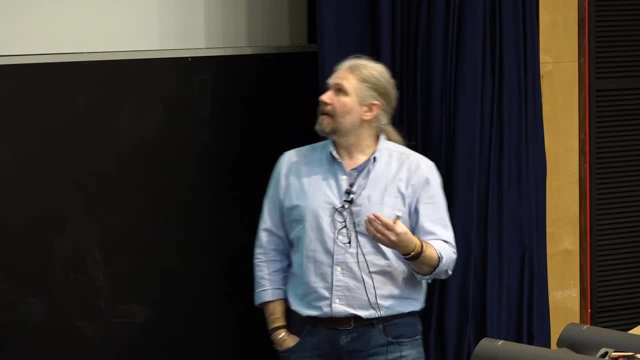 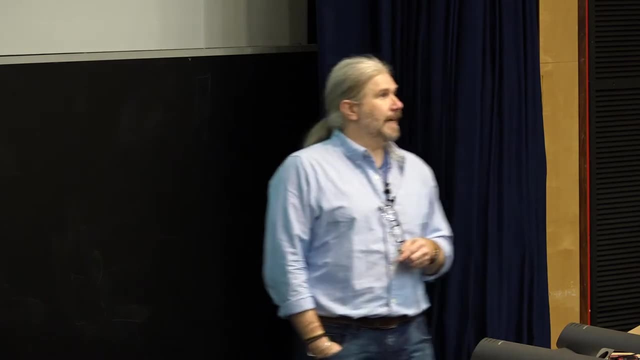 So if you put a lot of nitrogen inside the carbon lattice, you get pink. If you put silicon inside the carbon lattice, you get yellow, And if you put boron, you get more bluish light out. So next time you go to a museum or something, you see a nice big diamond piece and it's 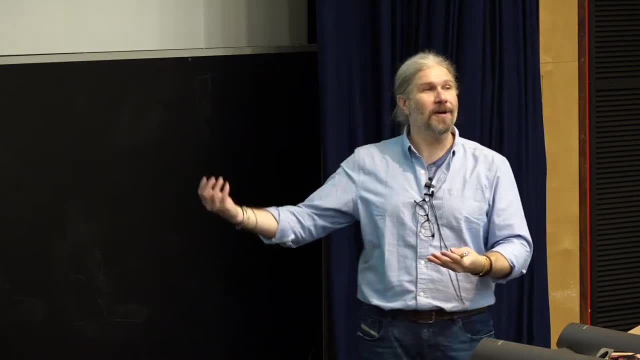 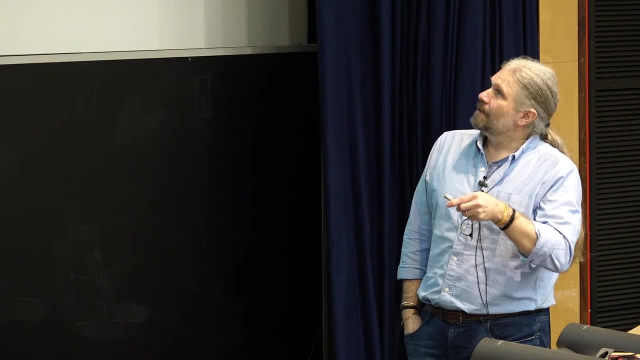 got a hue. you know what atoms are there. They take it away from pure diamonds to give its color. The thing that's interesting is to actually work with these diamonds: pink hue, but only one atom at a time, Well separated from each other. 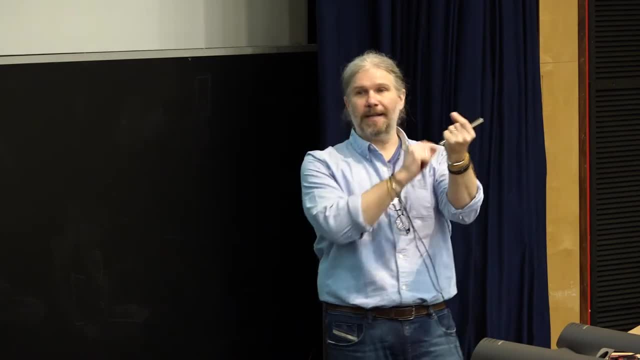 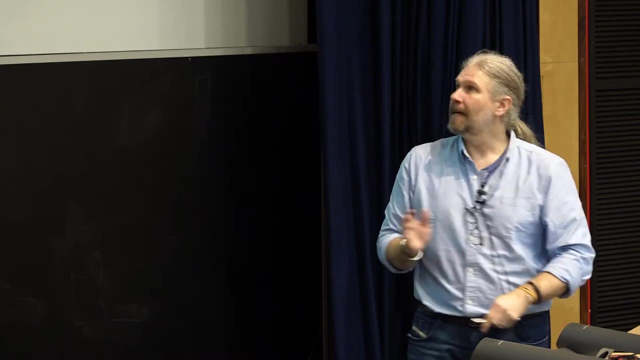 So I have just like a trapped ion. I only have one atom, with the one electron that I'm going to talk to, but nothing around it. So when I interact with it it's completely isolated as a quantum object And that's called a nitrogen vacancy center. 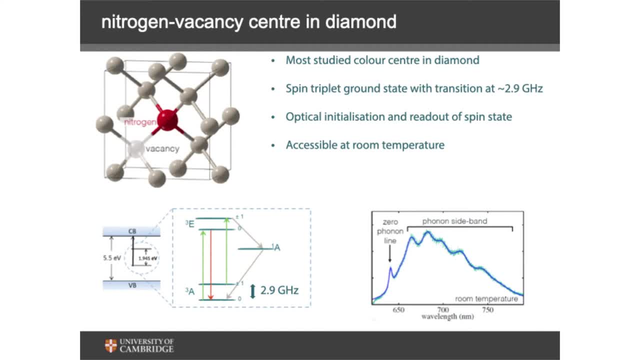 It forms in diamond. it's pure diamond. but instead of two carbon side by side, two neighbors, you remove one and replace it with a nitrogen And then you remove the neighboring carbon. you don't put anything in there That called a nitrogen and a vacancy combined. 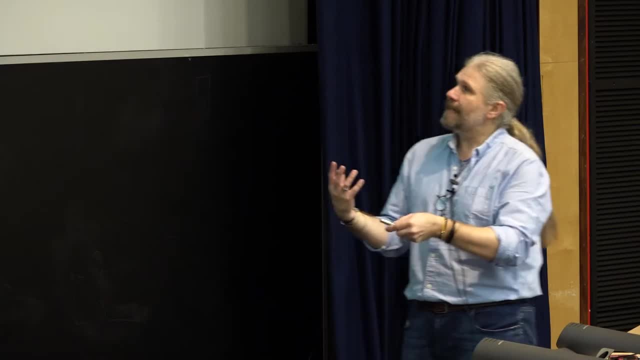 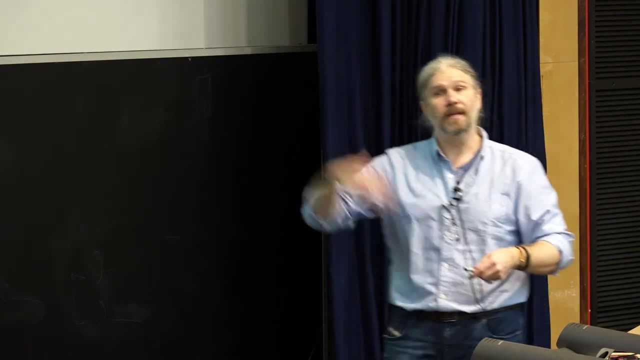 So, again, the reason I wanted to show you this is because this is very, very simple. So, as you can see, the hydrogen one side is optically active. It has a spin ground state with some splitting, so it has some structure, but it's got an active. 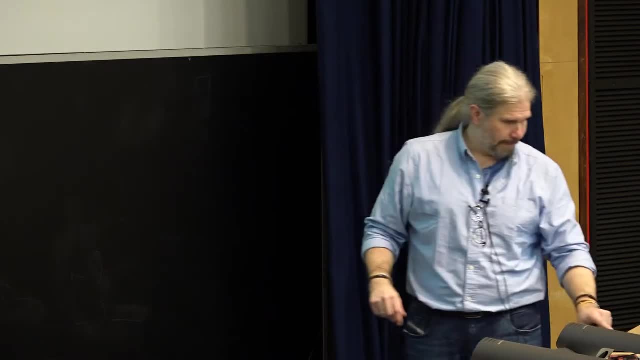 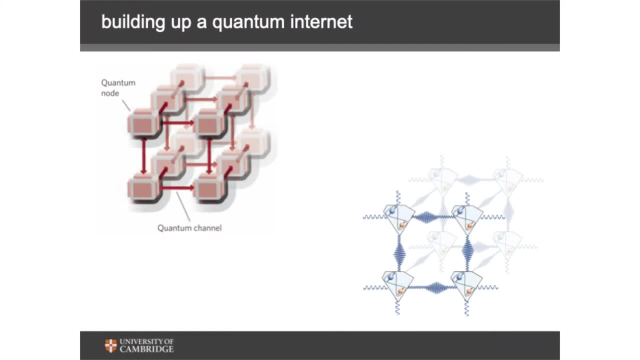 spin in the ground state and optical transitions that link that spin to photons. That's all we need to know. Once we have that, we can start generating effectively this concept of linking each one of those nitrogen vacancies. It's from Jeff Kimball's paper called The Quantum Internet. 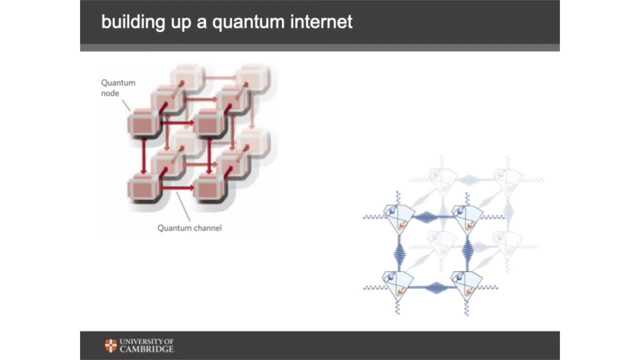 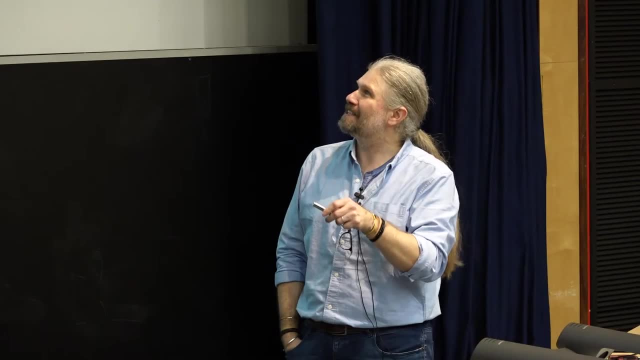 and red arrows. I said, if you have squares, cubes and red arrows, you're done. You can build a quantum internet. No one understood what an arrow is and we've been struggling ever since to build this thing up. But if you put a nitrogen vacancy center here, one 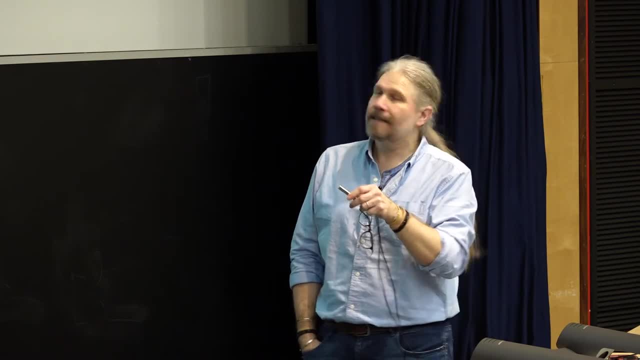 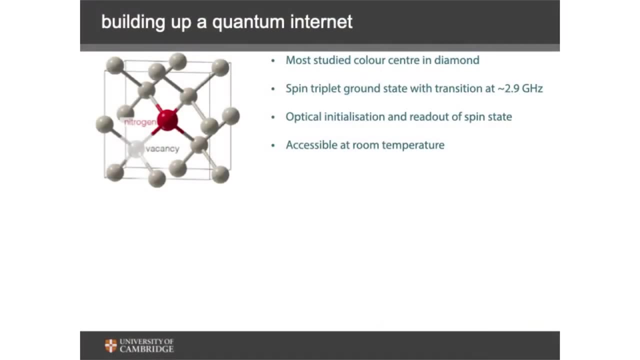 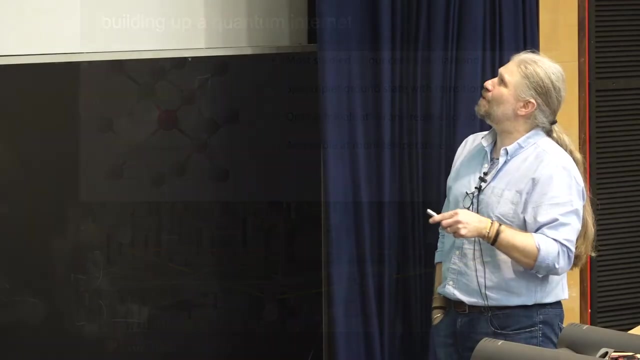 atomistic defect here and photons that come from it as the red arrows, you're there. Essentially, that's the motivation And that's exactly what Delft did. Ronald Hansen's group and a large team and collaborators have actually used, created this A, B, C. 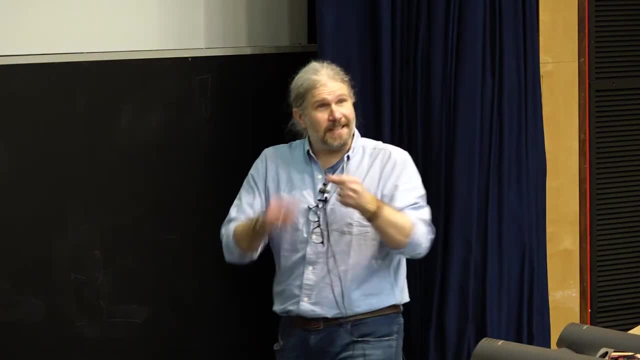 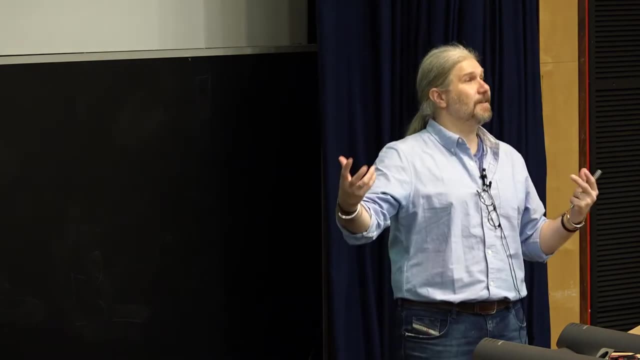 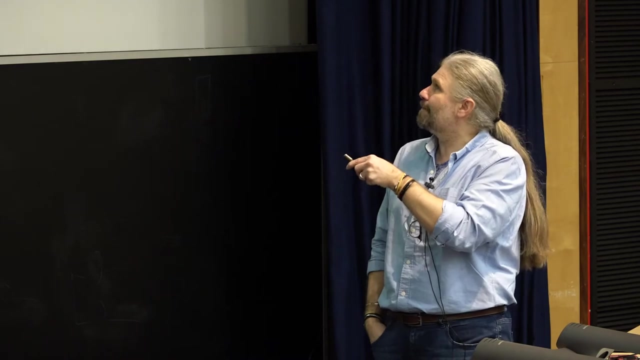 three locations where nitrogen vacancy centers. these little diamond chips are distributed in different locations and by simply exchanging light they were able to create entanglement correlations between these two spins that are not proximal to each other. The only thing that mattered was taking the light from this point to that point, or this point to that. 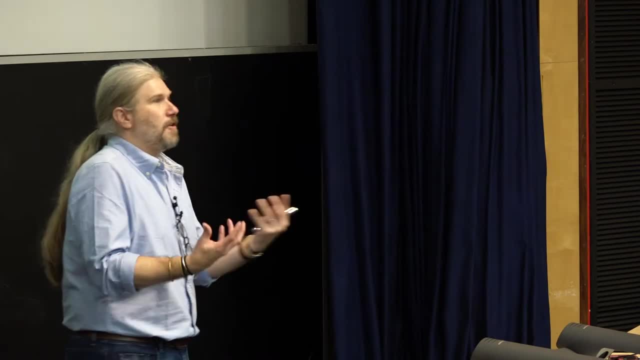 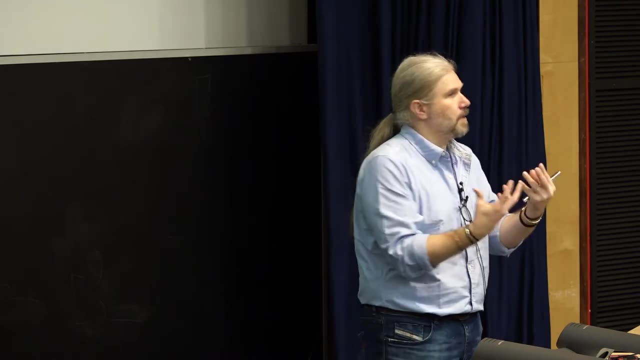 point. But being able to do this, they removed the spin and they were able to do this. They created a three-particle correlated state without the need for particles to ever coming together to interact with each other, and that's the power of quantum network. 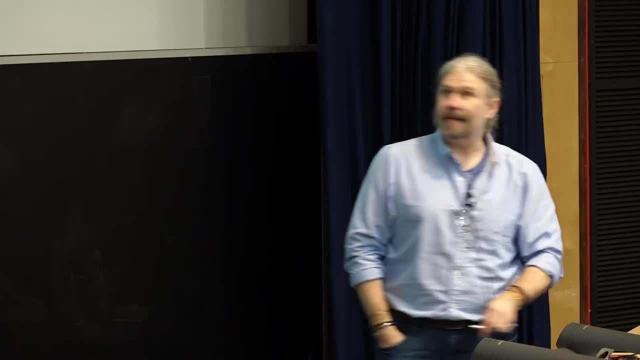 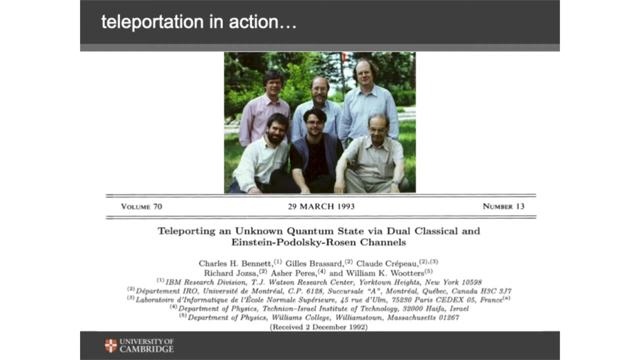 And through this, of course, one of the things they realized beautifully is going back to this concept of 1992, 1993, amazing idea of using entanglement to do something. I think, if I'm not mistaken, this might be one of the first examples of here's quantum entanglement. 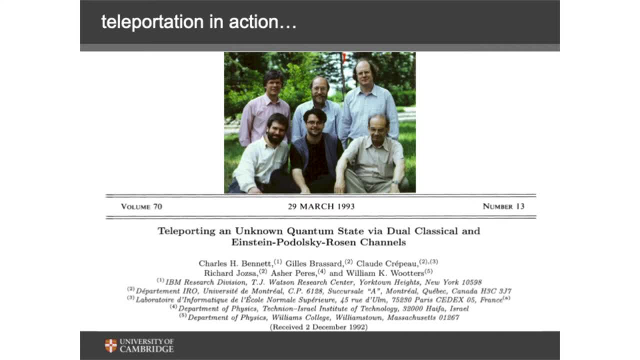 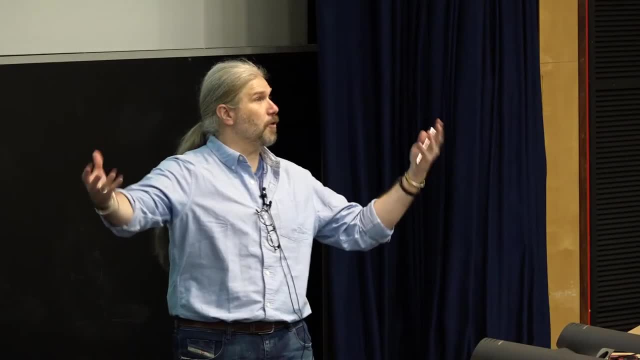 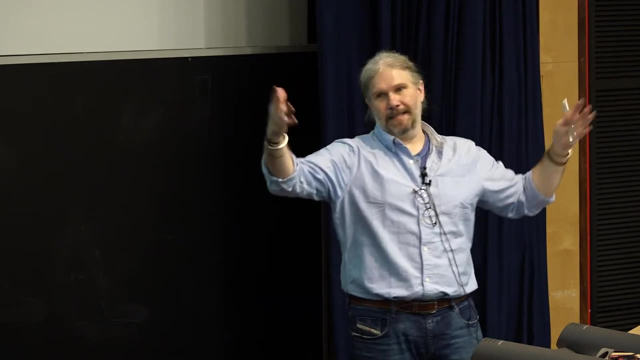 what can we do with it. And they came up with here's quantum teleportation as something that could be achieved if you have a resource of entangled particles in two different locations. So if you provide that as a resource, you can then use it to teleport information from A to B instantaneously. That was the claim. 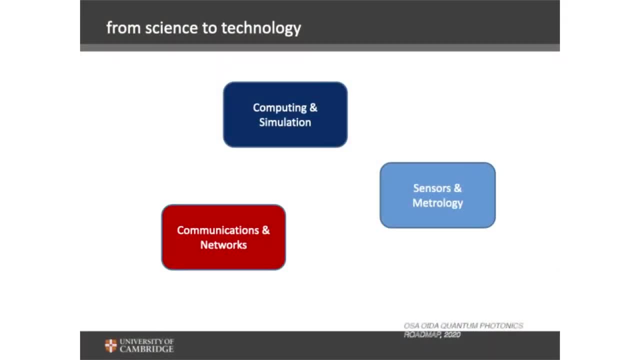 So, coming back to this, so do we have a quantum network? Yes, we do. We have a three-node quantum network. now There's only one, It's in Delft. We have a three-node quantum network. It's operational, it's working and it's based on DIAMOND. These are color centers. 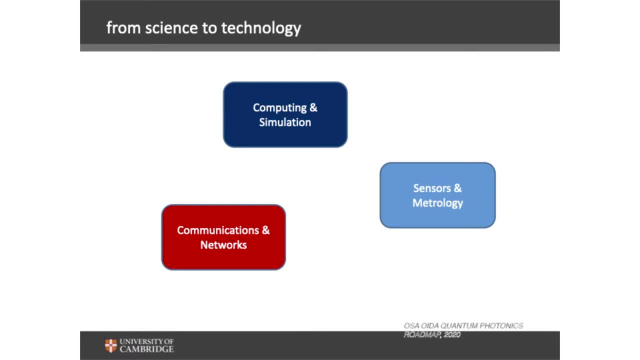 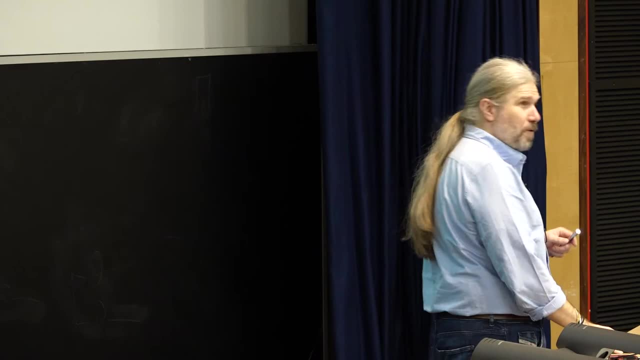 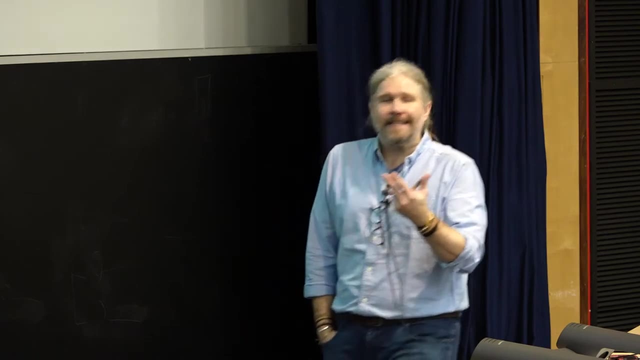 quantum objects in DIAMOND. So that was. I give that as an example for communications and networks. I'm going to move to computing and simulation, the computing side, following on from DIAMOND. actually, As we know, there are two, let's say two mainstream ways: quantum: 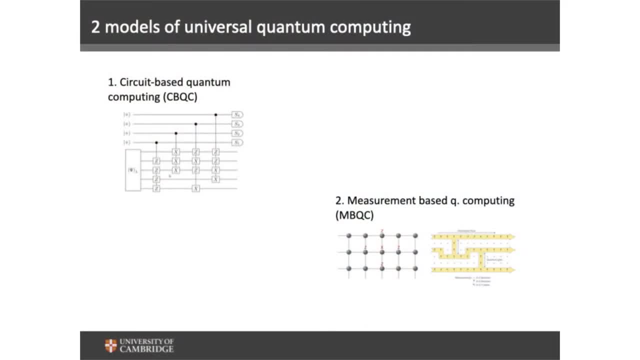 computing is viewed. You can have the circuit-based approach, the more obvious one, And then there is this measurement-based approach, where it requires providing resource into the system rather than controlling every single qubit, As long as you're able to dump the overhead of controlling all the qubits to the beginning of generating entanglement. 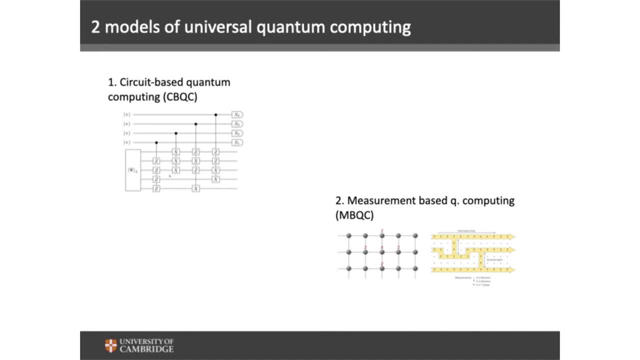 and feeding into a system. as long as you're able to do that, then you should be able to do a measurement-based quantum computation, And photons are more suitable for this because this doesn't require immediately interactions. It relies on measurement. We can measure photons. We can't get photons to interact with each. 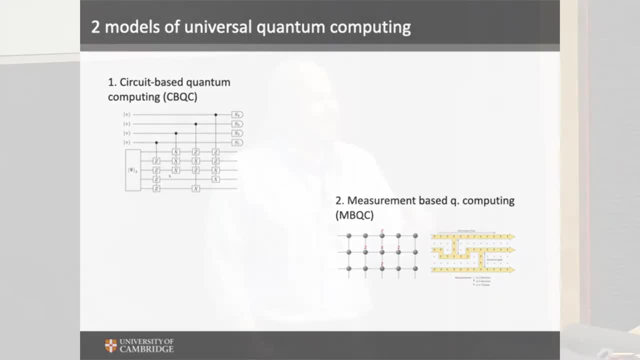 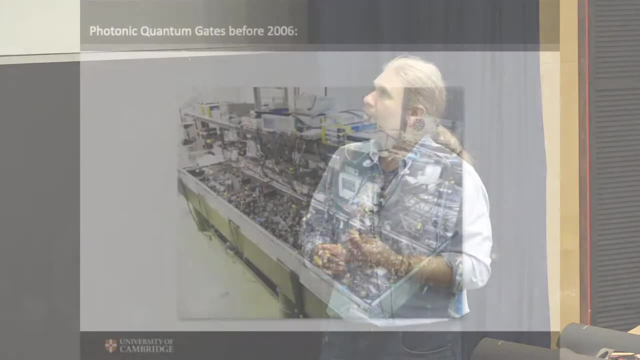 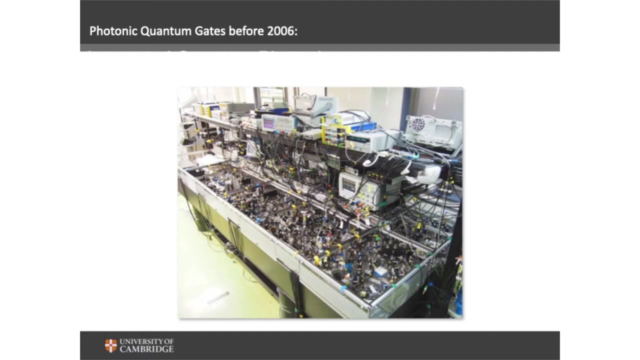 other efficiently. This requires interactions. It's difficult to make interactions for photons, but there's a way, And the way people have achieved it is using setups that look like this: This is purely for photon-photon interaction setups. This is photons going through this. 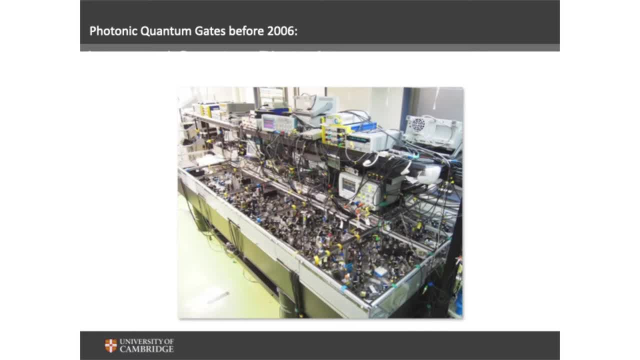 is called a probabilistic quantum computation approach. You use beam splitters, you use multiple options to actually evaluate, You have a full linear optic circuit circuitry and you pass your photons through and on the end you make a measurement. You make many measurements actually, but simultaneously. 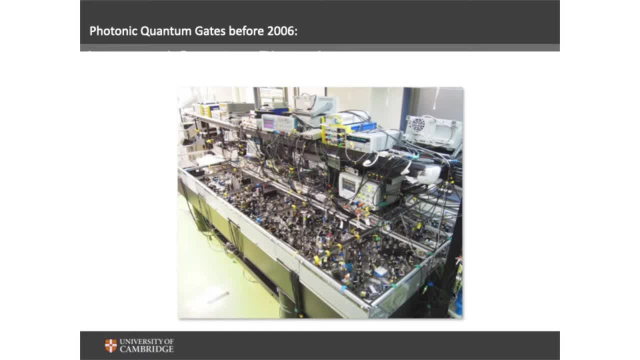 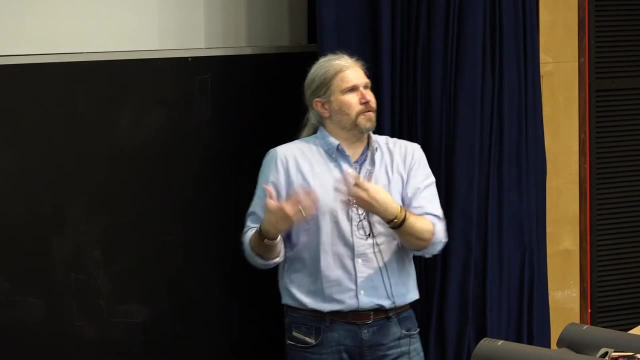 If you have made certain measurements and the outcome was a certain prediction that you had, then it means the channels you haven't measured are in a particular quantum state. So you can predict that quantum state with certainty if the other measurements give you the right condition. So it's a conditional measurement. You have to make some measurements. You fail most of the time because the whole thing is problematic. So it's a conditional measurement. You have to make some measurements. You fail most of the time because the whole thing is problematic. So it's a conditional measurement. You have to make some measurements. You fail most of the time because the whole thing is problematic. 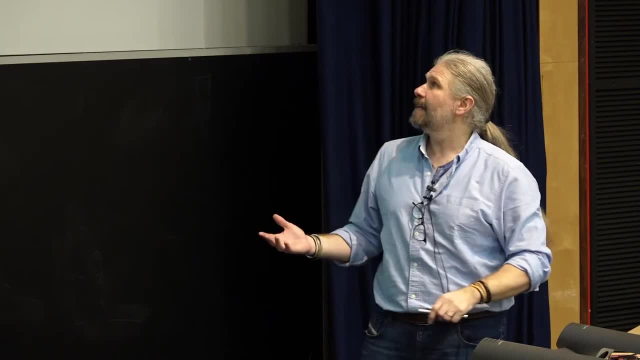 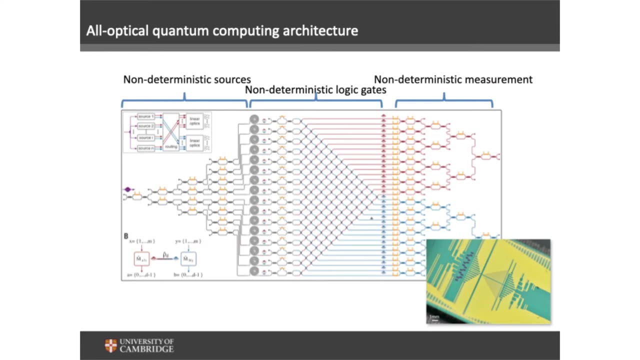 In fact, it looks kind of like that. That's what the setups will look like. These are all sources, non-deterministic sources, So sometimes you generate a photon, sometimes you don't. Non-deterministic logic gates. these are beam splitters. Sometimes they 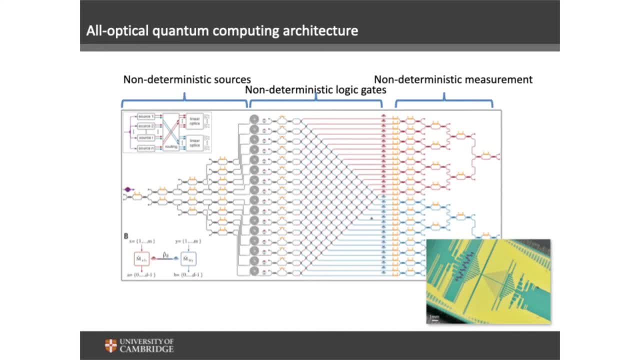 go left. Sometimes they go right. So there's ambiguity, But in the end these are detection systems. If you detect the right combination, the outcome is correct. So if you know the movie Anchorman, it's, It's 60% of the time. it's accurate all the time. 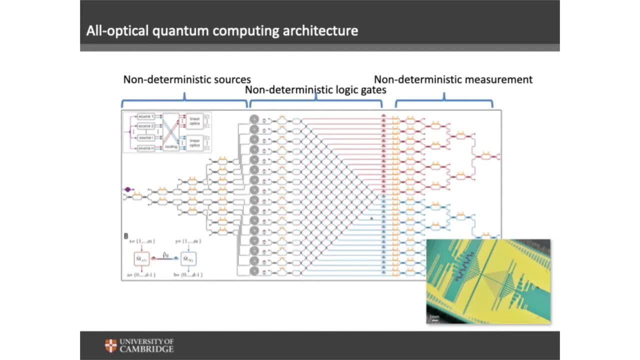 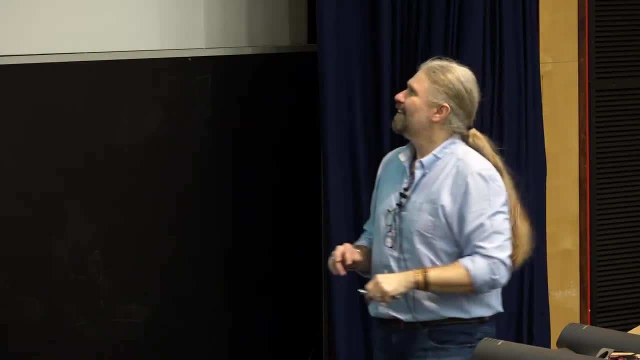 That's the phrase from the movie. So there's a low yield. but when you made those measurements you are 100% sure it worked. all right, 60% of the time it works all the time. This is a map. 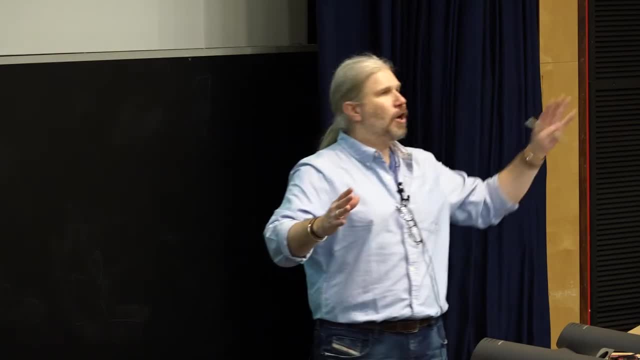 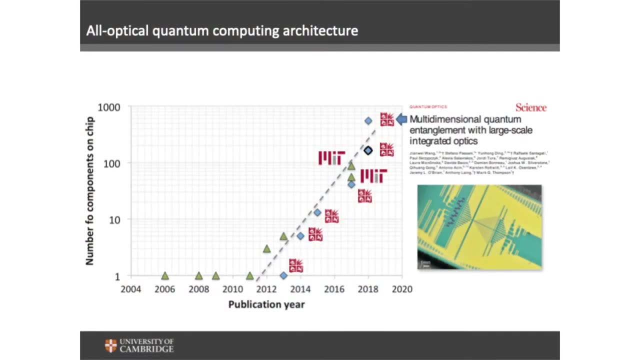 So this is on-chip quantum computation, one-way quantum computation approach. You feed the photos from one side, It goes through a process of a well-defined chip and it gives you an answer, like random world questions or traveling salesman questions, whatever boson sampling. 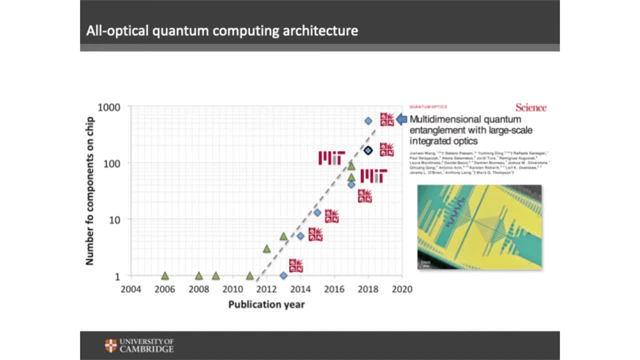 What I'm plotting here is complexity, number of components, on-chip. Complexity is a function of year for the non-deterministic probabilistic approach, And what you're seeing here is first initial test and then it kind of goes exponential, kind of like a Moore's law kind of thing, right. 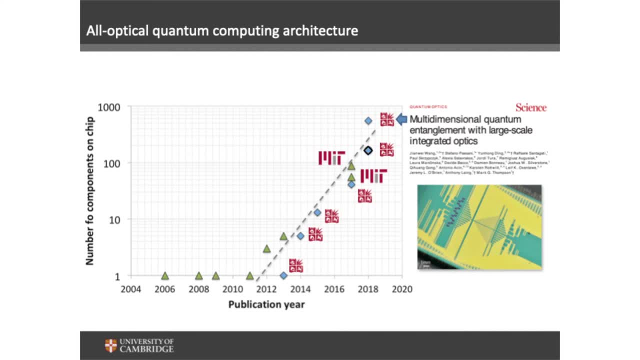 There's number of components on-chip where people have demonstrated many things, Bristol being one of the key players in this whole business. And this is a map, And this exponential rate of component density is good and not good okay at the same time. 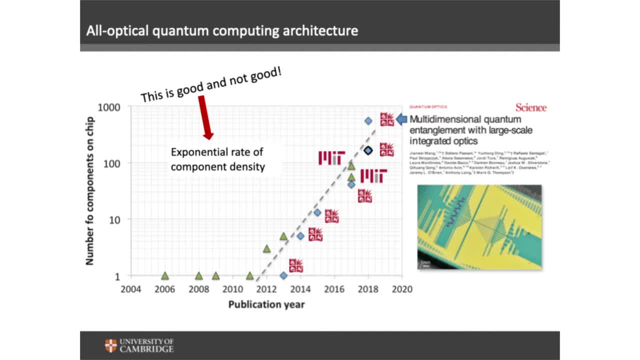 It's good because, hey, if we can increase our complexity of our devices exponentially, that must be good. right, That's progress. It's also not good because we have to increase it exponentially to get to the next level of complexity. The whole point was that we beat exponential need. 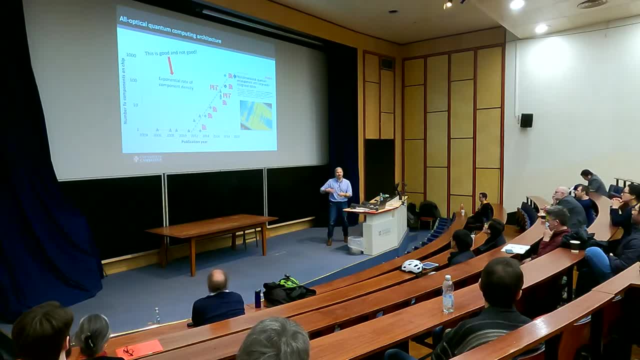 You want exponential ability, but you don't want exponential need. At the moment it looks like to go to the next level, to the next complexity. you do need the exponential growth, So, in a way, the fact that we are able to do it is good. 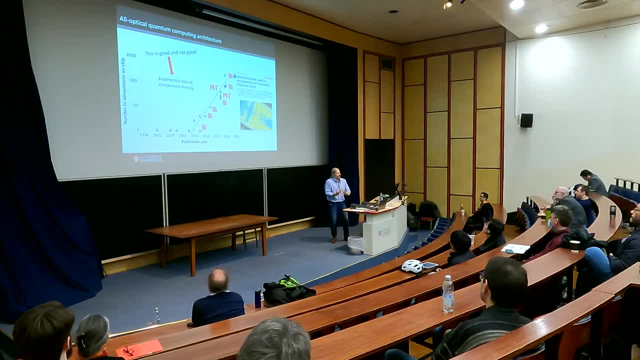 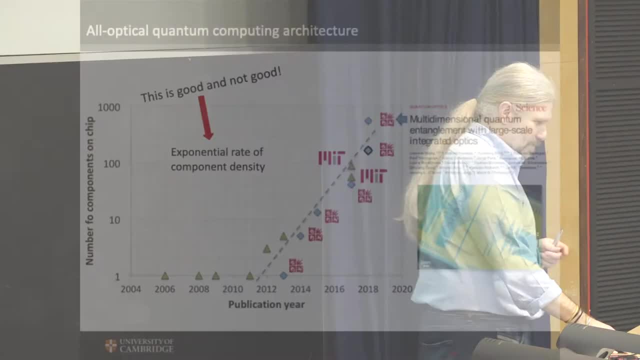 but the fact that it's needed is not good. You want to beat the exponential growth of vanishing, let's say, probability, the exponential growth of the issue of vanishing probability. So how can you fix that? You can sprinkle so one logic, one concept here is: 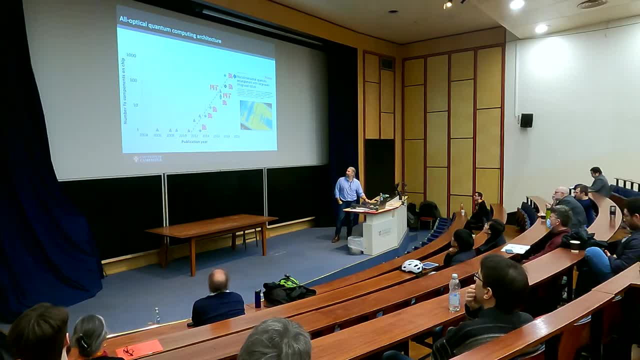 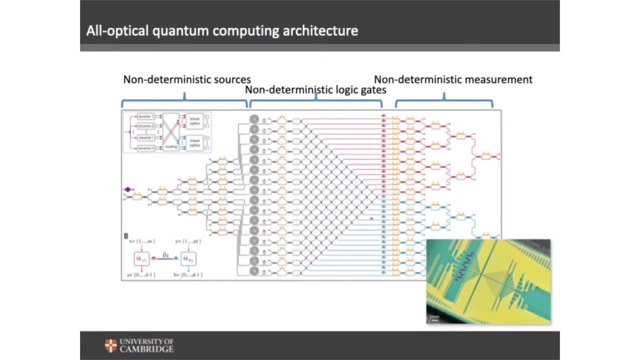 let me go back to the circuit. let me see where is it. There we go. Imagine you take this, This circuit, all probabilistic circuit, and you sprinkle a few deterministic gates in there. If you had, if you had, deterministic gates. 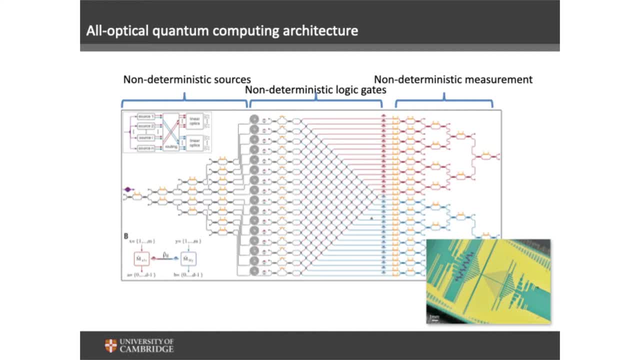 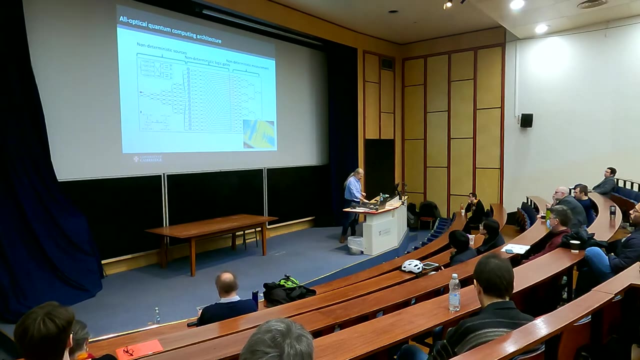 if you sprinkle a few, you are going to beat this pure exponential behavior. So there's advantage in trying to put something that takes light and another light, takes two photons and interacts with them deterministically. if you can Even that, even a fraction of that in that circuit would be helpful. 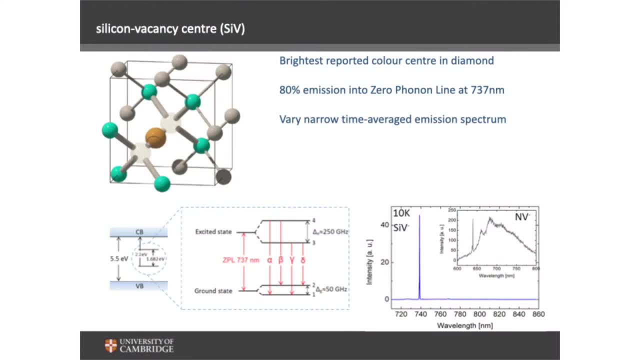 So how can we help with that? Another color center in diamond silicon, the one that gives the yellow, yellow-greenish hue, is actually well-suited for this. It has very sharp optical transitions. when you cool it down It has very good spin spin one-half system. 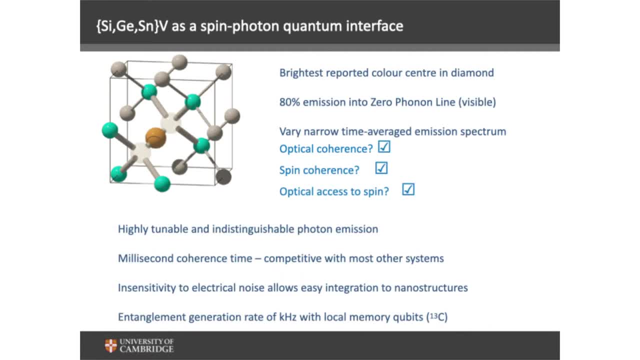 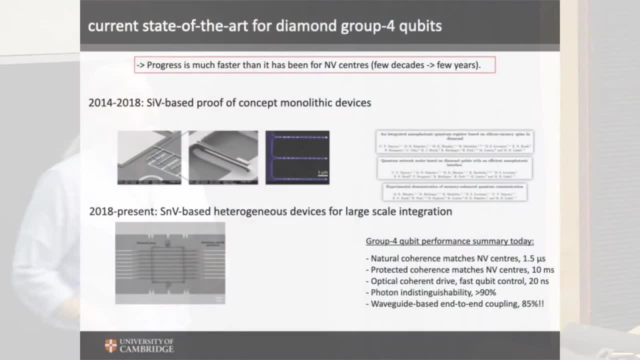 It's integratable, Unlike the NV center. it's better integratable into- let me see if I get this. it's better integratable into nanostructures without suffering from charge surface effects- all the material science complexities that come from actual physical package devices. 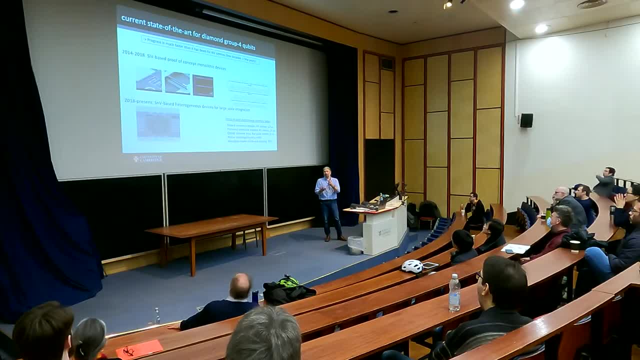 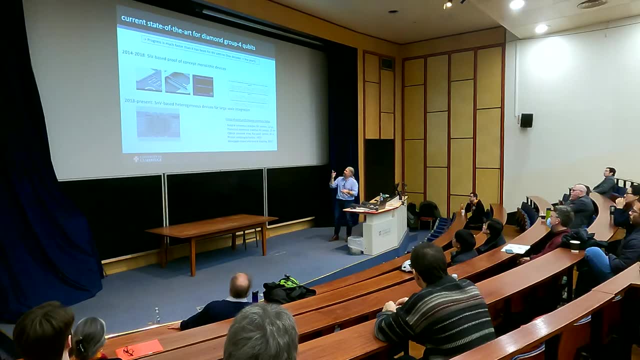 The NV center is good when you leave it alone, but because it has an actual electric dipole, any charge fluctuations disturbs the quality of this quantum object, whereas these, instead of nitrogen vacancy, the silicon vacancy, tin vacancy, germanium vacancy. 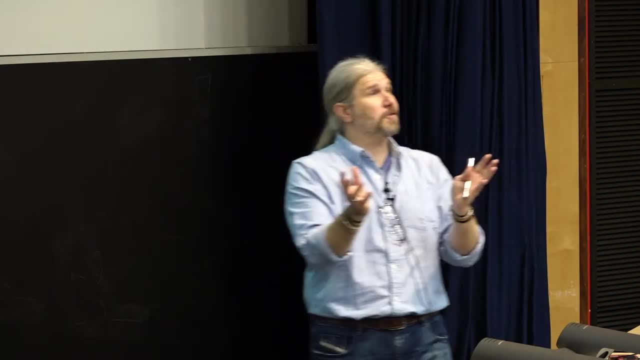 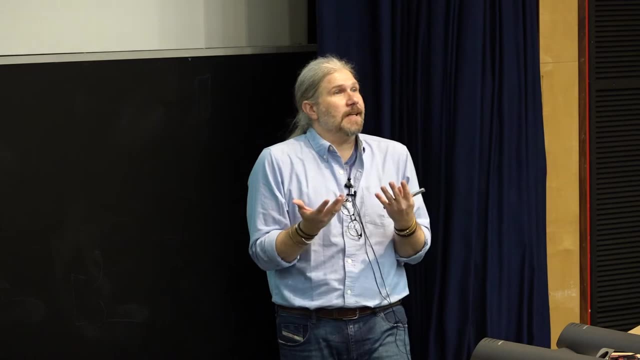 all these group four category in the periodic table. they're centrosymmetric, So it doesn't matter if there's charge fluctuations, It doesn't matter if you have a noisy environment. They're quiet, They don't see it. So they work with just the spin part of the story. 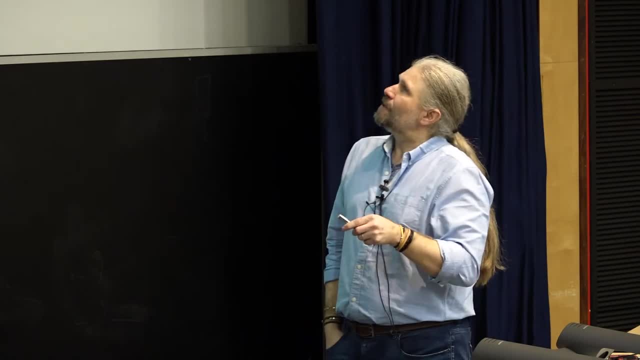 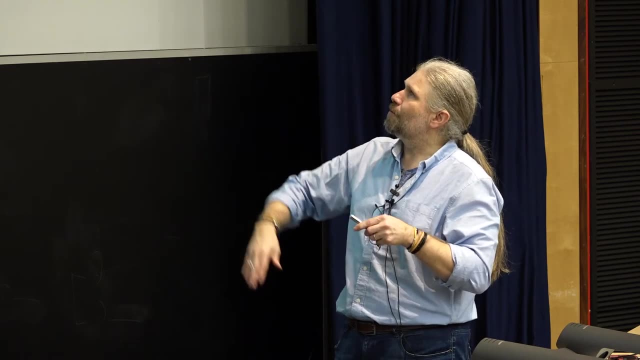 As long as there's no magnetic noise, they're happy. So that means you can actually take these group four color centers and put them in very complicated structures, membranes, or these cantilevers, these little diamond chiplets, for example, is something we're working with. 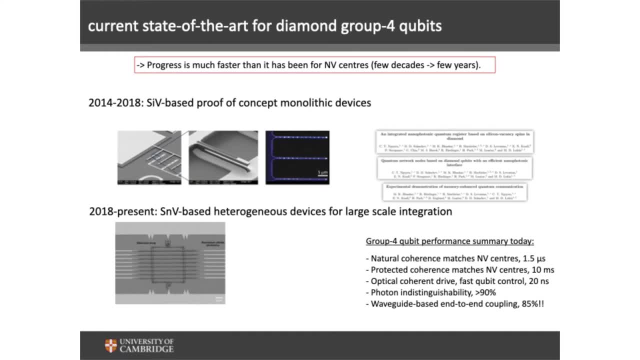 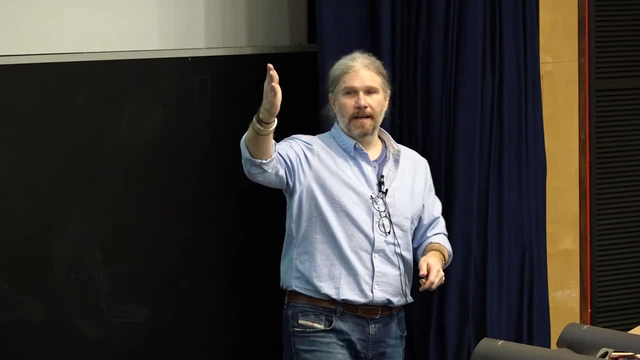 Each one is a wave guide. Each one has a single emitter in the middle, right here, and you can take this whole unit in diamond. You can etch diamond, create this unit, break it off literally and then come back, Come and place it into your fully integrated aluminum nitride. 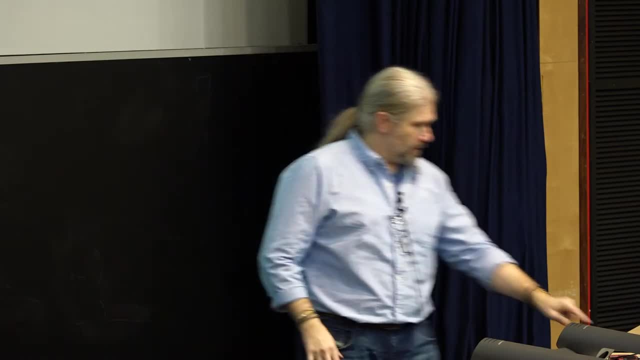 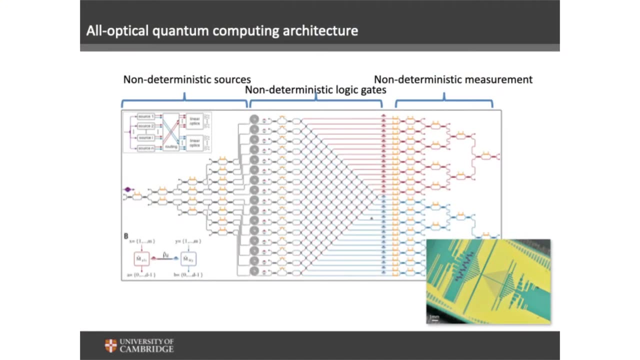 silicon nitride photonic chip, very large photonic chip. So this chip that I have shown here, going back Like that one, You can imagine that if we had, you know how I prepared the framework for it. I said if this could be, for example, randomly selected. 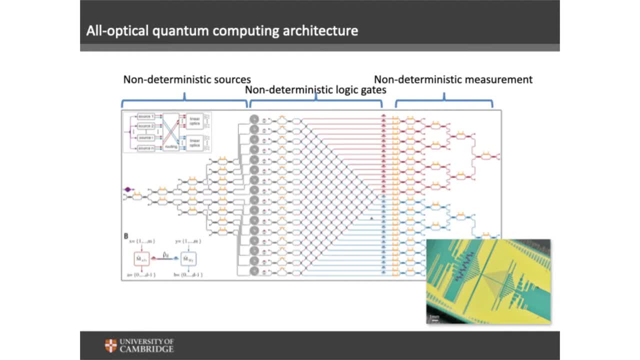 this one could be deterministic How we're going to do that in the circuit. Well, if this one is, for example, randomly selected, this one could be deterministic if you leave that space empty when you're fabricating this whole chip of. 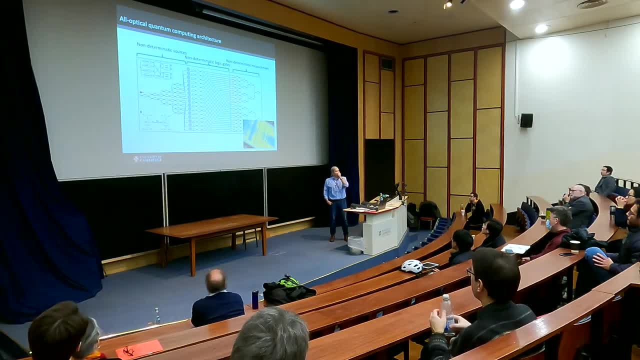 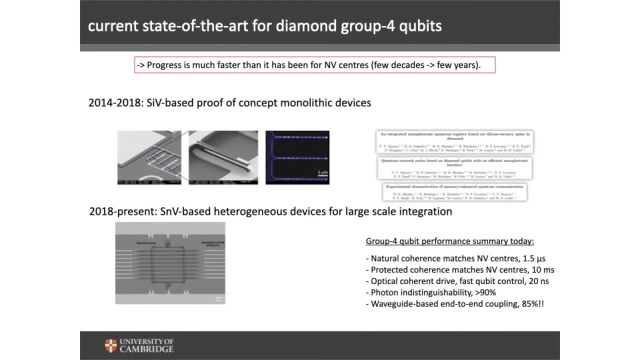 silicon nitride, and you take your diamond chiplet and you just carry it over and plug it in there. I think it was this one. you plug it in there, you have it. So even it determines the quantum object in your otherwise probabilistic circuit to enhance the operation capacity, and that's, that's the concept. 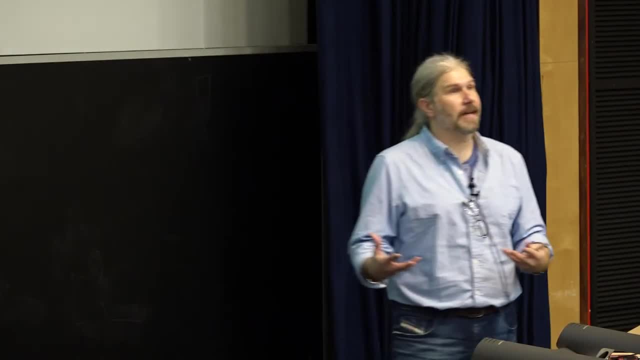 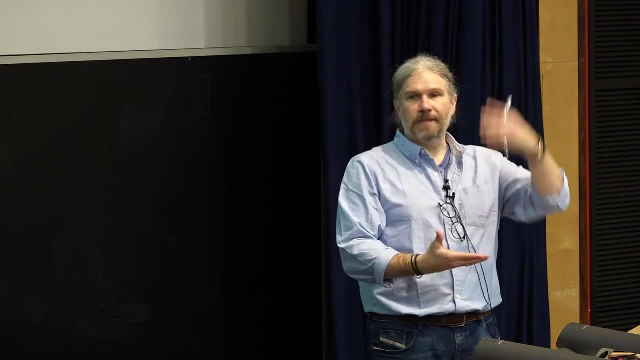 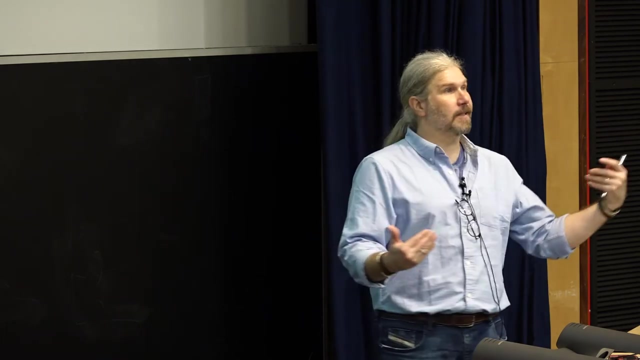 here Again. these chiplets will sit in circuits and they will operate as photon- photon interaction gates. Again, borrowing from a concept in quantum optics, The two level system will all interact with one photon at a time. so if, in the presence of an extention or not, the photon is transmitted or reflected, that's a 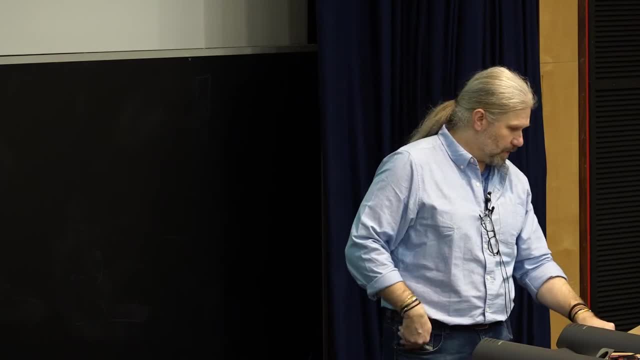 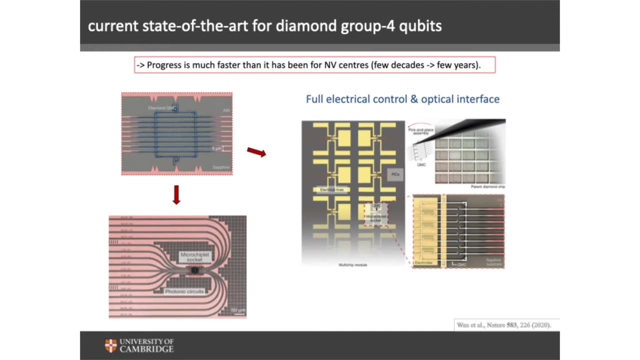 control beam splitter choice effectively and done deterministic. And you can plug these chiplets into microchip sockets, as you can see before here, and the idea is these are waveguides: they come in, interact and come out. these are your deterministic beam splitters or photon. 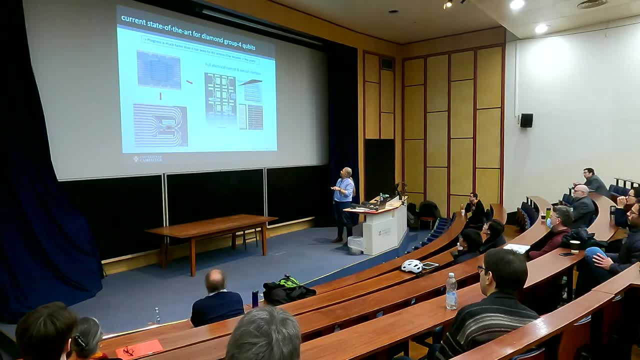 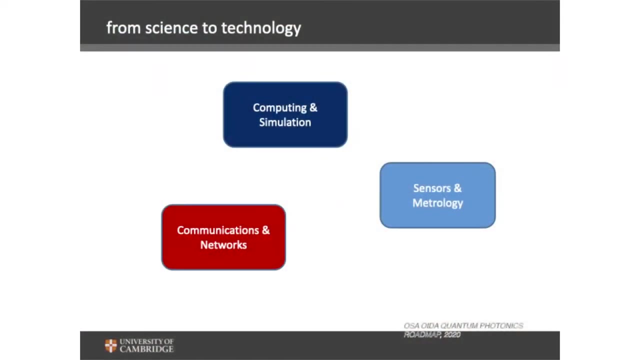 splitter sockets and you can plug them into one. so there's a good, scalable approach to doing this. or you can put this in electrical circuits and control, spin and link it to current. Alright, so the future is, let's say, bright for for diamond for that purpose. and now I want to come back to this guy, the third one. 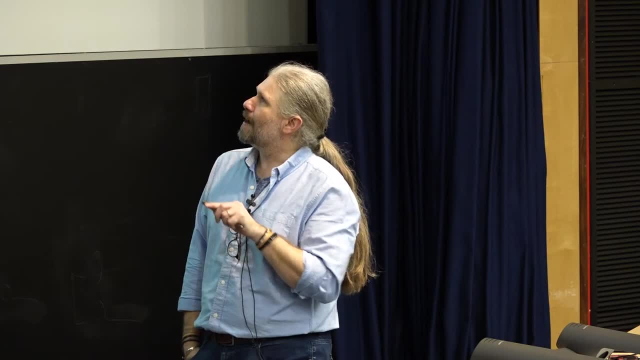 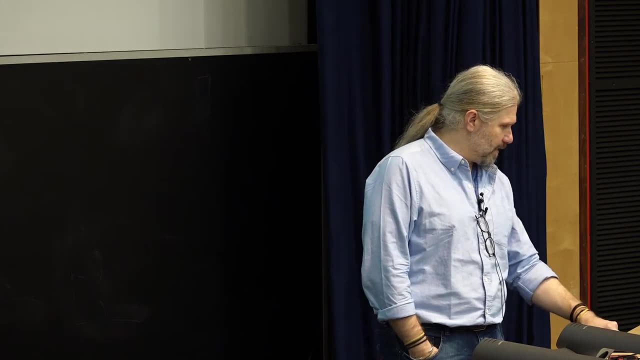 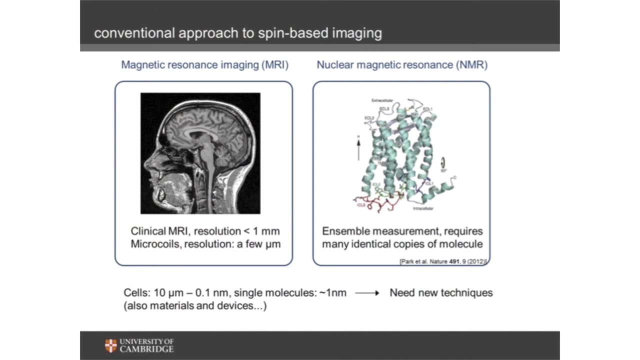 we talked about computing. we just talked about where there could be an impact on the computing side. there's the impact on the networking side, and diamond could be a significant impact on the networking side. So a few words on on that. so what, what could be attractive on the sensing side? well, the ground state is a spin. 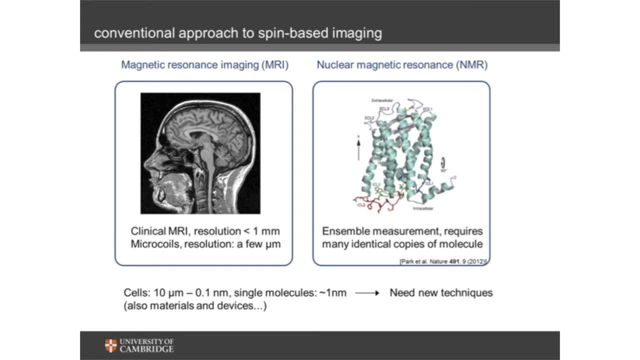 right, it's a spin active molecule in nature. it's not easy to find these things in nature. when you talk about single molecules or other things, the ground state is usually a singlet. it's a nice isolated singlet. spin active states are usually higher in energy, with a finite lifetime before they decay. to this: 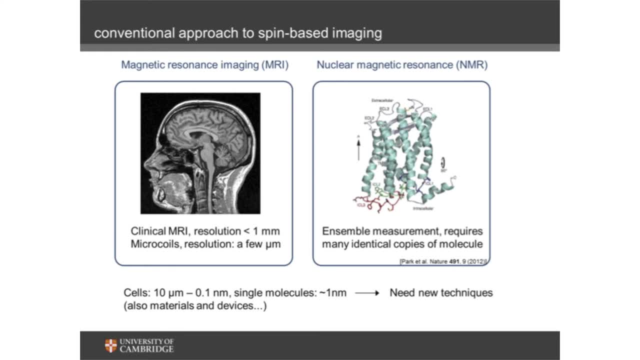 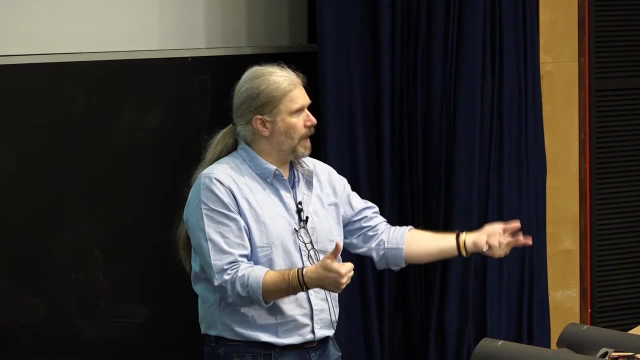 stable spinless ground state center. NV center in diamond is one of those rare cases where the ground state is spin active. So there is an active spin sitting there exploring the magnetic field. That's why we can talk to it. All the tools of quantum optics in lasers, microwaves, radio waves- to access these spins. 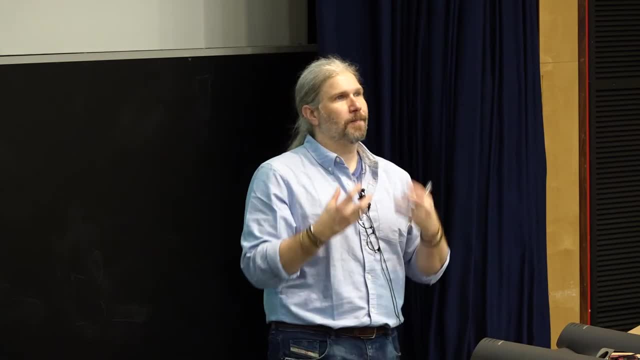 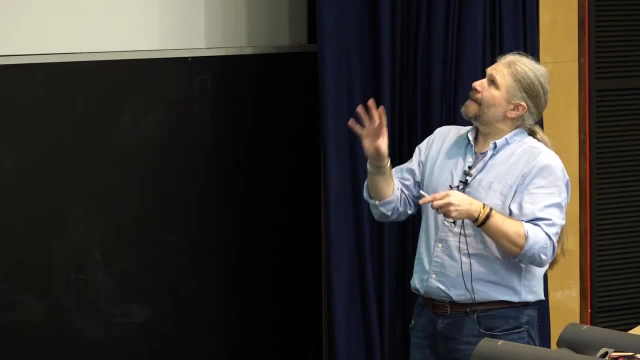 and going back to the old books of NMR to pick up protocols, develop protocols to understand things better and how to operate with spins. It's all in there. And what area that the spin, this access- optical access to spin- can have impact on is spin-based imaging. 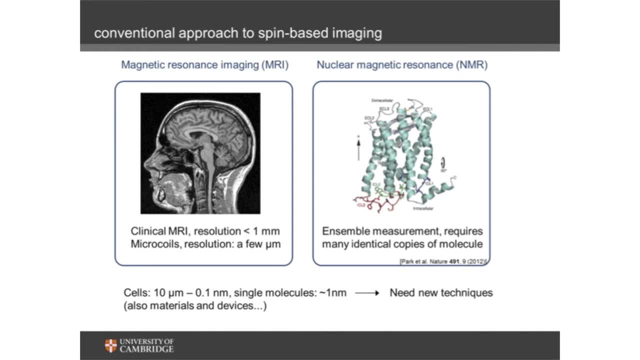 So here the MRI- magnetic resonance imaging- or NMR, nuclear magnetic resonance. they're the same things. For those who may not have noticed, they're exactly the same things. It's just that public doesn't like the word nuclear. So instead of nuclear magnetic resonance, you do that in your 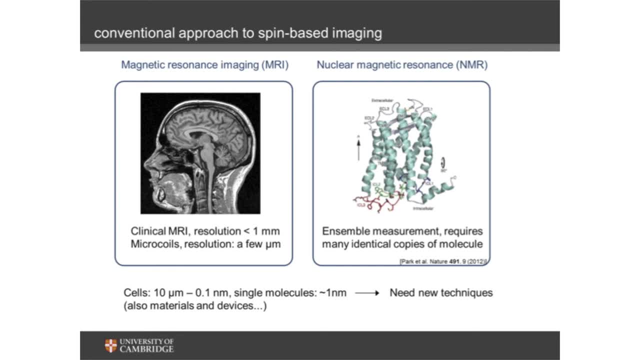 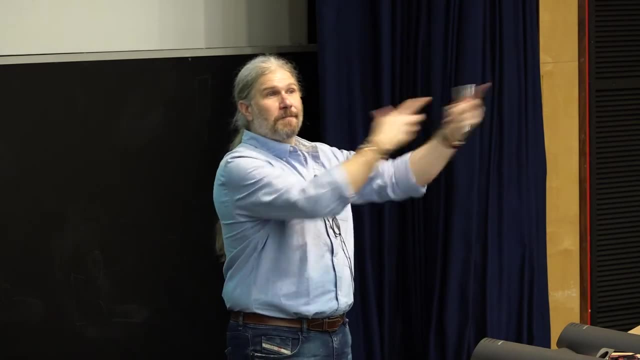 lab for research, and when you're ready to translate it to healthcare, it becomes nuclear- magnetic resonance- and you swallow the word nuclear there. But it is nuclear Because- not because there's anything radioactive, but because the protons, the nuclei, are processing a magnetic field. They process and generate a magnetic field themselves because they're. 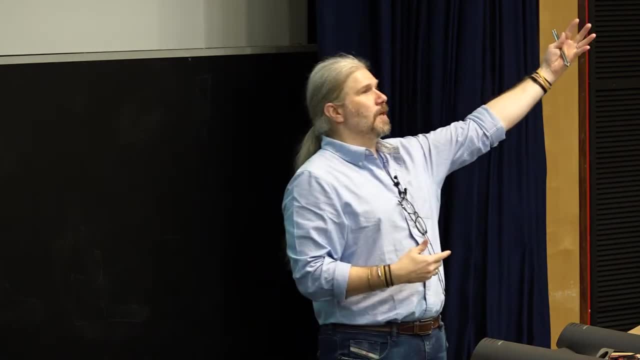 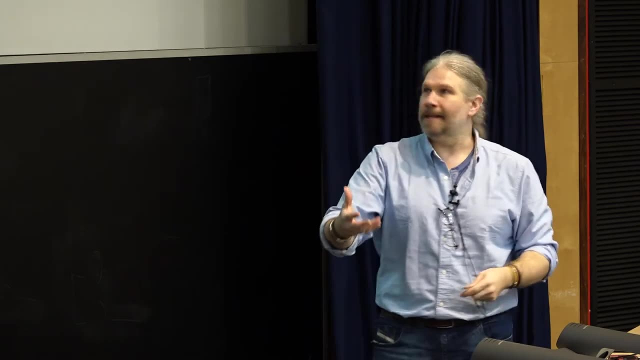 processing at a certain frequency- precision frequency- and you pick it up with a coil on the side. So you check how many protons are around and where they are And from that you can deduce what material is in there. And actually that's pretty impressive. They can build up a whole image based 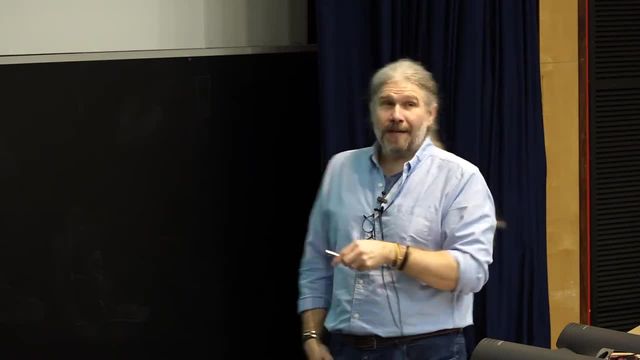 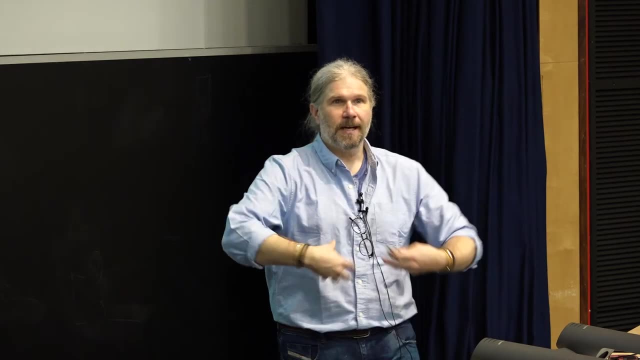 on where your coil is looking. The good thing about that is we can actually see inside us by the signal actually coming from us, not externally. We don't do something to us. It's the natural response of our body and that's fantastic. The downside is we have a resolution of about a millimeter, because the integration volume you need to develop enough signal to detect is set by how insensitive your nuclear spins are. Tiny Nuclear spins are thousandth of that of an electron, So that's why it makes it hard to actually detect. That maps your detection volume, the smallest volume you can detect. 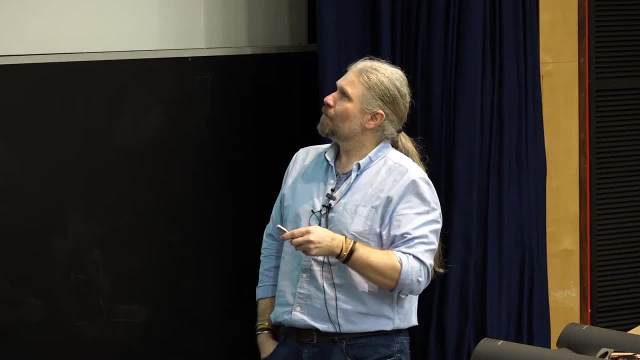 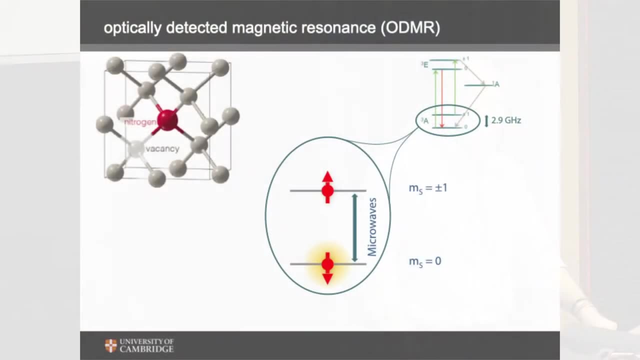 So you want to make this smaller and smaller, to be able to see finer and finer. That's what we'd like to do, And there are many attempts. What I'll do is I'll highlight how diamond could come in handy with this. So let's take a look at those ground states that I didn't really talk about much. 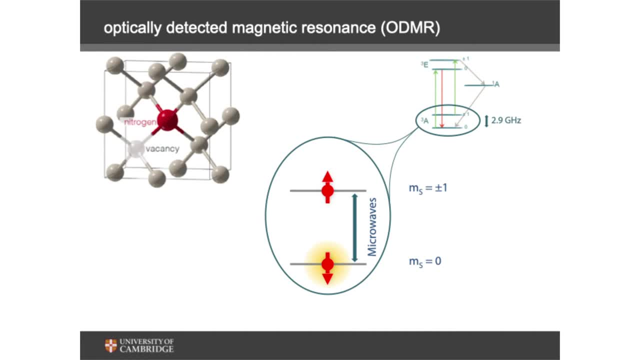 This was the optical transitions of the NV center in diamond, If I look over here closely. I said 2.9 gigahertz split. This is what it looks like. There's one spin state. There's another spin state. In reality, this is 2.9 gigahertz split. This is what it looks like. This is one spin state. This is another spin state. In reality, this is. 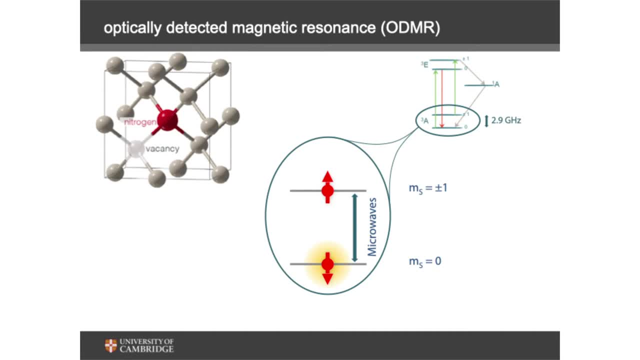 a spin triplet. So this is the ms equals zero triplet. This is the ms equals plus and minus one part of the triplet. So it's a degenerate two levels And you can imagine that if I apply a magnetic field, the plus one is going to go up, The minus one is going to come down. So it's going. 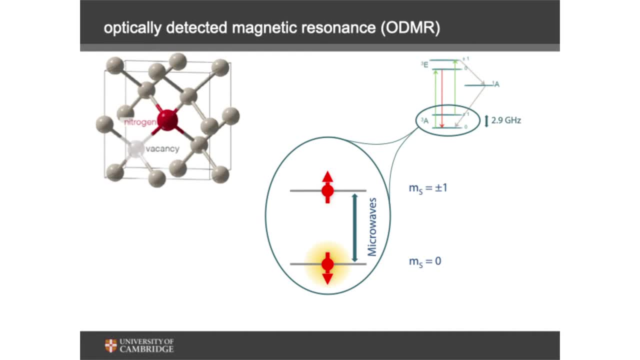 to be a three level system, But given that we have optical transitions, we can actually probe the fraction of the ms zero state versus ms plus and minus one states optically. I can actually record that optically. I can actually record that optically. I can actually record that optically. 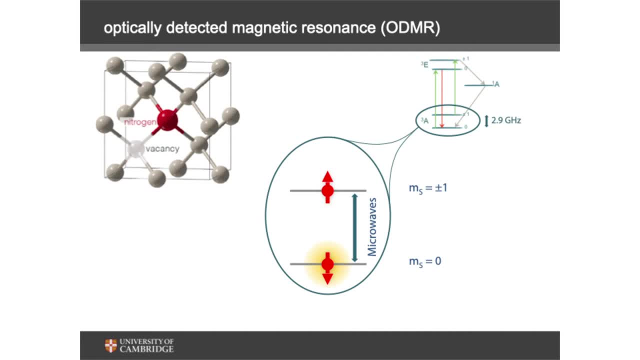 That's why we have a quantum network, because we can read out the spin state of our qubit efficiently. If that's the case, I can use the same thing to say: OK, if I pass a microwave, I'm doing pure quantum optics now in the good old quantum optics, the way it was done. 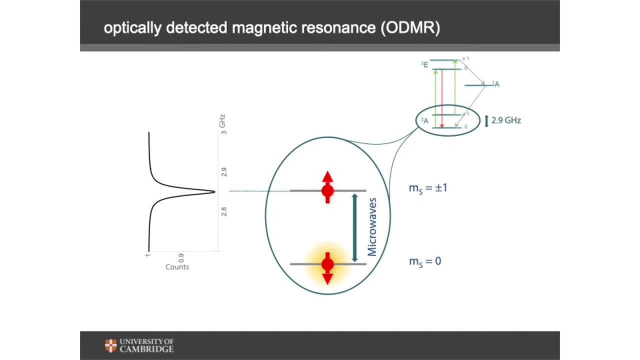 Even pre-lasers, by the way, when people identified the spin nature of atoms, that's another Nobel Prize. So quantum optics has received attention. So as you sweep microwaves, when you hit the right frequency, you're distributing the population. 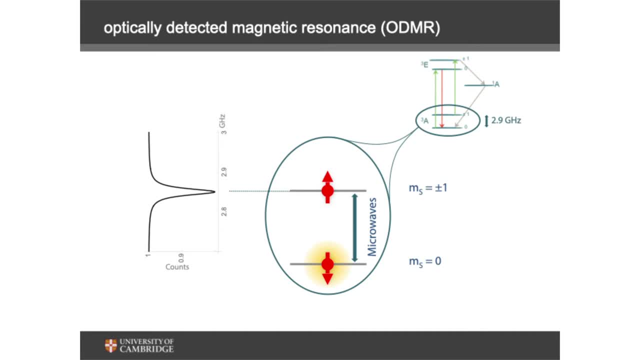 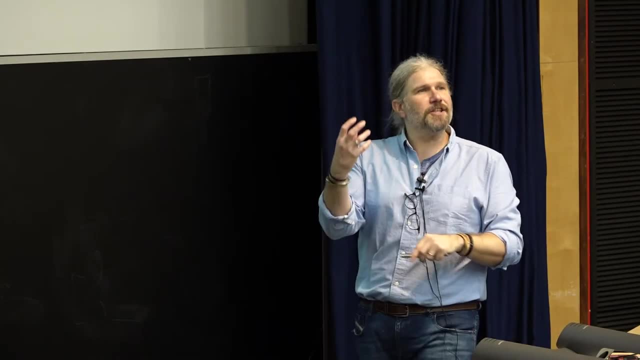 here You're shuffling the population. If you shuffle the population, the intensity of light that you see from the nitrogen vacancy center drops and comes back or it's altered. That alteration, when you actually actively externally disturb that spin population, is a signature of. 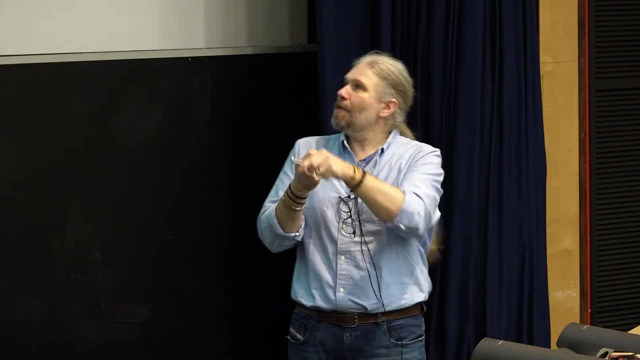 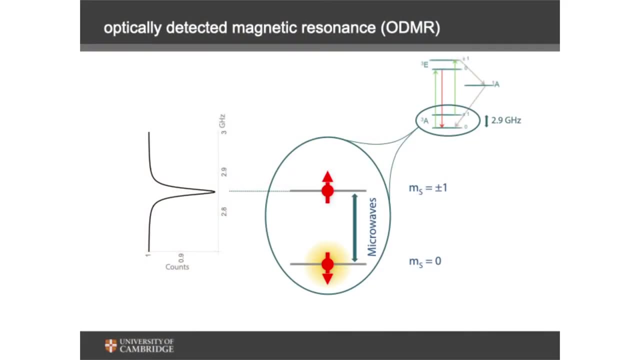 where that transition is in microwaves. So my accuracy is not even the optics anymore, it's the quality of my microwave frequency, frequency I'm sending, which could be subhertz right. So I have very high precision of telling where that transition, that splitting, is. So if there is a magnetic field, 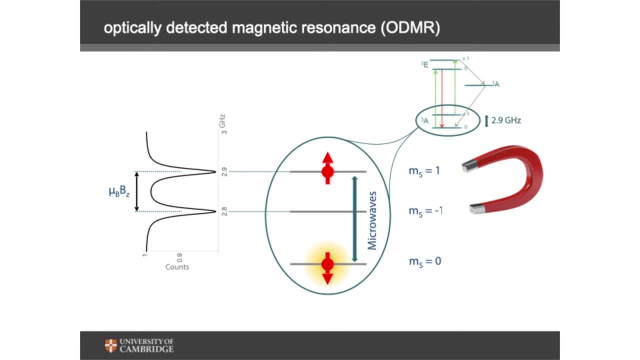 ambient magnetic field. what's going to happen is that, as I said before, the MS plus one state shoots up a bit. MS minus one, I'm done What happened to the one here? MS minus one state goes down a bit, So that resonance that I had in the middle right here is now turned into a doublet. 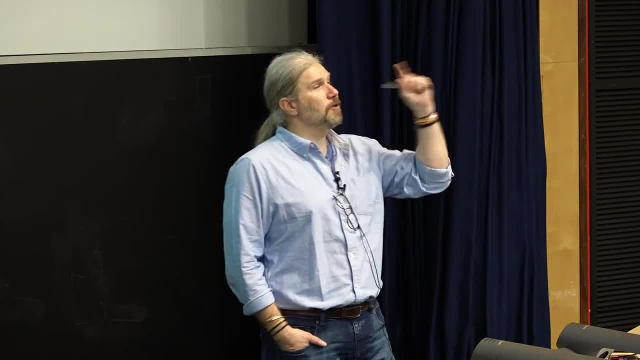 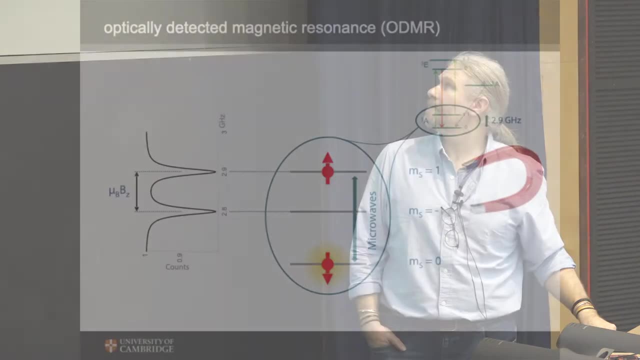 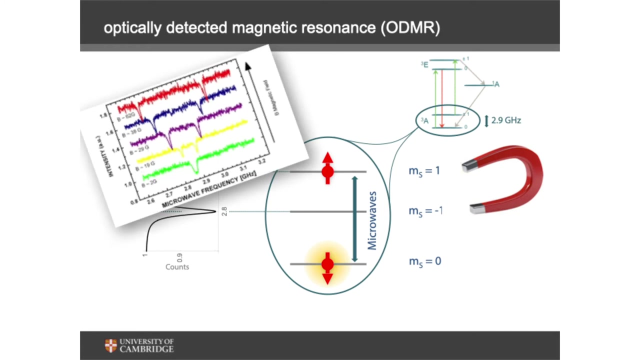 Okay, So from the splitting of the doublet I know the magnetic field that the NV sees. Great, Let's see. So here's an undergraduate lab demo of the NV center measuring magnetic fields As you apply Gauss in units of Gauss, meaning small. that's what I'm going to say, If you're. 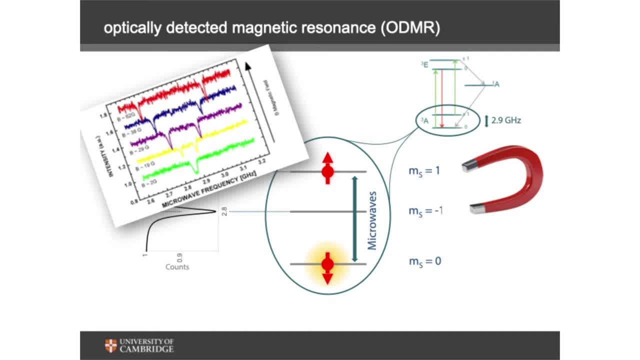 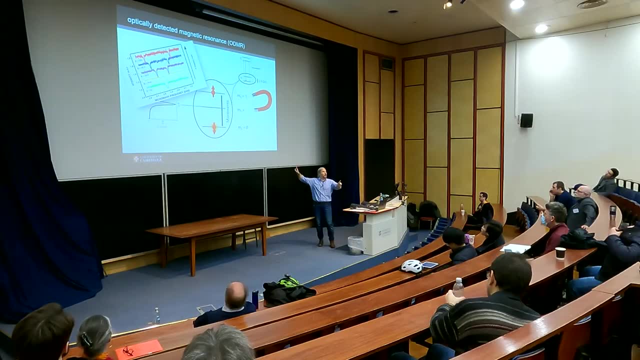 using units of Gauss, that means you're measuring a very small magnetic field, And what you're seeing is that you're measuring a very small magnetic field And what you're seeing is that this state is splitting up into more and more split doublets as you apply more and more field. 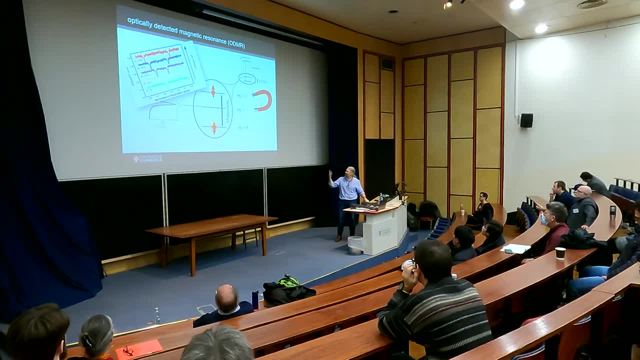 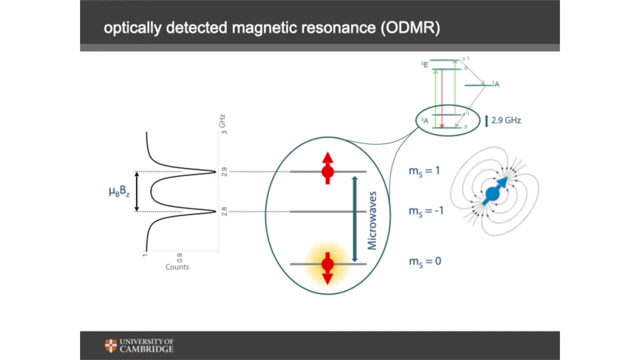 to the NV center. Okay, So it's a direct measurement. You can actually see this. So how can I use this? That magnetic field need not be coming from an external field we apply. It might be a nearby spin. So if I want to detect the presence of a spin that isn't coupled to 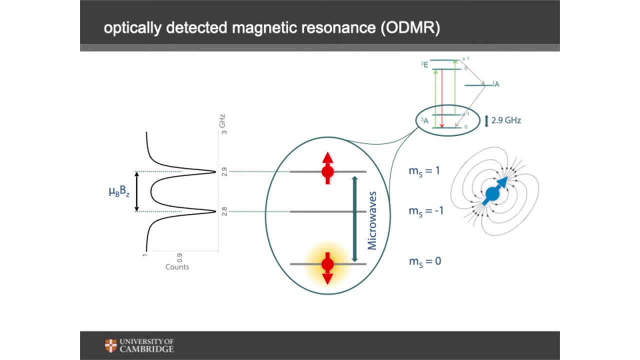 light. what am I going to do? I can't use MRI or NMR because the signal is not going to be not strong enough, but I can bring an NV center nearby and it's magnetic field of this one spin will split. to what extent I don't know, but it will split this transition and I should be able. 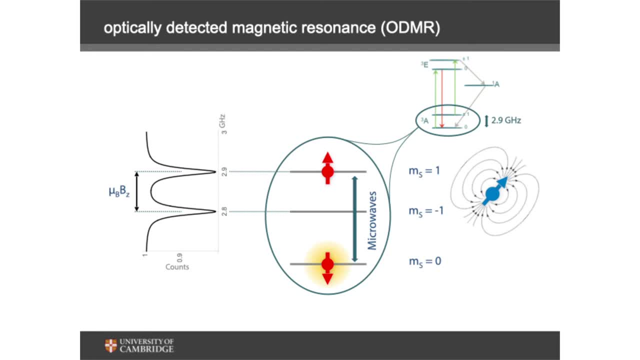 to detect down to single spins. Okay, Magnetic field down to a single spin, And it turns out that even light, even heat, is something detectable. So you can talk about nanothermometry with NV centers, but that's just to keep in mind that there's multiple modalities for this. 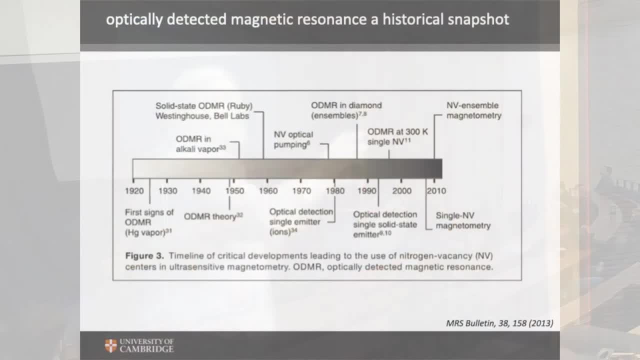 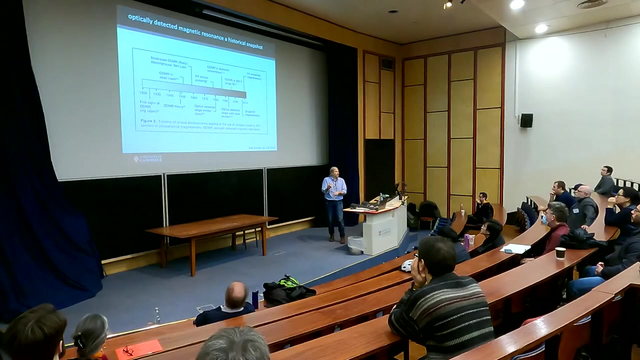 So this is called optically detected magnetic resonance. So it's not magnetic resonance. imaging the way we did it, using the signal from the spins processing together in a finite field, but rather optically reading out what your NV center tells you or what your physical system tells you. And it actually goes all the way to 1920s with mercury. 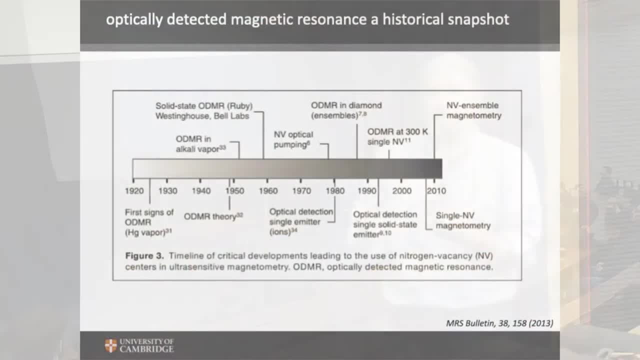 vapor. So it's again atomic physics, optics and atomic physics combined together to give us first applications of optically detected magnetic resonance, internal degrees of freedom, And it goes somewhere. here is the optical detection of: So this is the single emitter, this is the ions. right 1980s, That's where, first time, we actually 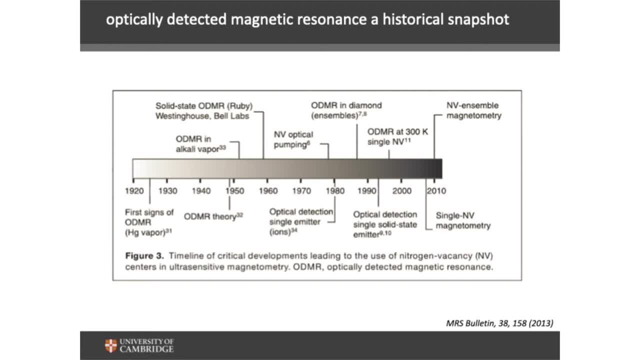 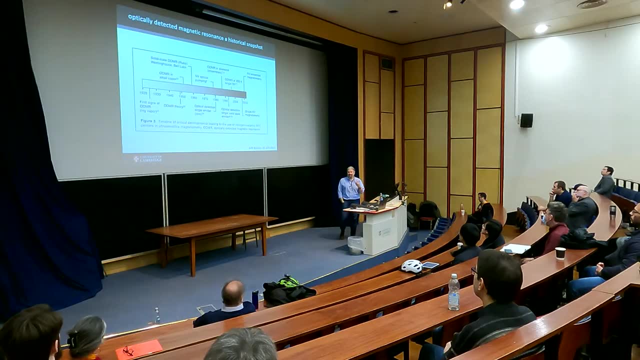 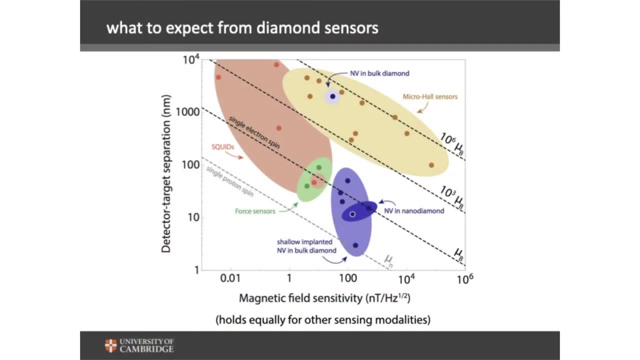 see single quantum objects And NV magnetometry. nitrogen vacancy centered magnetometry is literally in the last 10 years. It's amazing. this has been 10 years already, but it's only been around for about 10 years or so. How does it perform now? This is a nice map. I like this map. it's magnetic. 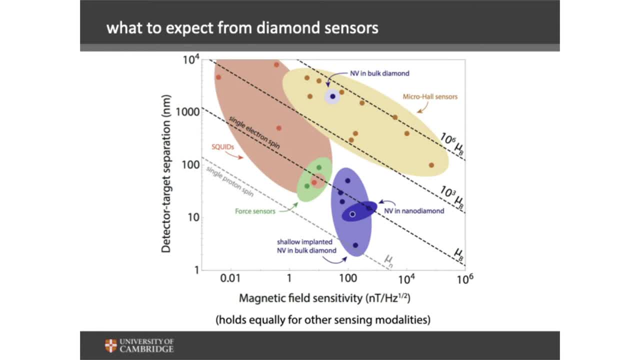 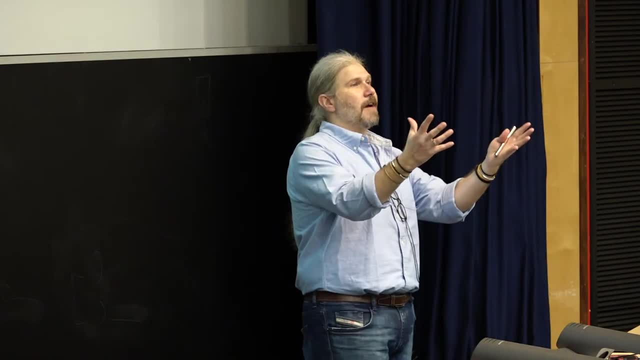 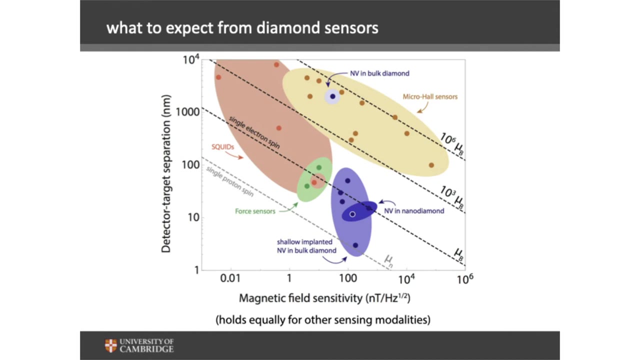 field sensitivity. How sensitive are you to a strength of a magnetic field that you're seeing, you're exposing the NV to, And this is the characteristic size? How big of an area do you need to integrate to get that signal? Or how far are you from the source? essentially- And there are many, many different- 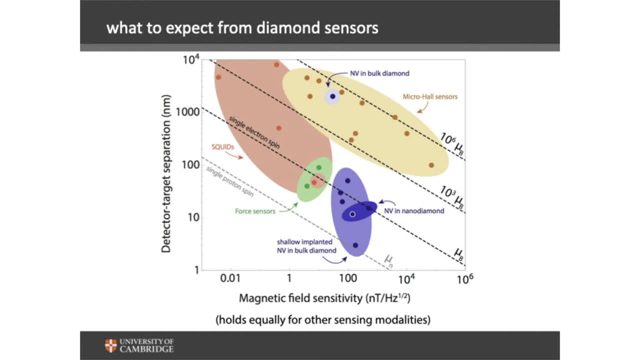 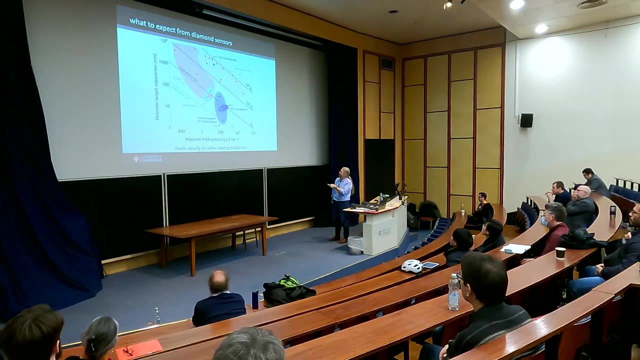 micro hole sensors, the single electron spin- these are squids- force sensors. there are many different approaches to it. This is the typical NV performance area, So it's not the best in terms of sensitivity by measure of the value here. magnetic fields and nanotech. 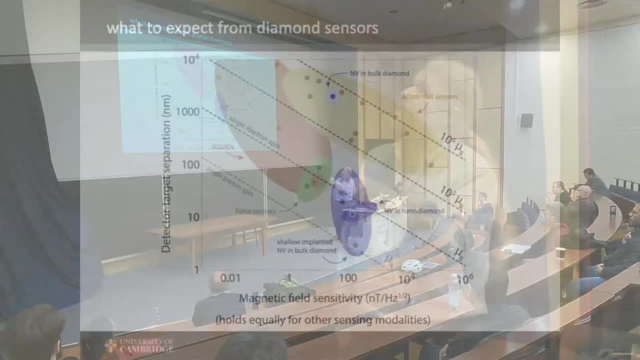 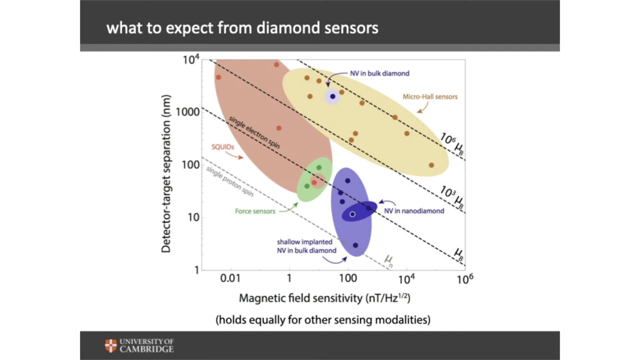 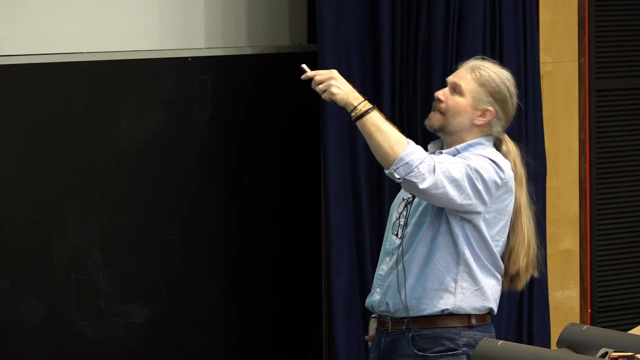 Tesla per root hertz, But it is actually one of the closest things you can be to an object that you're trying to detect. The diagonal lines are informative. This line is the compromise of distance versus field sensitivity required. This line is 1 million electron spins, If you wanted. 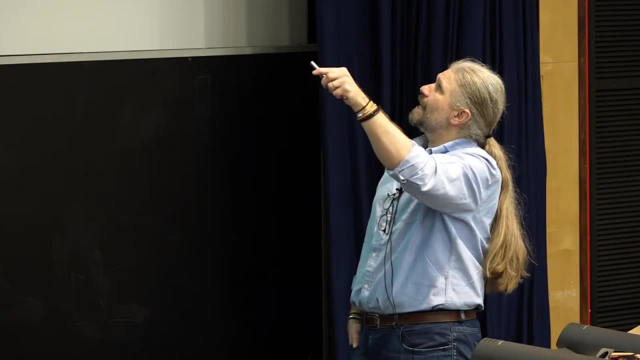 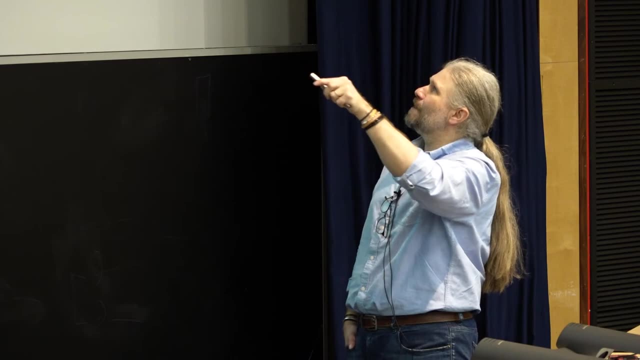 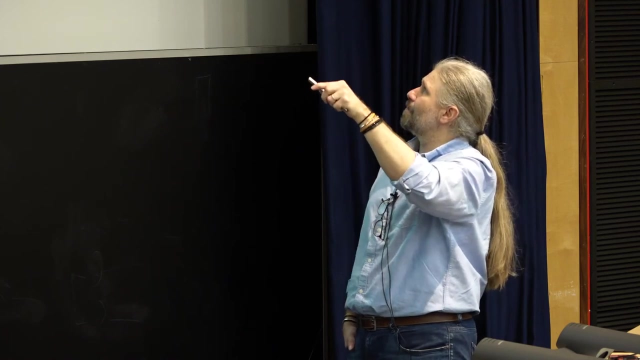 to detect signal from 1 million electron spins. this line is all you care about, So you're here and you're safe. If you want 1000 electron spins, signal correspond to 1000- you need to drop down to this level of sensitivity or detect the target separation. This is one electron, If you wanted. 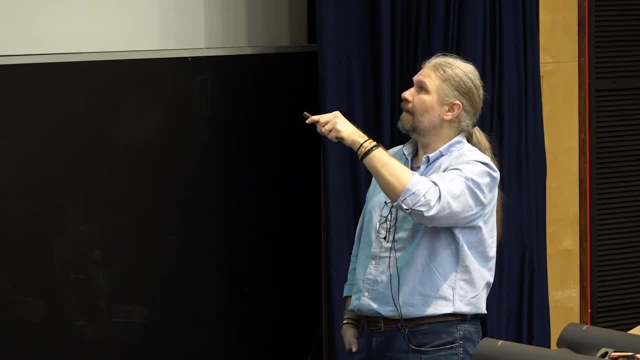 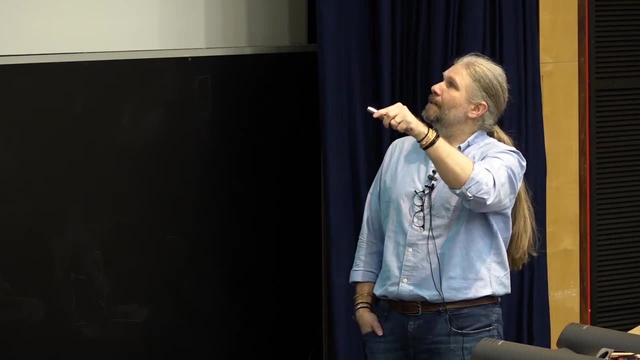 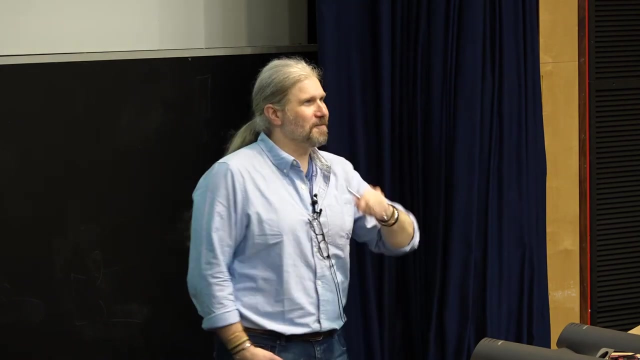 to detect a single electron. that's where you need to be If you want to detect a single proton. so if you want to do single proton MRI, that's your line And the only thing that kind of rests there is the NV It's just about. It's not comfortable to say we can detect, you know. 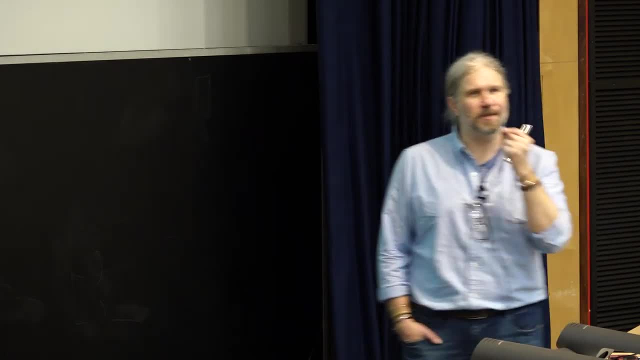 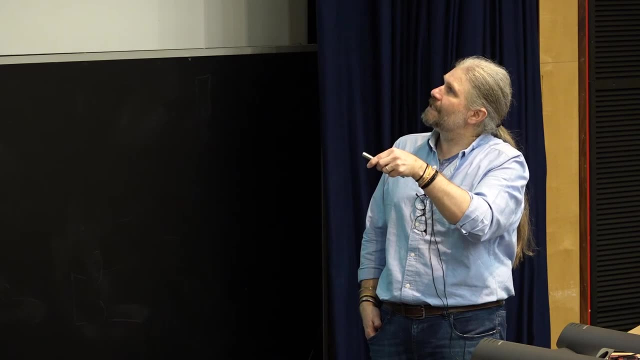 with high signal noise. but it is there, So it has the precision to be able to do this. And this has to do with, again, the interfacing question: How close can we come? Look, the reason we're touching this line is not because the NV center is very sensitive. 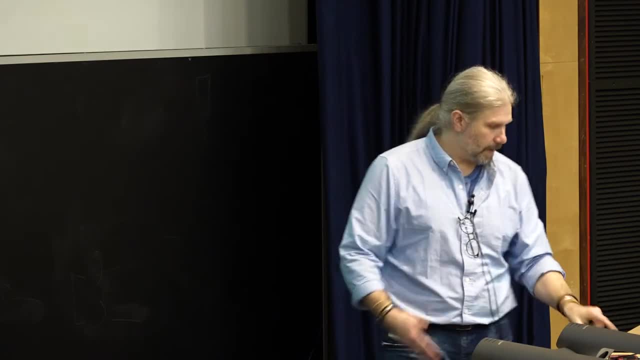 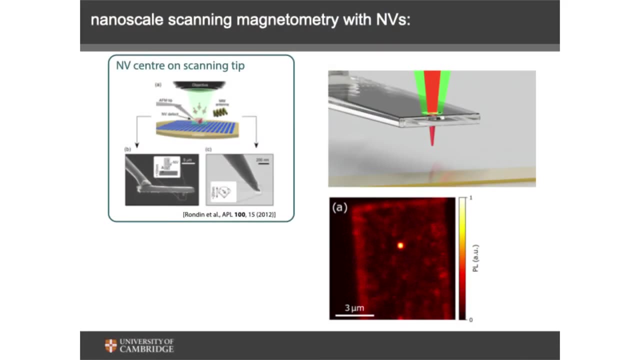 but because it can be very small, It can come to a very small contact. All right, So here's one example of how NV centers are used. This is a cantilever, just like an atomic force microscope, But instead of topological bend as. 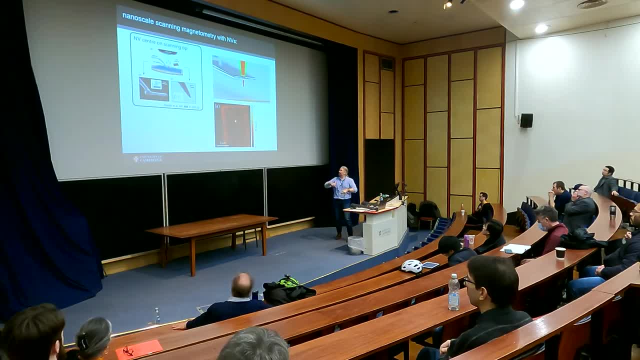 you go over objects and measuring the deflection of your atomic force microscope. you have a tiny little NV center in this diamond film And you look from the top. When you look from the top, this is how it looks. It's bright, It's like a single trapped ion. It's nature's trapped ion. 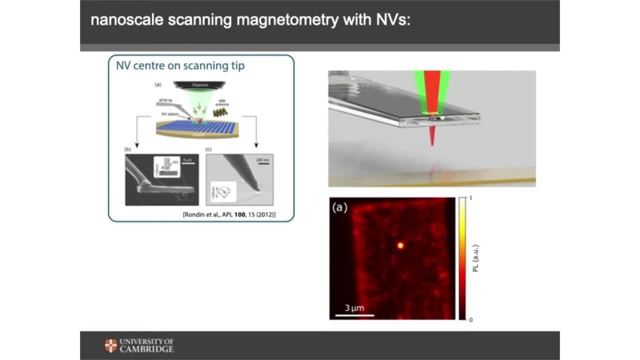 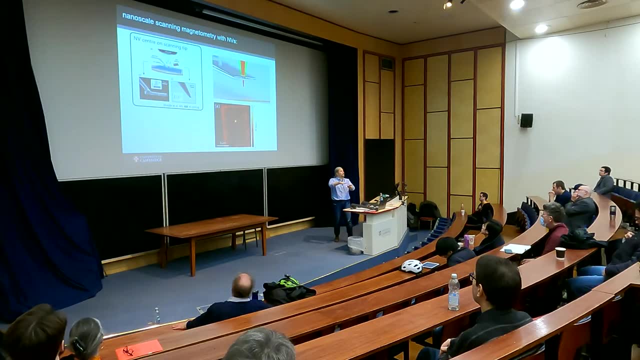 It's trapped in diamond with no other elements required to keep it in place. It's always there, always active, And you have this cantilever And you just scan over a surface and you get magnetic image coming from that material underneath And it can be as close as 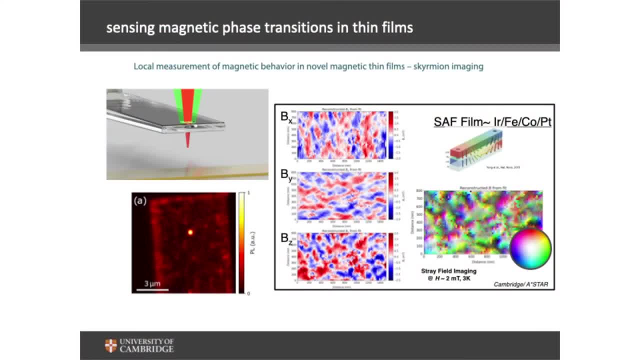 you know, a few tens of nanometers essentially- And that's an example image- You can actually get a full vectorial map of the field on top of a magnetic material and you're imaging the stray field vectorially. That's the nice thing about the NV center: You can actually 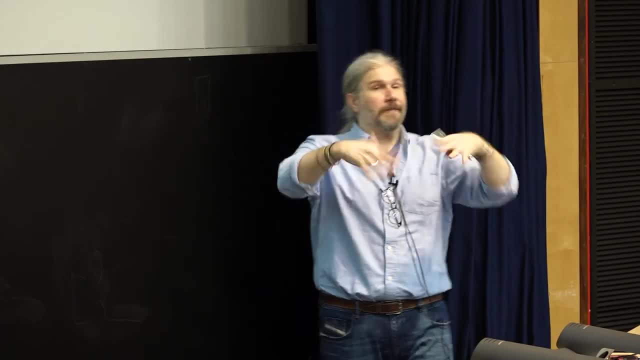 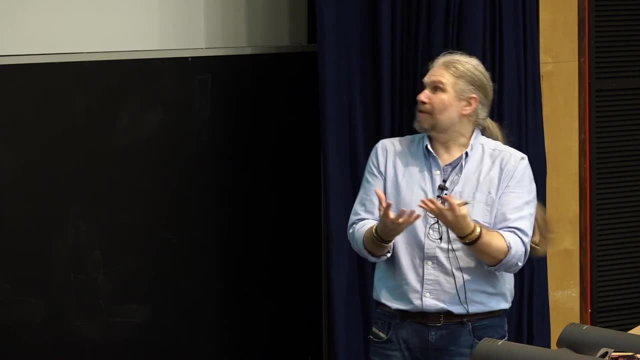 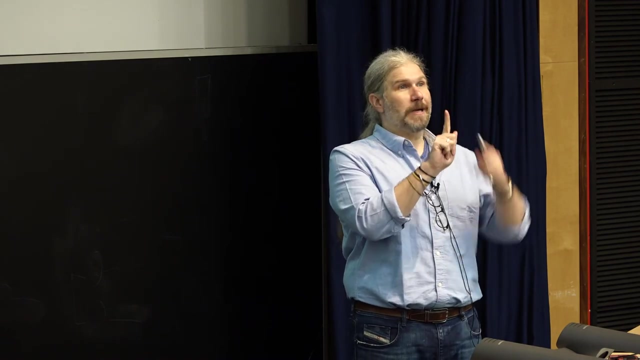 get a full vectorial map of the field on top of a magnetic material, Even if it's antiferromagnetic. in fact, you can capture the spin texture underneath and understand at the nanoscale. And the biggest wins in this is that your measurement device is a single electron spin. 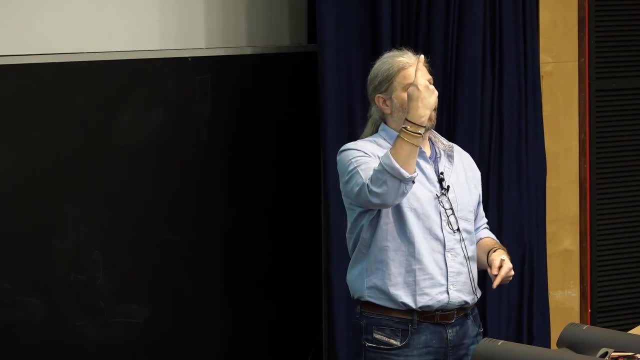 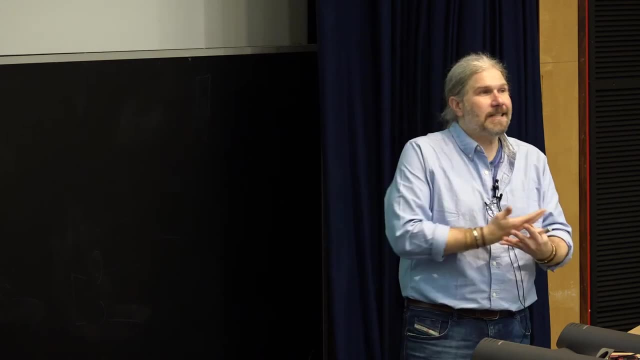 So the back action to the material you're measuring is on the order of one electron. What you're measuring is probably hundreds of electrons equivalent. So the back action is removed. So it's a nice clean, undisturbed image you can get, as opposed to magnetic force imaging. 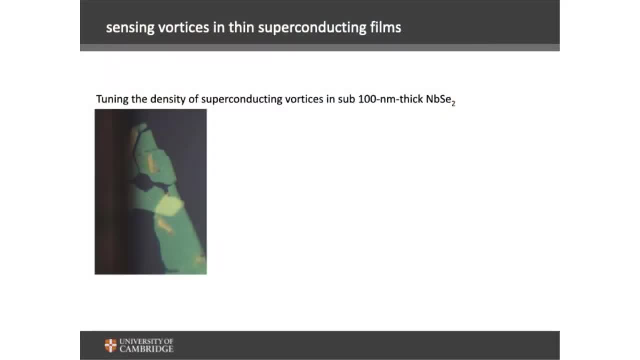 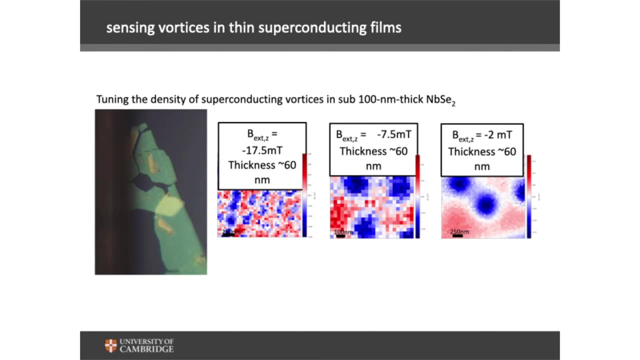 for example, And here is a superconducting material, thin film, very thin superconducting material, And if you look at again, if you do the same experiment on this material under different conditions, you can actually resolve vortices opening up. 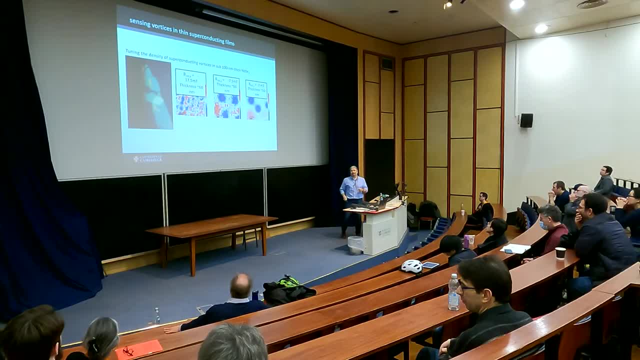 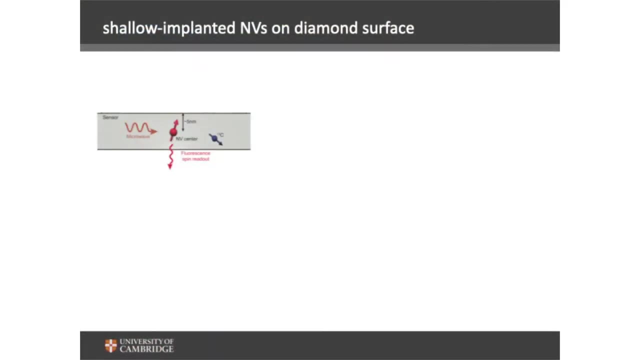 Superconducting vortices opening up in the field in this otherwise superconductor. So it's very nice. You can actually capture these spin textures or magnetic phenomena in nanoscale using these systems. And I'll show one more thing. Let's see how am I doing with time. Good. 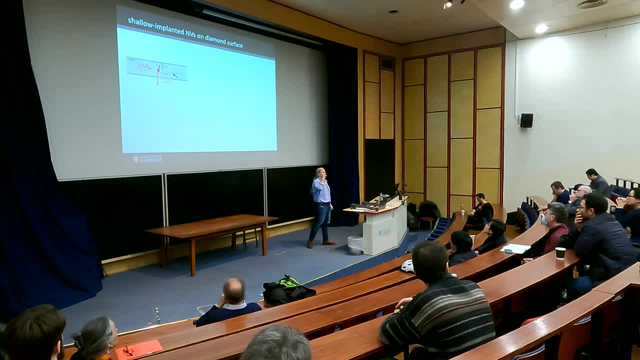 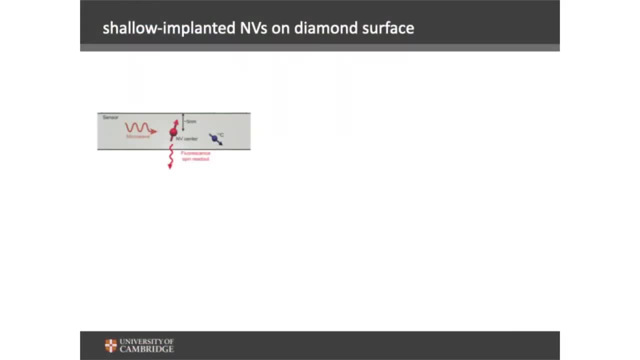 So instead of a tip you can also say: I don't want to bring my detector to the object, I like to bring the object to my detector For that one. this is also another modality of measurement. with NV centers You place them very close to the surface on the. 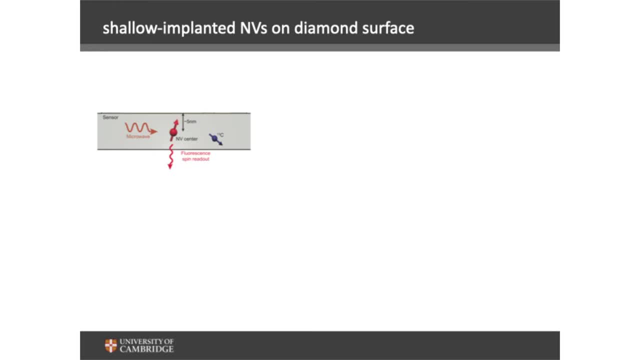 order of five nanometers. And then you say, OK, I'm ready, Let's put something on it And let's measure that something. Now the interaction. this is the funny thing about the NV centers: it measures in a dipolar fashion, So it will measure what's up here, but it's not going to. 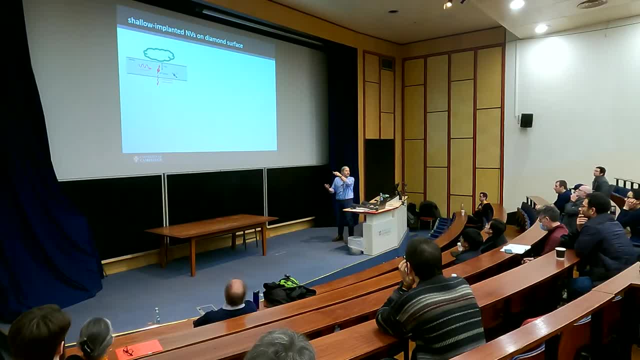 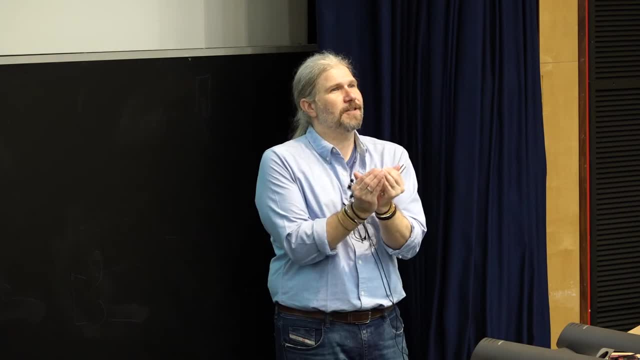 measure what's up there of the same species, because it's too far off. If it's too far, the signal is vanishingly small, so the NV center won't detect it. So it is a naturally small integration volume for detection. And what people have done, particularly Harvard, 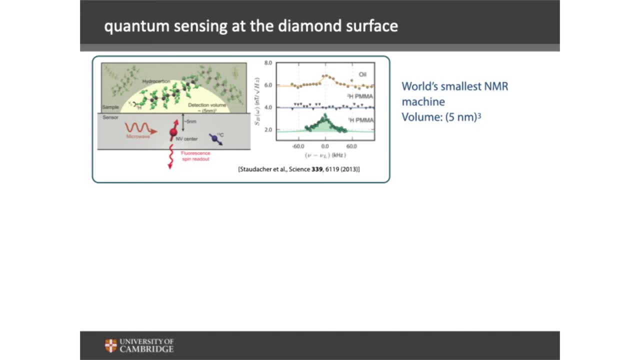 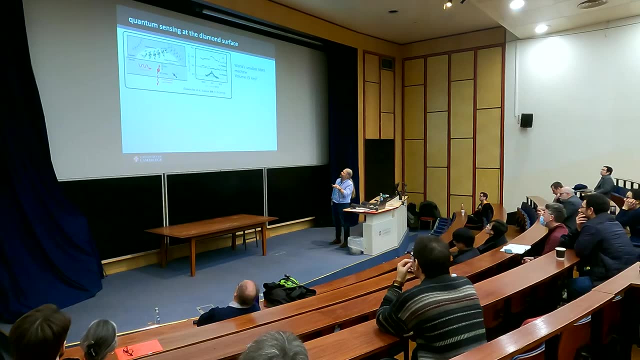 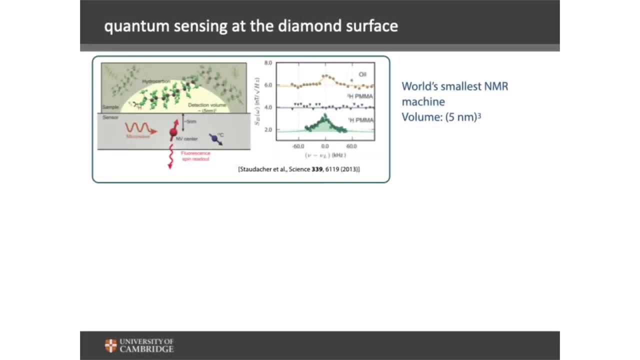 is demonstrate that if you put a solution, a complex solution, on top of a diamond surface with very shallow implanted NV centers engineered around five nanometers, you can actually detect the spin of hydrocarbon chains as they land on top of your NV center. And this is 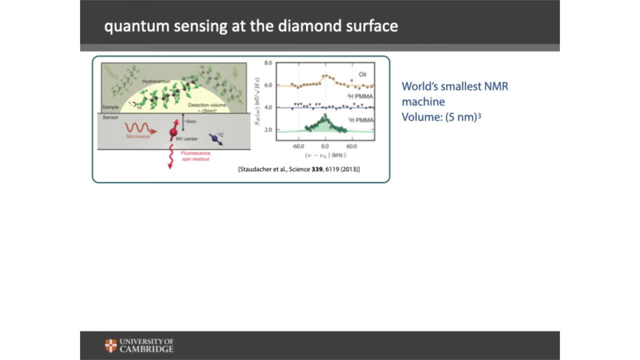 what you're seeing here. This is from 1913.. You're seeing a five nanometer cube volume, world's smallest NMR machine, where you're measuring different species: oil, PMMA, hydrogen atoms and all that. So this is MRI with a five nanometer characteristic length scale. 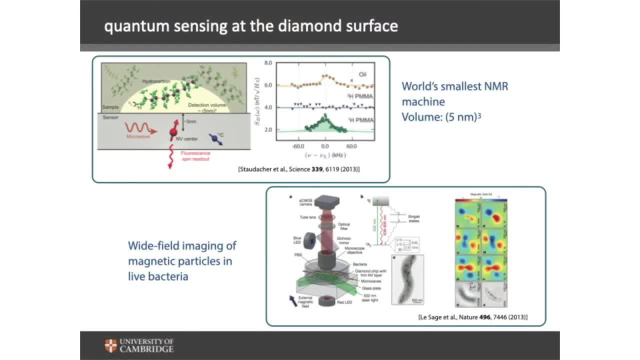 And of course you can take it much larger. So that's single NV talking to a very small thing, but it can have an ensemble of these NV centers And you can look at macro things like these worms, live bacteria that actually eat iron. So they eat things and they produce iron. 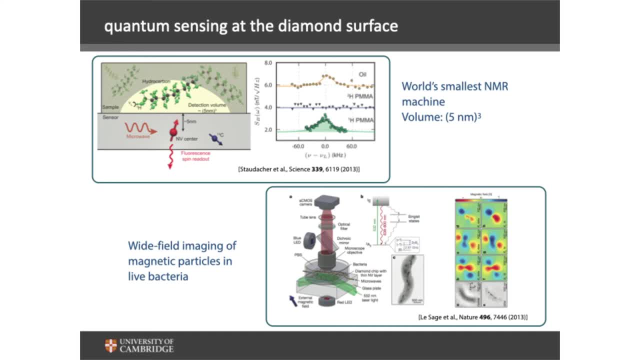 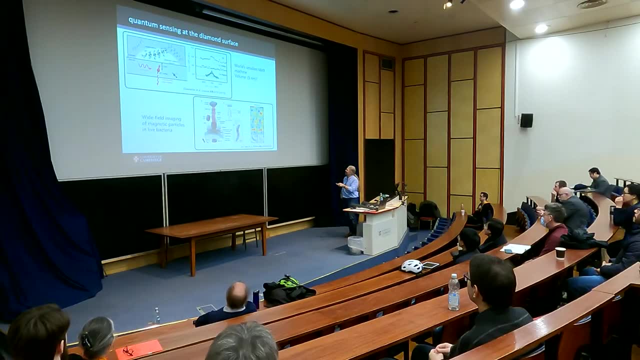 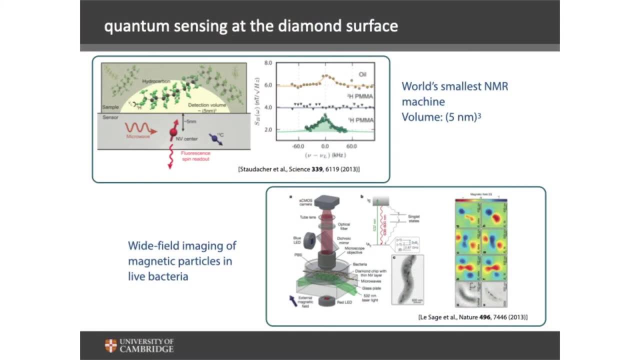 but they don't get rid of it. So they have iron in their bodies, And then these iron deposits align with the first magnetic field. So it's a funny system on its own, And they're able to measure. The only way to see it, of course, is to do scanning, electron microscopy, like they've done. 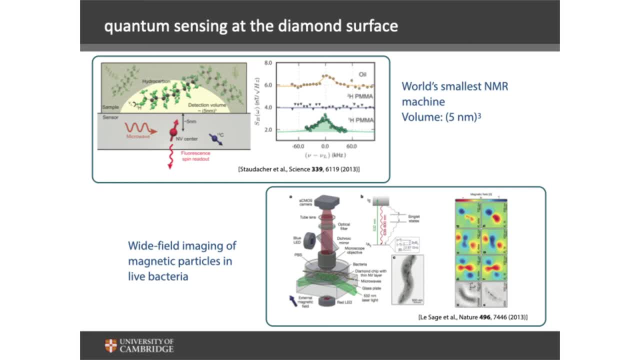 here. But you kill the species, of course, when you put it into an electron microscope. By doing it like this, with a diamond film right here, this is our effectively diamond film, with the shallow implant But high density, you can actually map out the orientation of these iron. 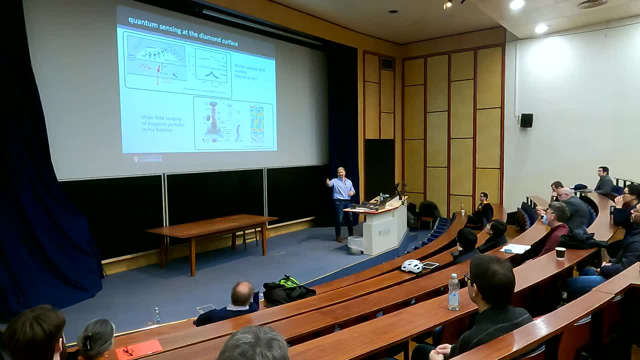 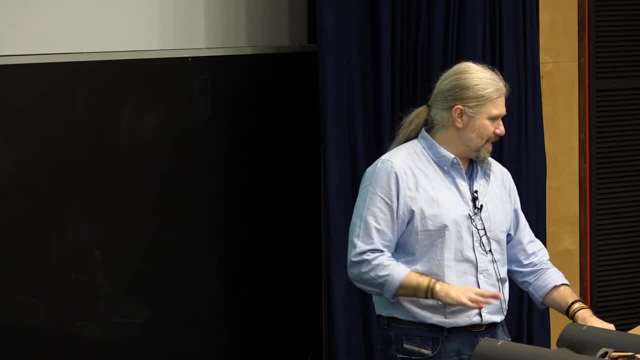 deposits inside these lines as the thing wobbles on in your sample Anyway. so I think I justified. diamond is good and it will be around for many different applications. I want to finish off last few minutes. I want to finish off with something that has nothing to do with diamond. 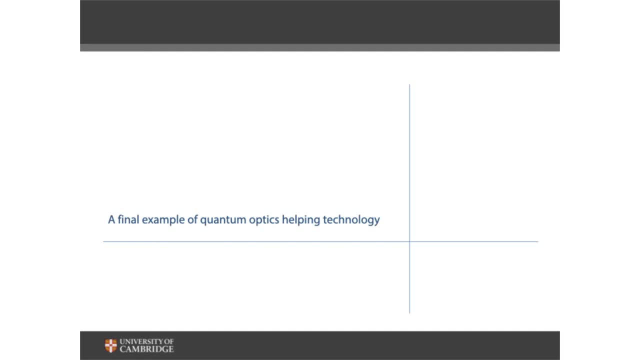 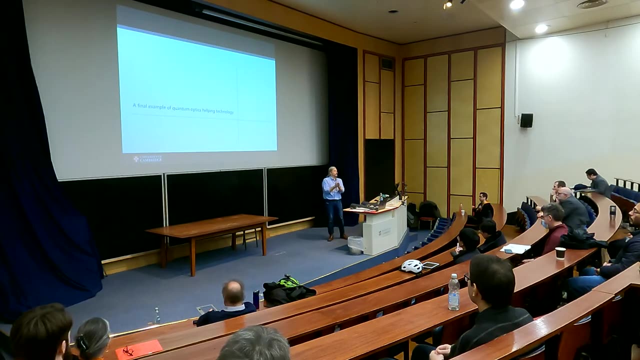 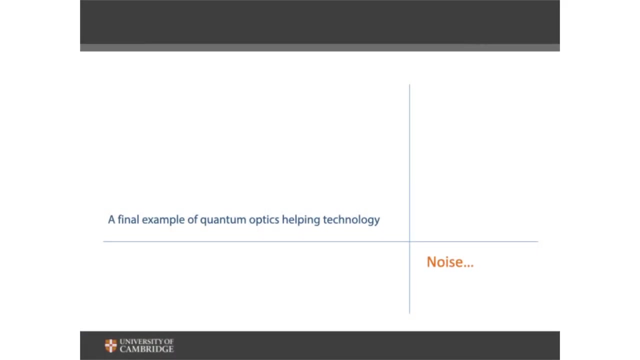 but really taking back, taking us back to the main message. The main message was quantum optics, And I want to highlight one very odd feature of quantum optics and how it has also impacted our technology, And that is noise. Everything I talked about was signal, improving signal, isolating signal, And 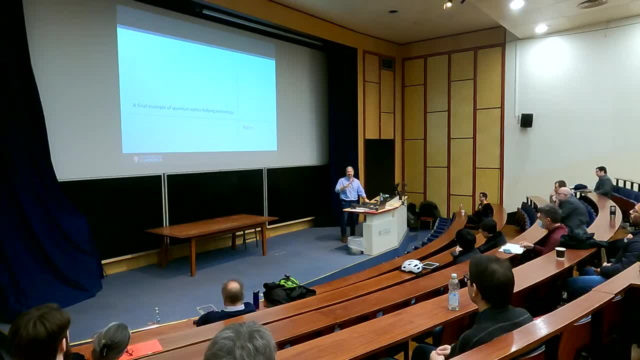 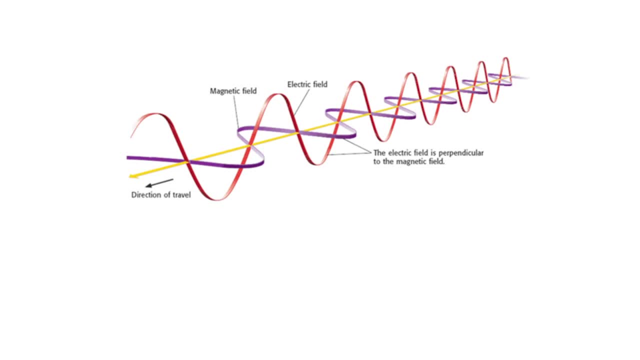 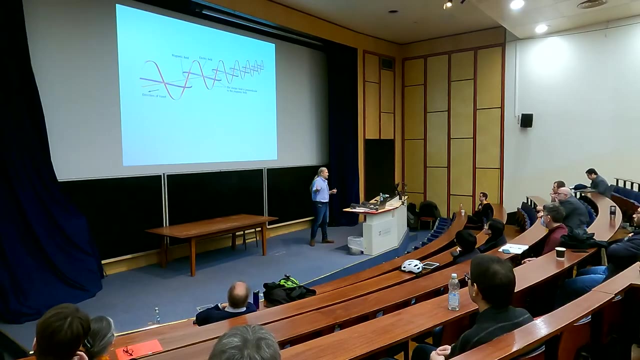 now for the final punchline. we're going to talk about noise. So if I talk about light, we can talk about the quantumness of light. We always talk about the wave and particle nature. It's always the or can be. you know the thought I want to stress. you know the debate has been going on for 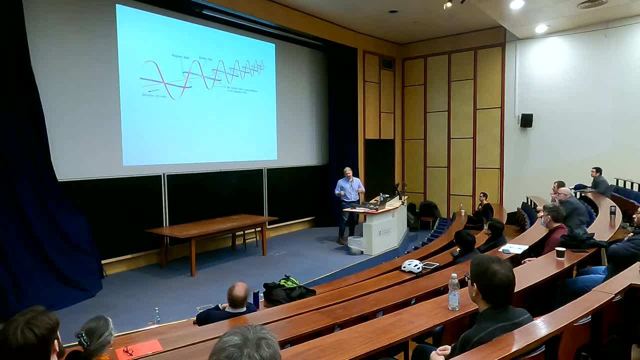 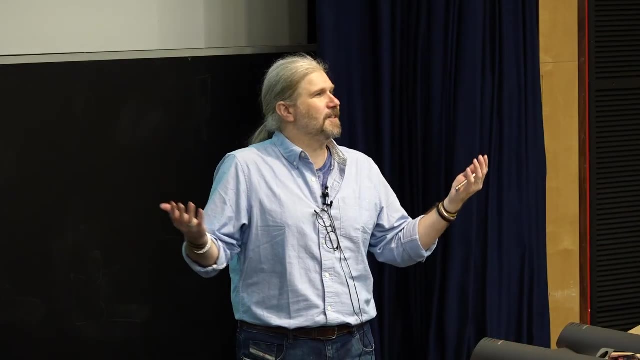 decades, centuries, You know you had Hohen's beautiful experiments and ingenious idea of Hohen, wavelets and Young's experiments. for now Prano for everyone, experimental, demonstrating that light is wave, And then you have Newton claiming that light is corpuscular. for no good. 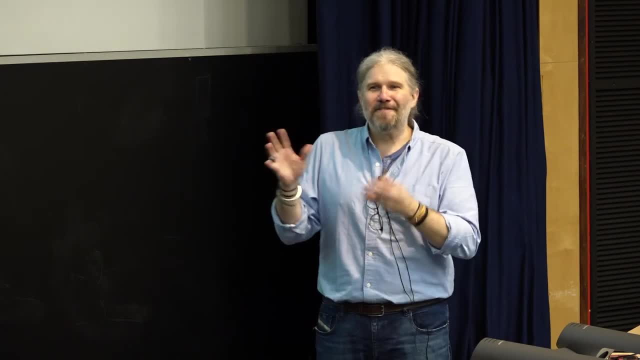 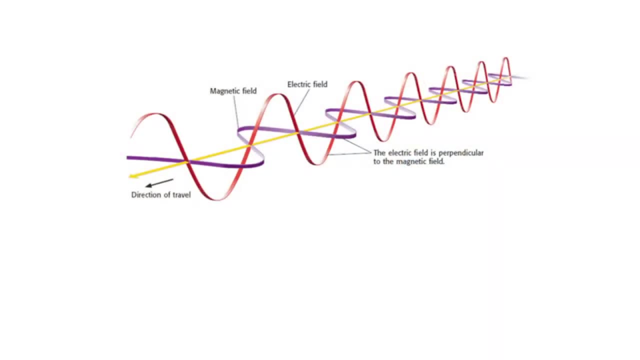 reason, because it's simply authority. But aside from that, you know, we now know that light is made of particles, photons, if you treat it that way. but the interesting thing is, there is more to the story of the quantumness of light than just whether it's wave or particle. it's this part, it's what happens to. 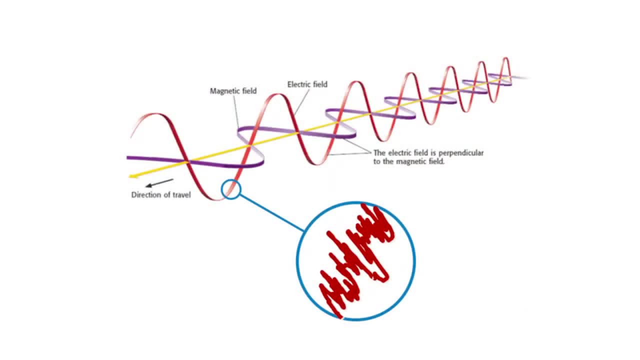 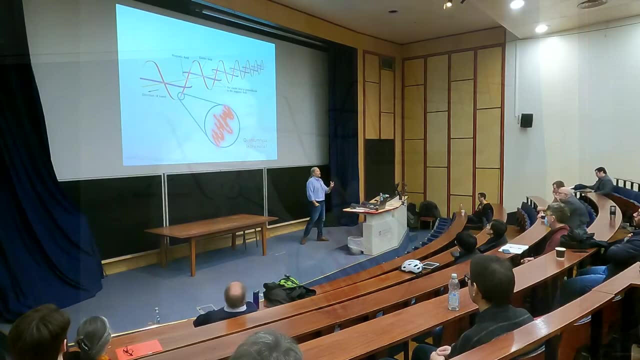 if you, if you zoom in and look the noise on it, that's where quantumness is. so it is. there's more quantumness buried in the fact that there is noise that you can't get rid of. it's not the classical noise, there's quantum noise, and that's interesting one. and so, and what happened was, 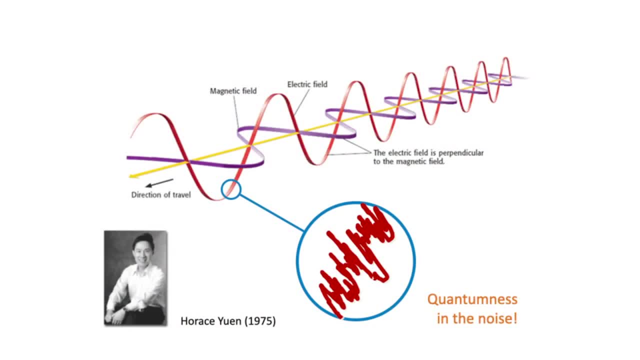 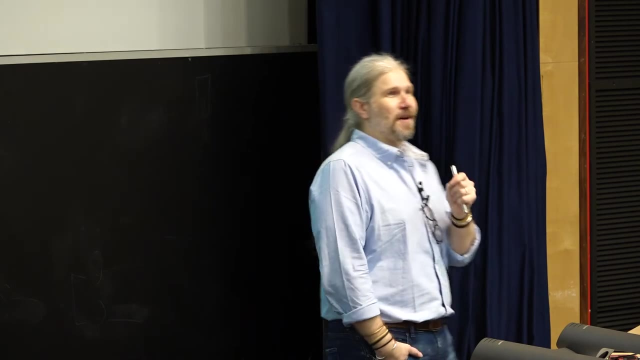 in 1975, Horace Ewan came up with the idea that the fundamental limit of noise in any object, in any physical systems, probably vacuum, vacuum noise. and he came up with the idea that if you use light and non-linear optics you can take the absolute limit of noise and squeeze it. you can make it. 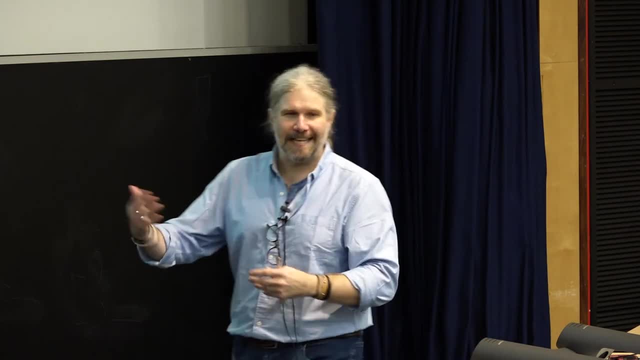 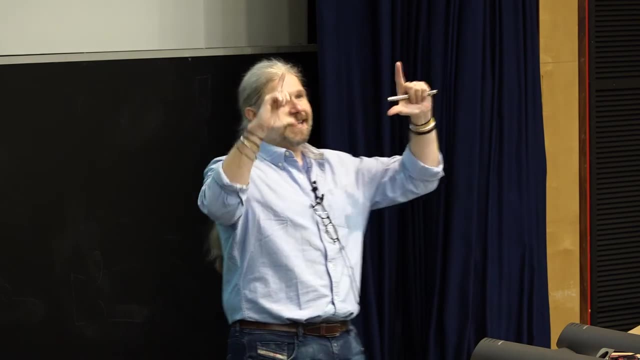 less. it comes at the expense of something, of course. it comes at the expense of noise being larger somewhere else. so it really is. you can make it less. it comes at the expense of something. of course. it comes at the expense of the concept of squeeze. that's the word. the technical word is squeezing. so you take the. 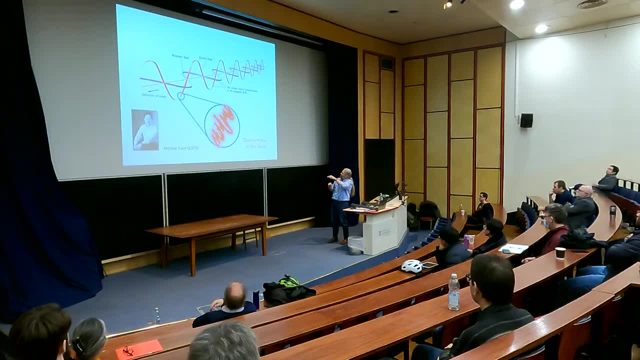 uncertainty. and you, you take this, that whatever this, this segment is, that's how uncertain you will be set by quantum physics, set by vacuum fluctuations. and he says, if you employ non-linear process in in materials, you can actually take this and make it much smaller and maybe noise. 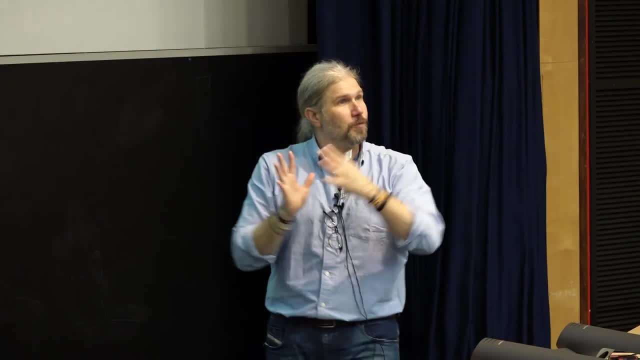 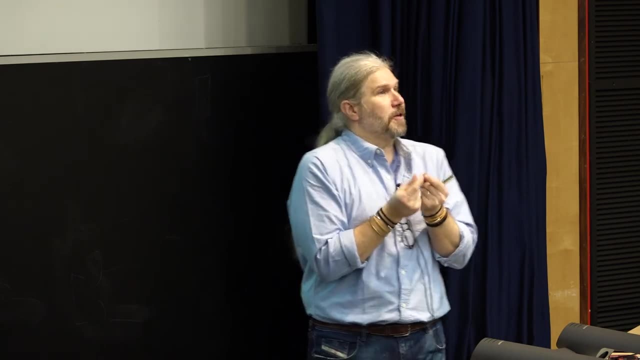 fluctuations in and out of plane will be much larger. fine, but you, you, the volume is preserved. think of it that way. there's no breaking of fundamental laws here. but you can choose an axis where there is no noise or there's very little noise, and that's called squeeze light, and 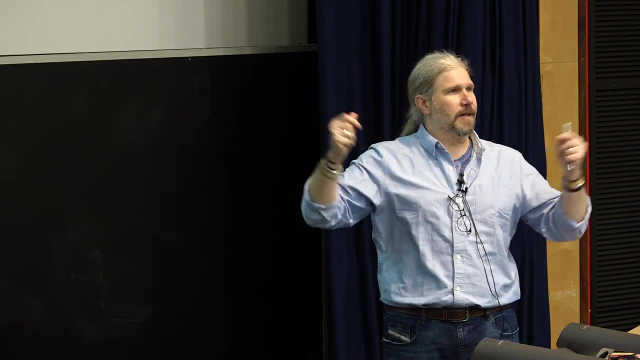 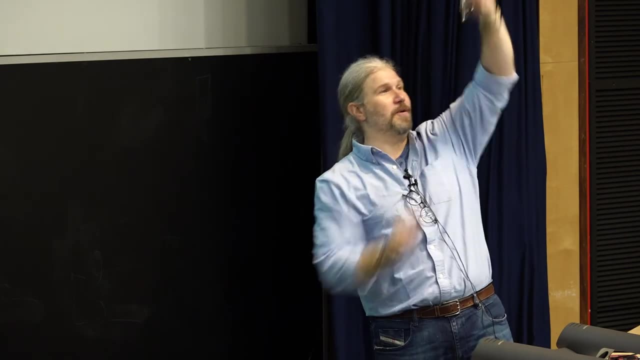 people have demonstrated this. and now it's that that squeezing is such a way that it's like a thin line. think of it that way: just start from a circle of noise, and now it's squeezed to the point where it's not even an ellipse, it's a that extend a complete line. but the catch here, the nice thing, 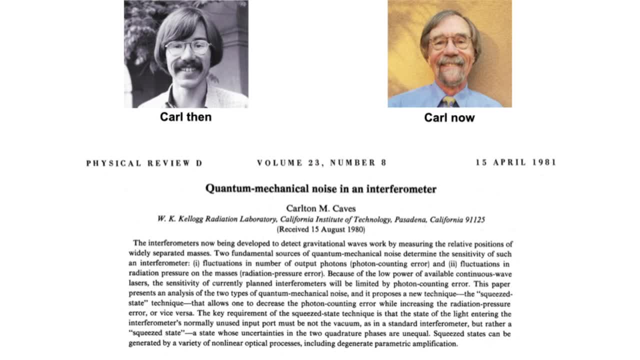 is 1980. in 1980, Carlson caves- Carl caves- came up with an idea, and this is Carl. then, when he came out with the idea, and this is Carl today, great guy, fantastic guy, Carl. then, when he came out with the idea, and this is Carl today: great guy, fantastic guy. 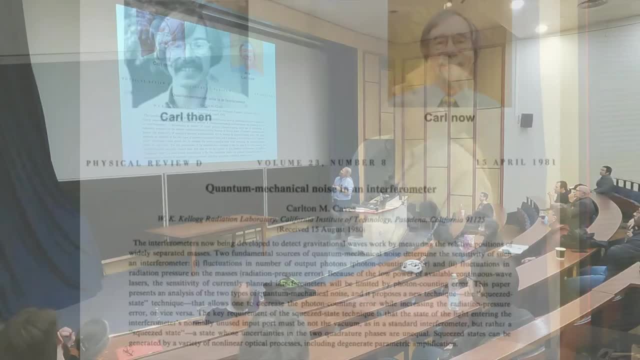 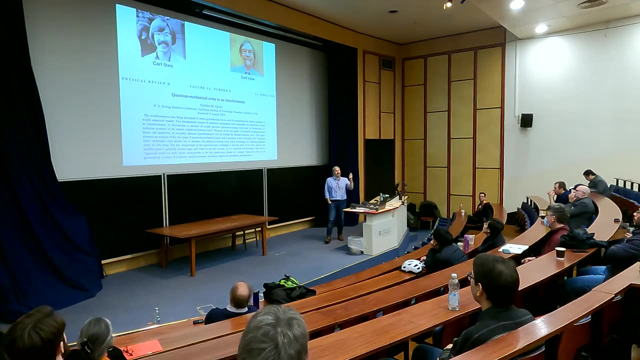 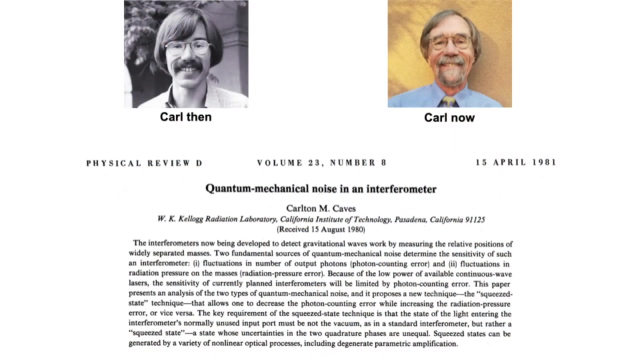 and it came up with the idea that if you could get rid of the quantum mechanical noise in an interferometer, you can do more sense of sensitive detection. you can do more sensitive detection of things, whatever that is, and this relies on the concept of squeezing, interestingly, a horse. you. 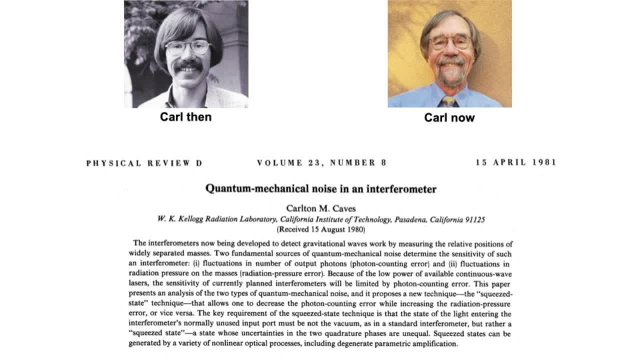 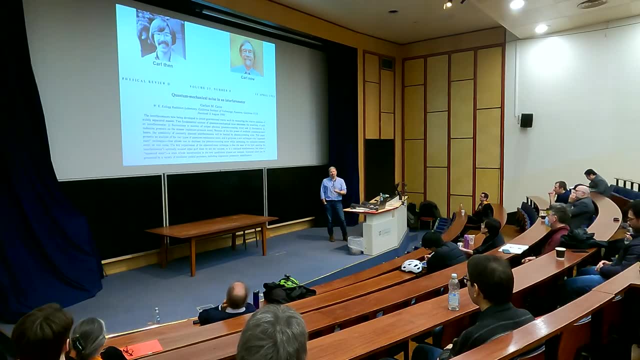 and did not come up with the word squeezing. it came out with the word coherent, two photon states, more technical, and then Carl said let's just call it squeezed, because we're that's what we're doing it, and said that the uncertainties in the two quadrature phases are unequal. that's the point. 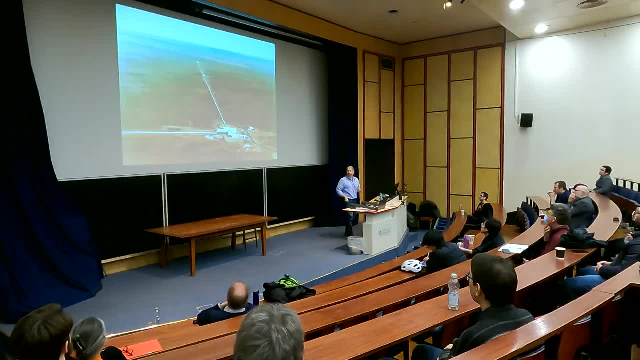 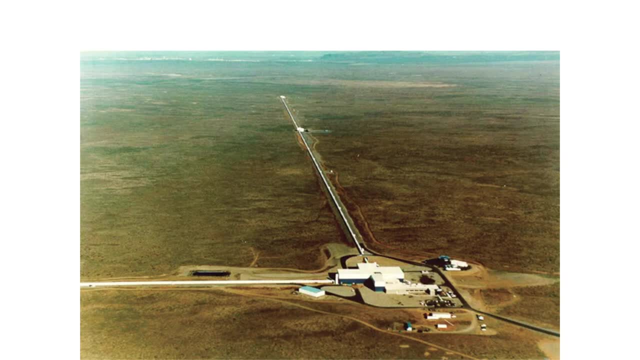 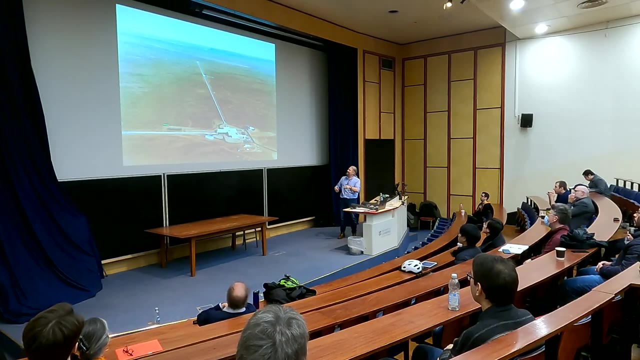 right and where could this be useful? it could be useful in LIGO. what is the biggest interferometer we have today? LIGO. what is the interferometer that's trying to measure the weakest possible signal? LIGO. classically, you can make your interferometer as stable and as good as possible. 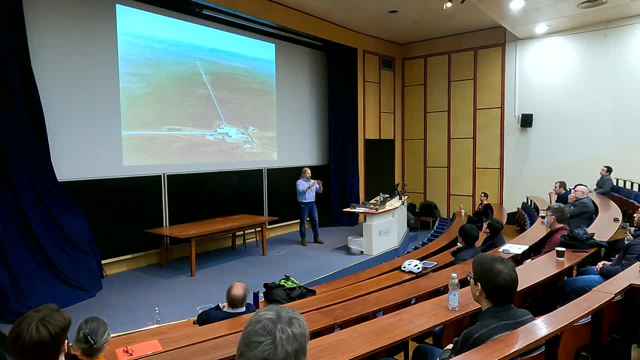 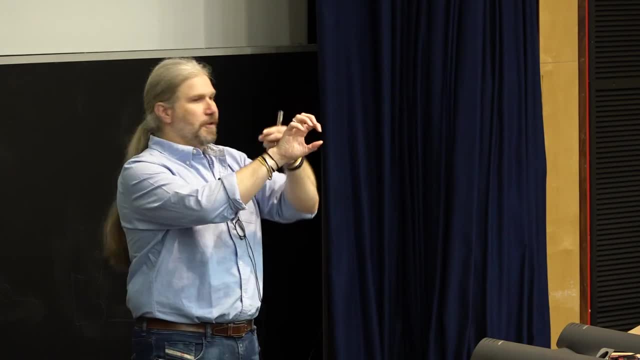 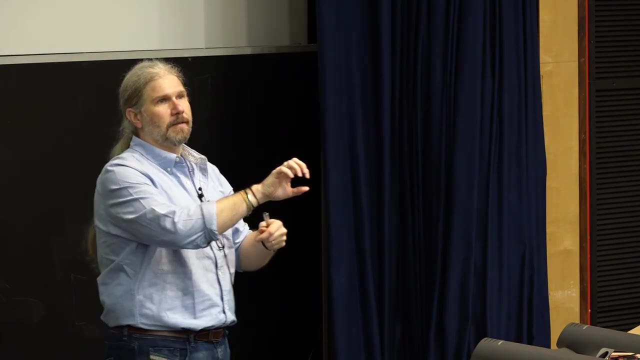 but there is one catch: no matter what you do, you will have a beam splitter, but in the interferometer light comes in and splits at a beam splitter and then combines again right at that beam splitter. there's two outputs, but there's also two inputs. light goes in one of them, vacuum goes in the other. classically it means nothing goes. 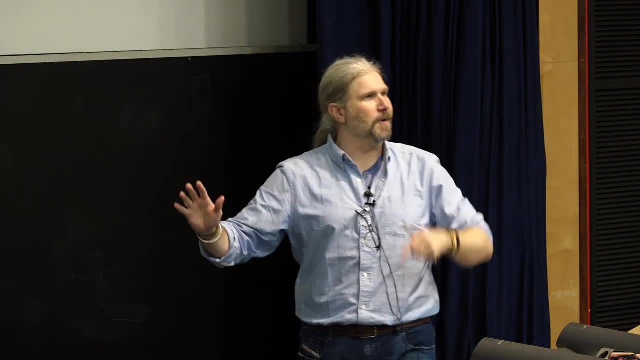 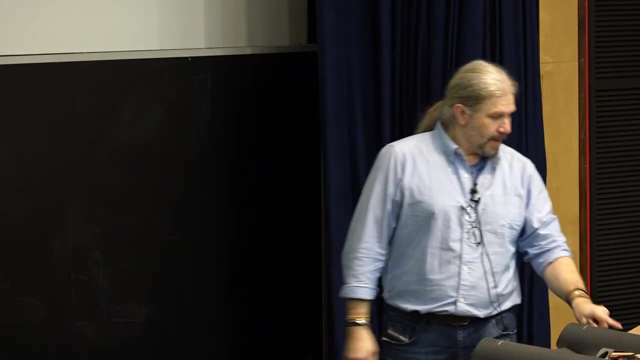 in the other. quantum mechanically it means full vacuum noise goes in the other. one uncontrolled vacuum noise feeds into your interferometer. that's your fundamental limit of sensitivity. so this is what Carl caves was saying: if we actually feed in instead of one beam splitting into two, 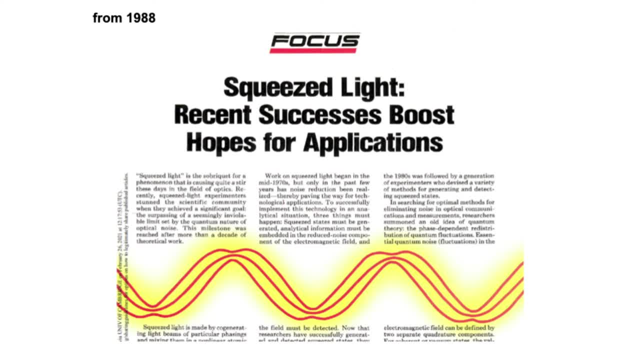 why don't we start with two beams? one, the beam you want that's going to carry your signal, your detection beam. two: squeezed vacuum. let's make sure that we take the vacuum and squeeze it in the axis we care about, so it doesn't affect, uh, the experiments. and this is a an article from 1988. squeeze light. recent success boost hopes for applications and one of the applications that was a boost that was hoped was gravity wave detectors approach. the level of sensitivity needed for calibration likely will have become routine and presumably employed in the efforts for LIGO 1988. this is paper from 2019.. I wanted to highlight the author's list on on how complicated these 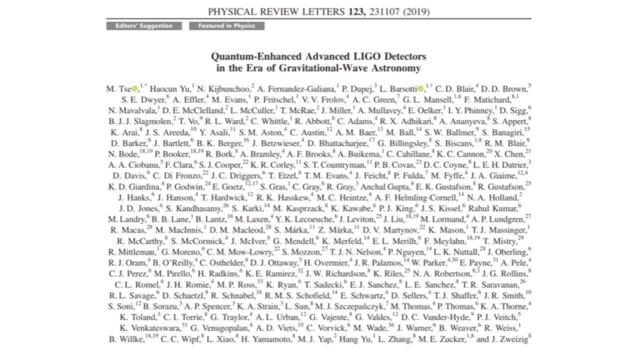 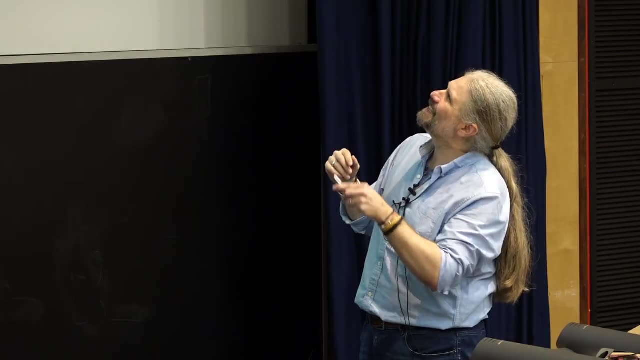 experiments can be and, interestingly, you might think that this, at this point, like in particle physics papers, you might think that it's alphabetical. it's not. if you, if you're careful, there is credit given in some random order to uh, to a certain number of people, and then at some point it becomes alphabetical. so so, so clearly, these people did the. 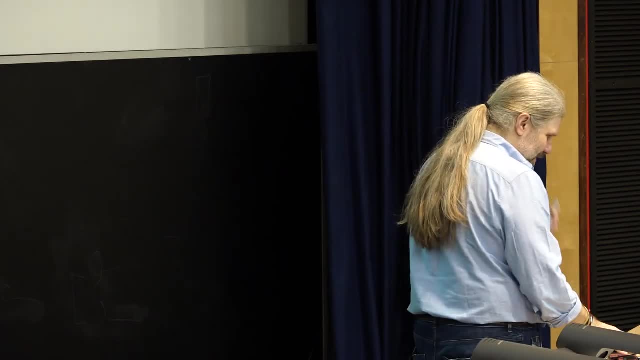 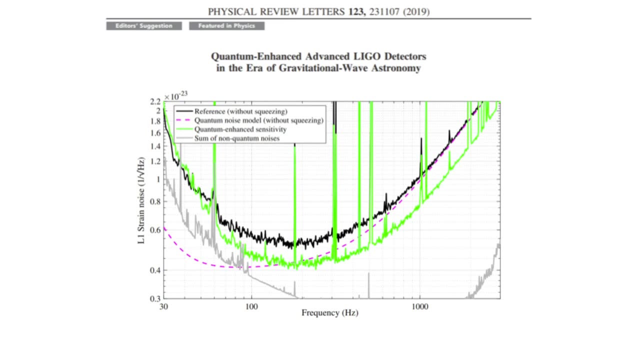 work. uh, I think those are the main ones that actually struggled with the, with the whole experiment. what they've shown is is that reference- this is the best LIGO can ever do- is this black line of noise versus frequency, so it's like a noise spectrum, if you will. how good your system. 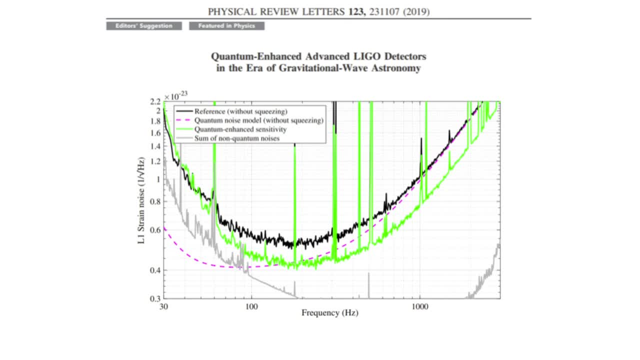 is. so this is what that profile is. all right. so you cannot. if your signal happens to be, if your, if your gravitational wave is at 100 Hertz and it happens to be at this level, you wouldn't be able to detect it. that's what it says. that's the, the lowest, the threshold for. 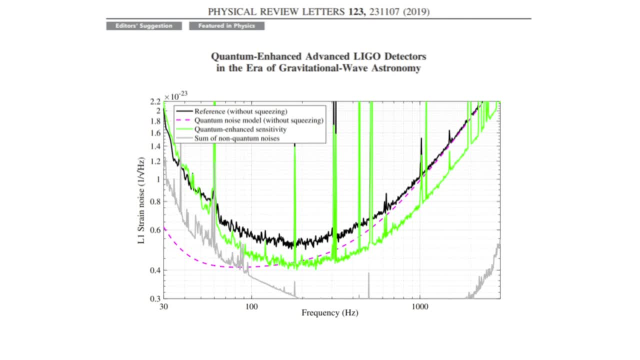 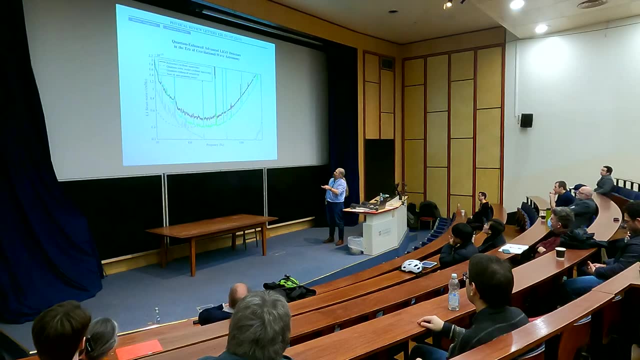 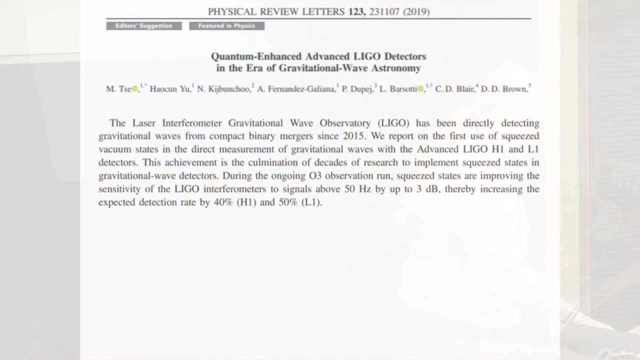 detection. and when they put quantum enhanced sensitivity by putting in squeeze vacuum from one side and a normal laser from the other, they're able to drop it down. remember this is logarithmic, so they're able to drop it down and they use that to actually detect, uh, detect gravitational gravitational waves. so squeeze light based gravitational wave detection. 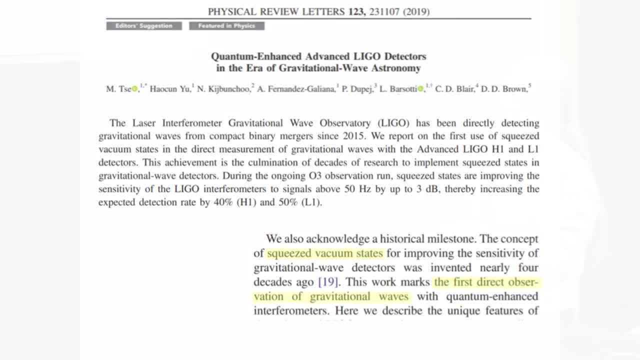 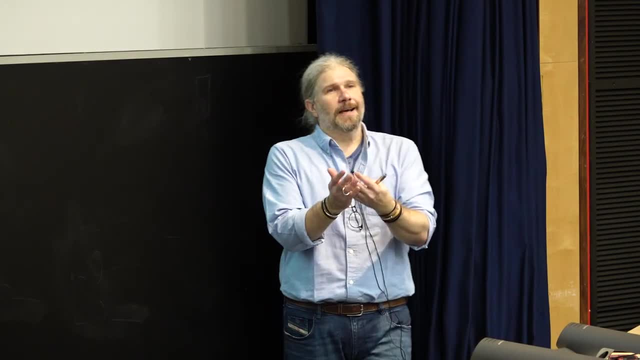 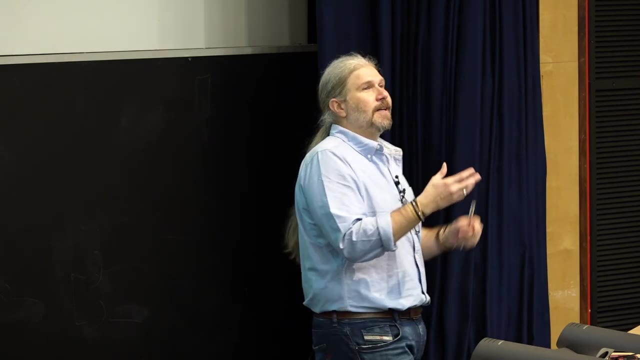 has happened. it's the first direct observation of gravitational waves using squeeze vacuum states, essentially by essentially using a nonlinear Optus Crystal to generate squeeze light. and what is squeeze light? what do we? when I see squeeze light, what do I mean by, especially squeeze vacuum? it turns out squeeze vacuum is photon pairs instead of vacuum, instead of zero, nothing. it.